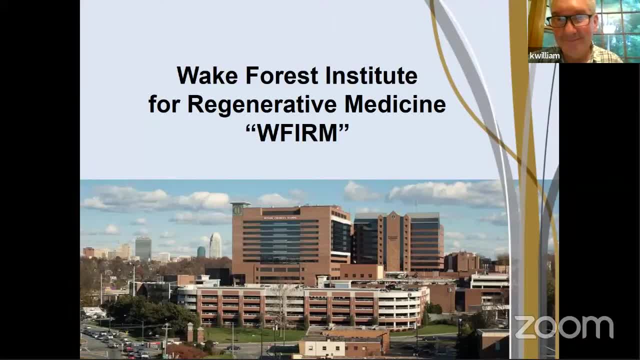 It gives me pleasure in welcoming all of you to guest lecture by Prof Kudi Wilms from Institute for Regenerative Medicine, Wake Forest School of Medicine, North Carolina, United States of America, On behalf of Department of Chemistry, Faculty of Mathematics and Natural Sciences, IPB University. 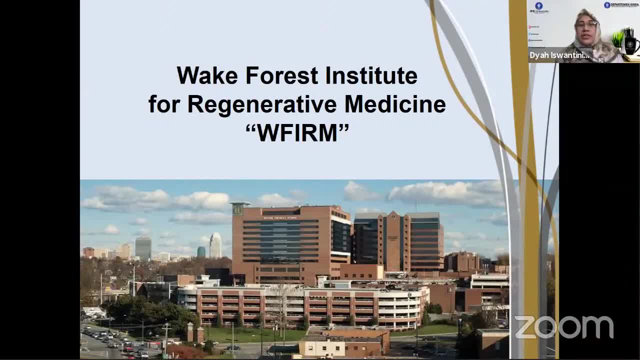 I would like to welcome Prof Kudi Wilms to our university, especially to our department, even by virtual meeting, We are glad to see you. I would like to express my gratitude for your time and giving lecture today, As your title of lecture, Tissue by Engineering, is very interesting. 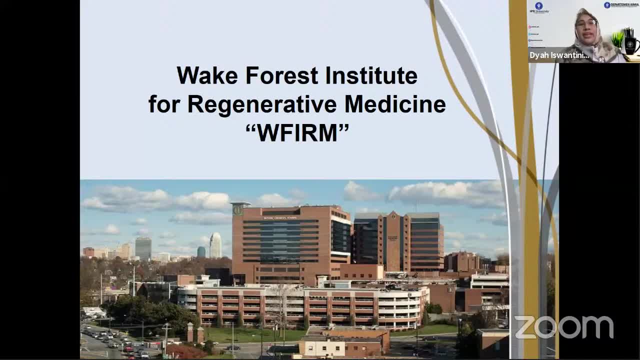 I believe everyone here- me, my colleagues and also my students- would have an engaging and enriching session ahead. Thank you very much, Prof Kudi Wilms. I hope Prof Kudi will continue having guest lecture for the following time. 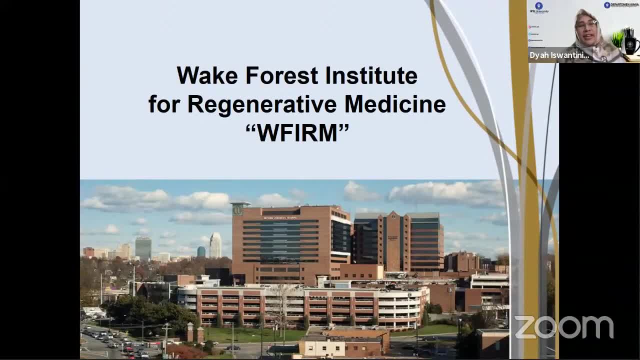 I even pray when the pandemic ends and everything runs normally. Prof Kudi Wilms will personally visit our department And I hope everyone can contribute to guest lecture firsthand in person. Also, I would like to thank Dr Irma Sparto as moderator and for arranging this general lecture. 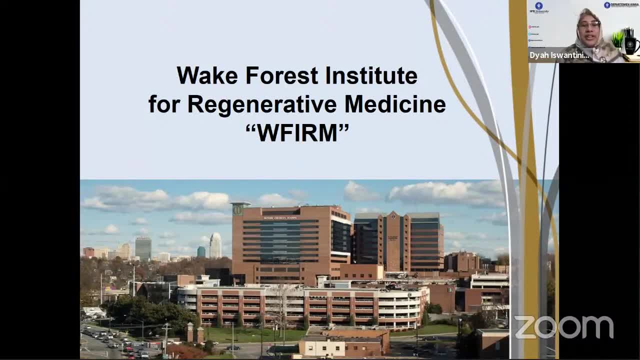 Okay, without further ado, let's join this guest lecture together. Thank you very much. Wassalamualaikum, warahmatullahi wabarakatuh Waalaikumsalam. Thank you, Prof Dia. So, with this welcoming speech, 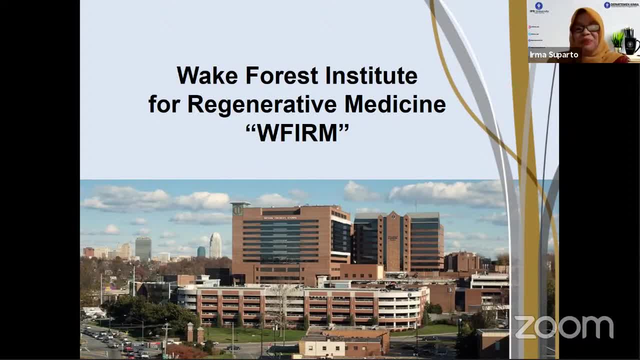 that means we will be able to start the lecture, But you know we always love to take pictures. Usually, Kudi Wilms is the photographer when he comes to Indonesia. Oh, Pictures, Yeah, But today we will take just picture in front of this Zoom. 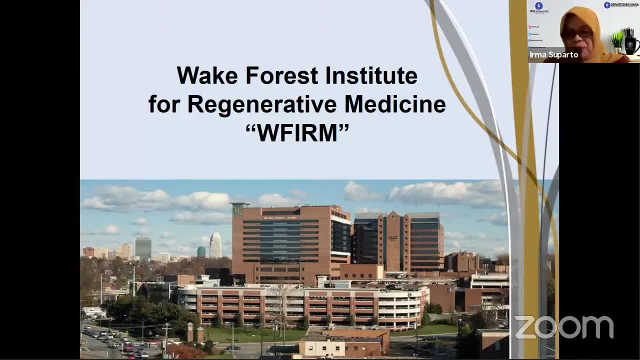 So we have only a couple of panels. So please, Ibu Santi, you can start taking pictures, maybe? Yes, Thank you, Ibu Irma. Everybody open? Yes, Yes, On camera. Maybe it's better if the slide should be removed first. 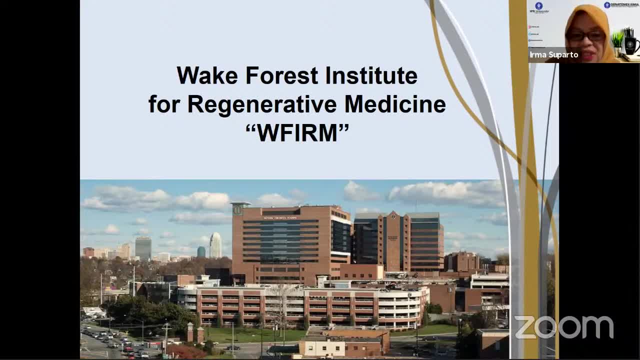 Prof Kudi, I will stop share screen. Can you stop share screen? Will you be able to start again? Un siap-siap, ya. Un. Okay, We want to. Okay, We just make it small. How about it? 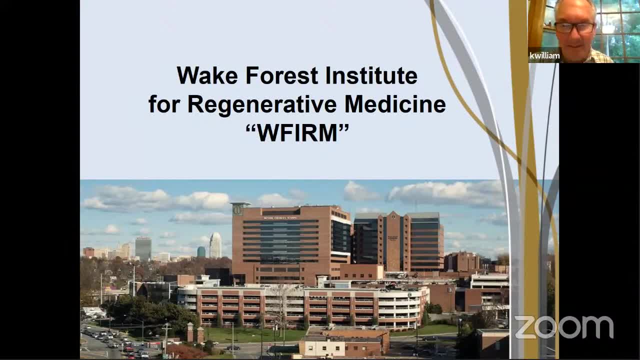 Okay, Wait a minute. You want me to do what here? Stop share screen. Is it possible, Kudi? Okay, Don't worry, Don't worry, Don't do it. Okay, Mungkin ambil aja, ya, Okay. 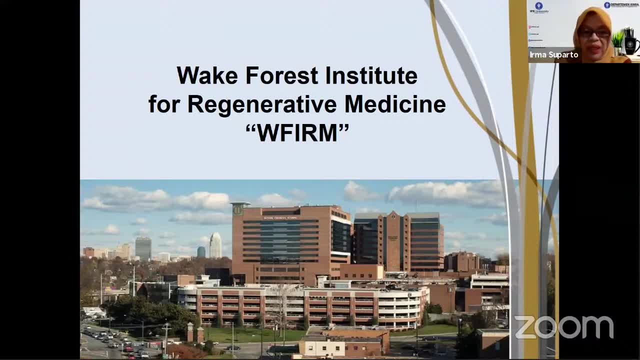 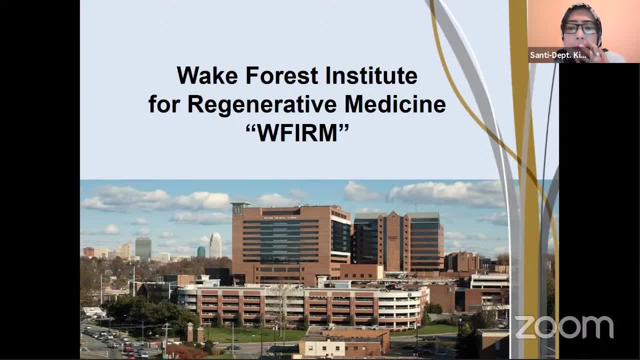 Good job, He's really good. All right, We're going to hang up. You slow down. Sorry, I couldn't tape it. We talk. Yes, Okay, I don't know. I'll tell you what you got: Boon set. you got a link. 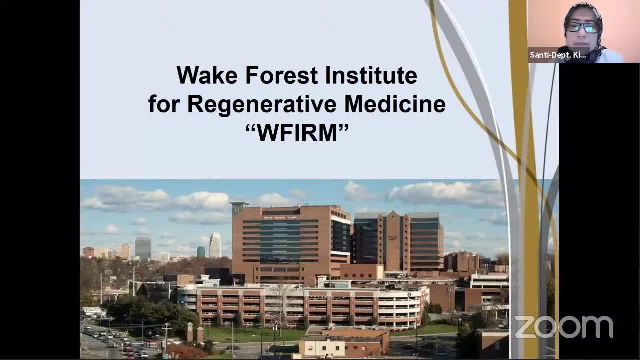 Yes, I do. I'm sorry, Just still write if you want I need to. What video is this? Okay, Boon, it's a format. No, just so you know It's الرBayah. Do the above again, no matter what. 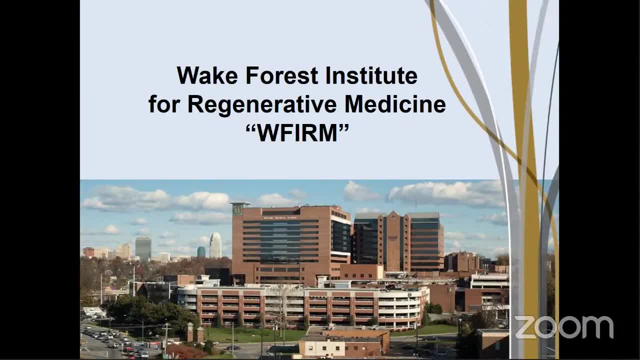 We created a different format. This is William's first video, right? Yes, Yes, This is William's first video, as you can see, by a computer. Okay, Okay, Are you done? Yu, Okay, Are you done? 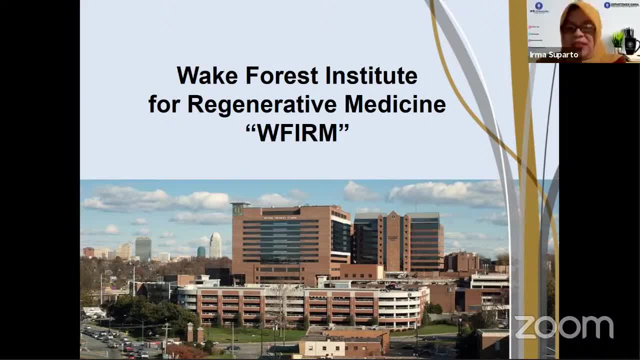 Take a photo of the first slide, One, two, three Second slide. Okay, I would like to welcome also to Ibu Yesi. Ibu Yesi is from the physical department. Yes, Good morning Ibu Irma and Ibu Diah Ispantini, and also Professor Billian. 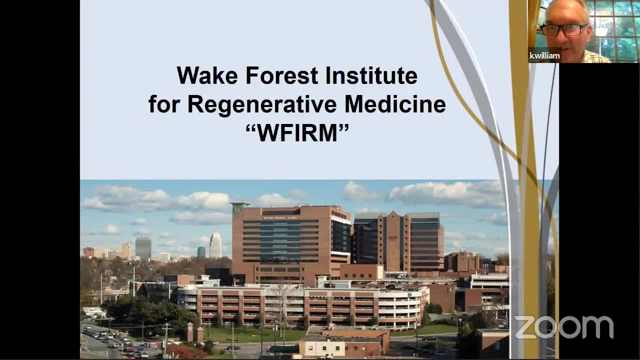 Nice to meet you. Nice to meet you. And thank you for the invitation and the opportunity. Dr Yesi, a very productive researcher, also in working together with biomaterials. Okay, all done, Yuni. Okay, thank you everybody. Now it is such a exciting- we are going to listen to Prof. 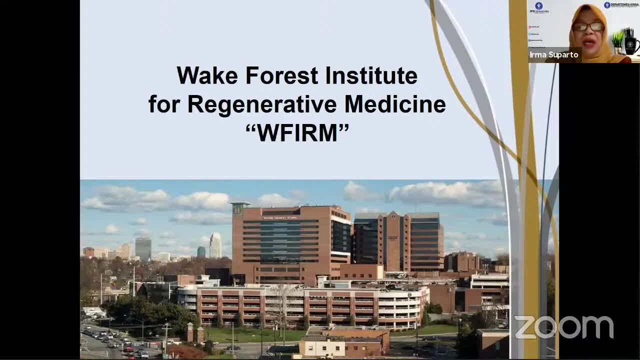 Cody Williams give a talk, but I would like to give a quick CV. He is. he graduated in this- I'm well, I have to say it- in 76 from Iowa State University and become a veterinarian in the 1983.. 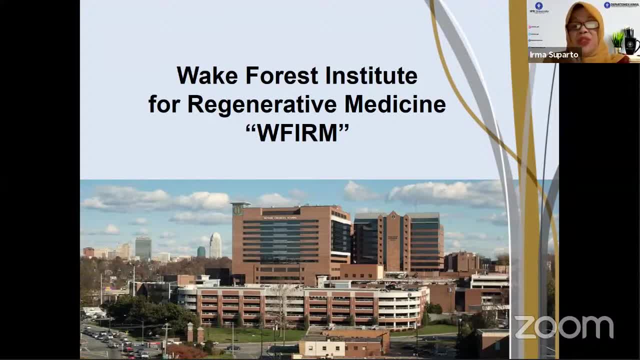 And he works many, many places and most of all in Wake Forest University, North Carolina, as a professor in regenerative medicine, comparative medicine, in pathology, in surgical sciences and also translational science institute. Many chapters, many, many book chapters and articles, and he has so many Indonesian students as his. 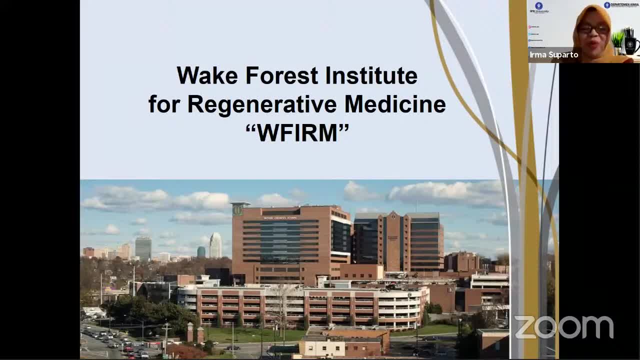 PhD students, including me, including me. Prof Cody was also my advisor, So it's a great pleasure to be here with him, So we're going to listen to his talk now. So if there are any questions that you have for Prof Coleman, and then we'll respond to the question. 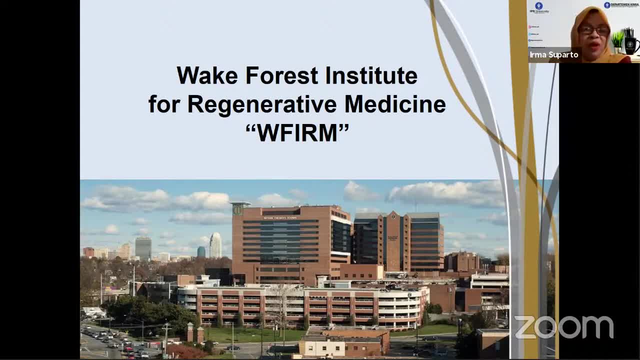 It's a very great honor. Please, Professor Cody, you can start the lecture and share your perspective. Thank you so much. Thank you, Irma, Great to see you again. Yes, So I've come to Indonesia now about 21 times. 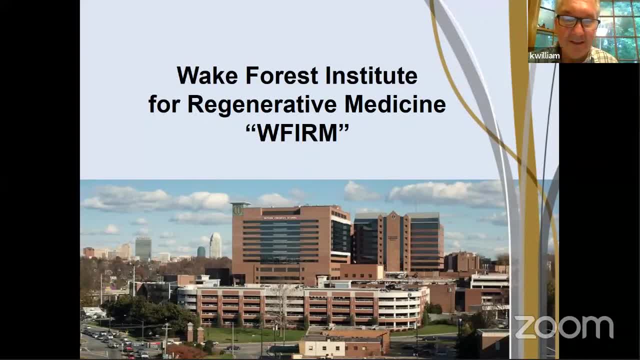 I come about either every year or every other year to Indonesia. I'm very sad I can't be there now, but hopefully things will clear up and I can be there within the next year. Irma has invited me to give many, many talks. 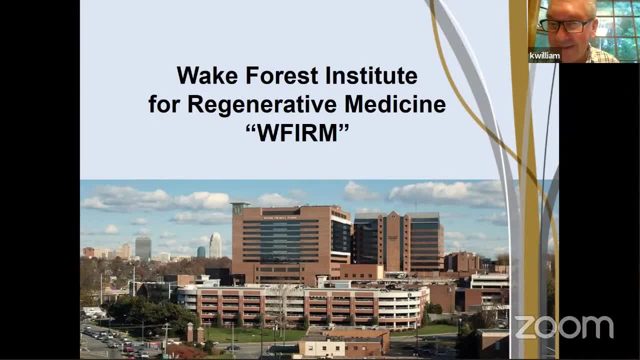 mostly dealing with primatology, physiology, pathology, and that's basically what I am. She finally found something that I had to ask for slides for this. I probably shouldn't be telling you all this, but I got a C in chemistry when I was in school. 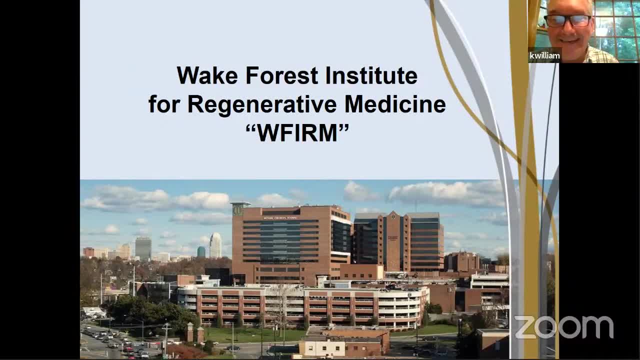 I did a little bit better in physics, But I got a C in chemistry, So hopefully I won't come across too naive, but I'll go ahead and get started. Greetings from Wake Forest University. I work at the Institute for Regenerative Medicine. 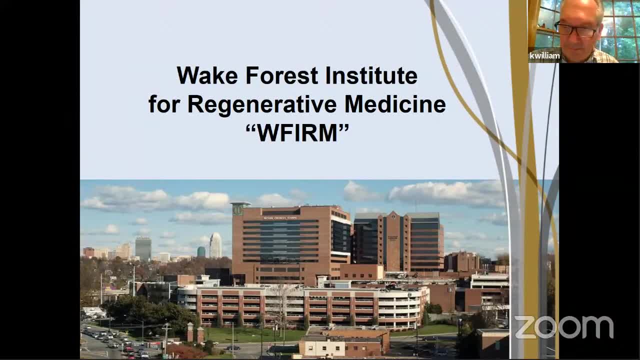 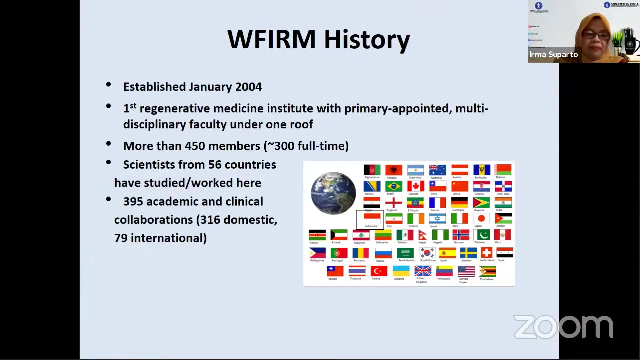 or as we call it, WFARM. Hello, Hello, And it's not changing my. You hit the slide and then you press enter or forward. Well, that's what I'm going to. There we go, So WFARM history. 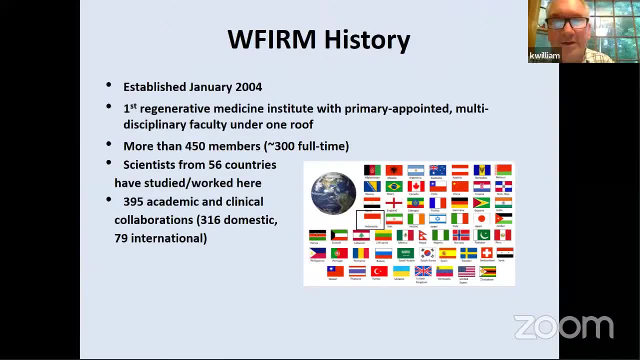 We were established in 2004.. We were the first regenerative medicine institute with primary appointed multidisciplinary faculty under one roof. We have more than 450 members, scientists from 56 countries and engineers from the United States and engineers from the United States. 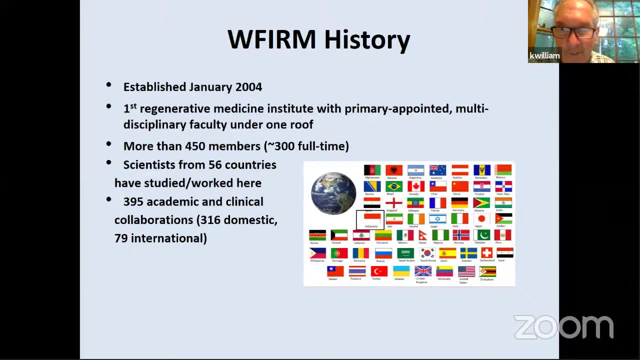 and engineers from the United States and if you'll notice down there right below the world, a little bit to the right, with a box around it, is the Indonesian flag. from our collaborations with Indonesia, We have 395 academic and clinical collaborations, 79 international. 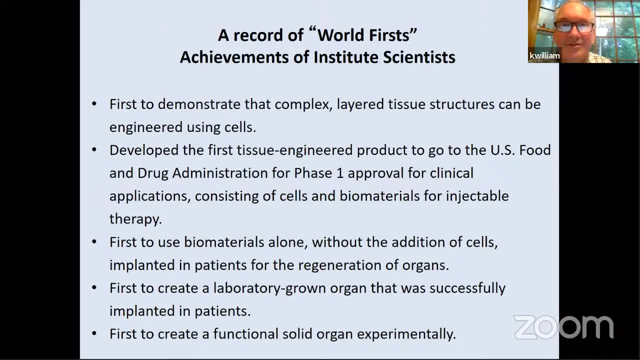 We were the first to demonstrate that complex layered tissue structures can- I'm going to move my, there we go- can be engineered using cells Developed, the first tissue engineered product to go to the US Food Drug Administration for a phase one approval for clinical applications. 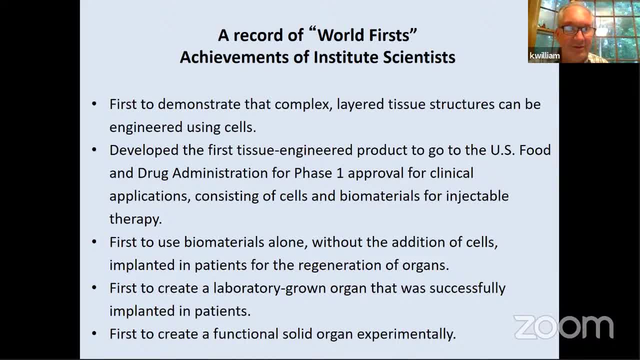 consisting of cells and biomaterials for injectable therapy. First, to use biomaterials alone, with and without the addition of cells, I still don't like where that is. There we go: A first to create a laboratory-grown organ that was successfully implanted in patients, and first 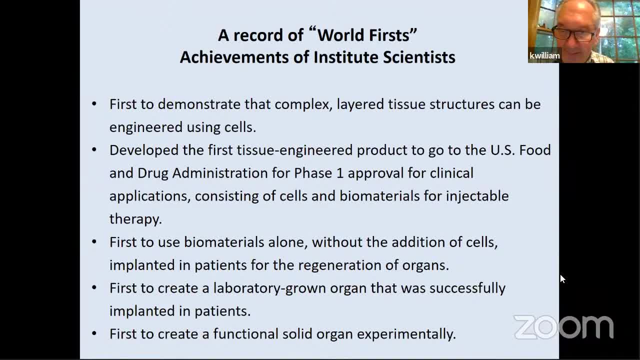 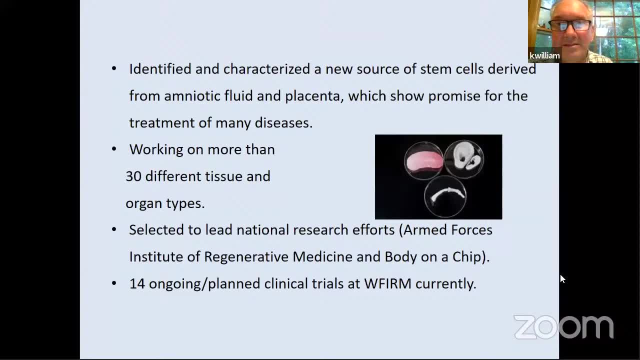 to create functional, solid organ. experimentally Identified and characterized- a new source of stem cells derived from amniotic fluid in the placenta, which show promise for treatment of many diseases, Working on more than 30 different kinds of tissues and organ types. Selected to lead the nation. 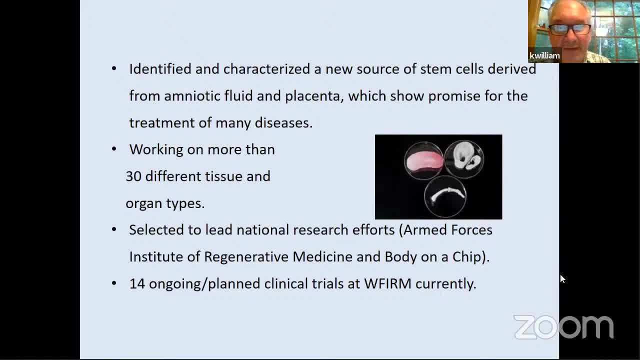 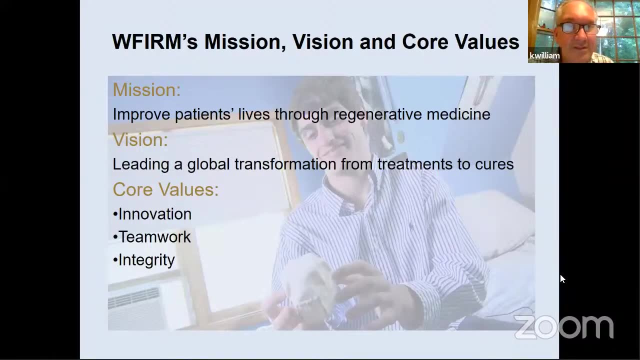 research efforts: the Armed Forces Institute for Regenerative Medicine and Body on a Chip, 14 ongoing planned clinical trials at WFIRM. currently, Our mission is to improve patients' lives through regenerative medicine. The vision is to be a leader in the global transformation from treatments to cures. A very 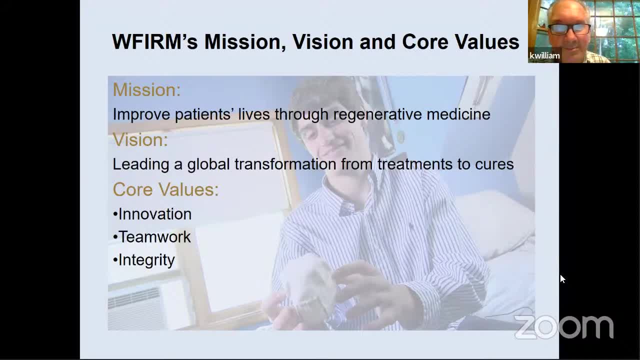 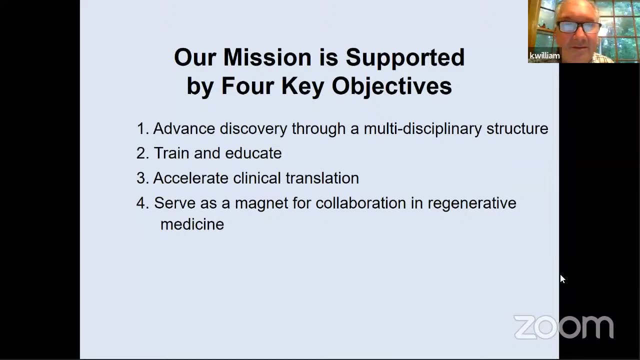 big emphasis of ours to get this into people as safely and as quickly as we can. Our core values are health, safety and integrity. Our mission is supported by four key objectives: to advance discovery through multidisciplinary structure, train and educate, which we all do. accelerate. 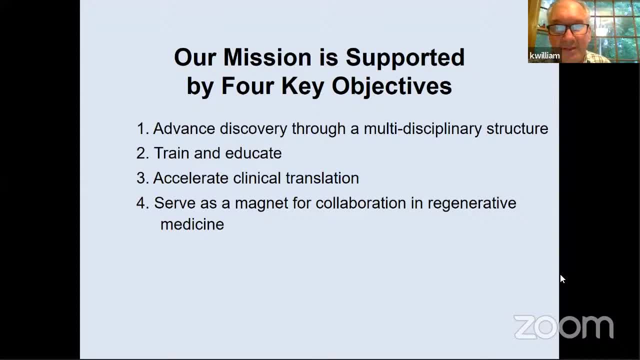 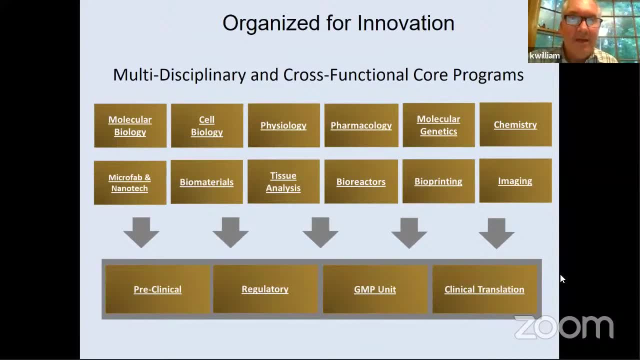 clinical translation and to serve as a magnet for collaborations in regenerative medicine, which I just said we do, and including with Indonesia. We have within our institute, multidisciplinary and cross-functional core programs And regenerative medicine is a combination of basic, really a combination of basic. 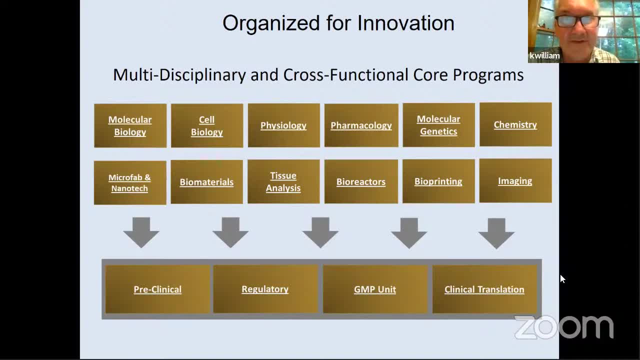 sciences: molecular biology, cell biology, physiology, pharmacology, chemistry, nanotech, biomaterials, tissue analysis, bioreactors, bioprinting and imaging. We can take our findings that we have in the lab and the best way to do it, and we can take them to the 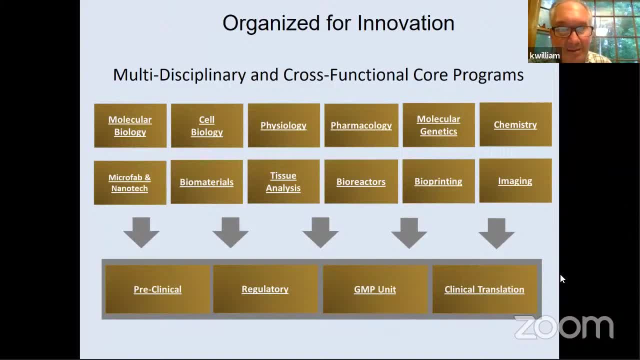 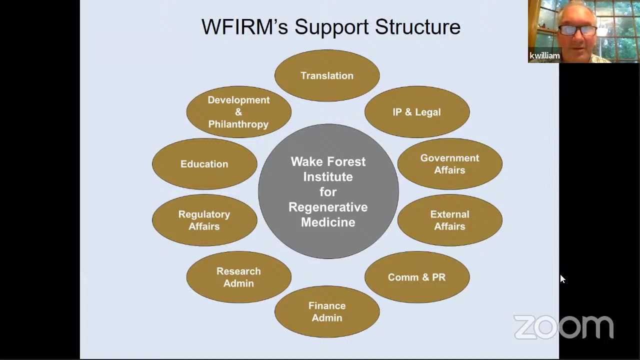 benchtop, through preclinical studies, then regulatory studies, then using a good manufacturing practice unit and then into clinical translation. We have many different facets of what we do. Important is translation. We have IP and legal people that work with us, government affairs people that know how to work with the FDA, external affairs people. 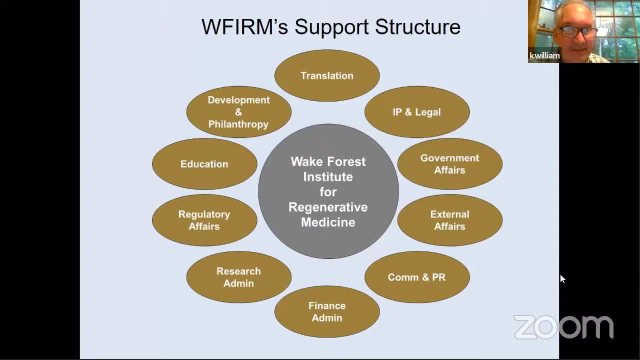 PR, Finance administration, research administration, regulatory affairs and education- all within four different levels in one building. four floors on one building. all of this which makes it very, very nice for collaboration: easy to go, talk to somebody, easy to get things. 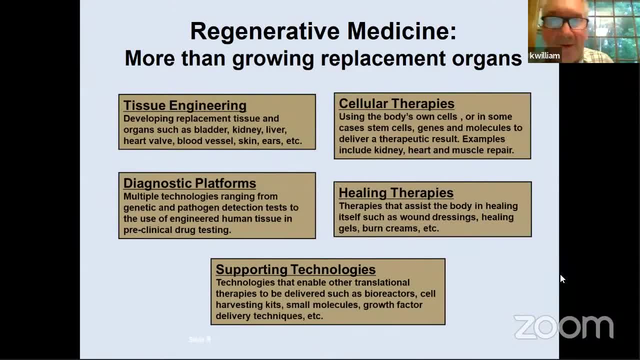 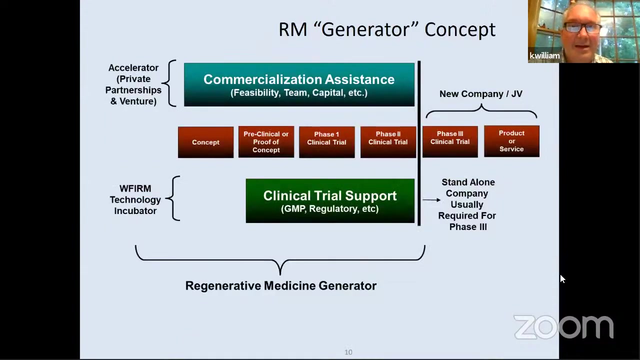 done. So what do we do? Regenerative medicine is more than growing replacement organs. It isn't about pozwis, proper medicine or rulebook therapy or some kind of general fellowship. we are focusing on proactive blood living and wills tissue engineering. 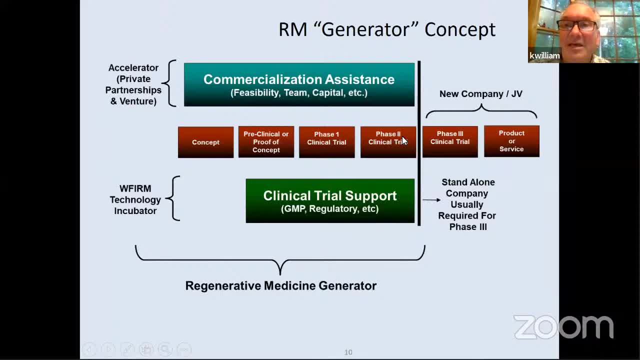 cellular therapies, diagnostic platforms, healing therapies and supporting technologies. My emphasis is really using small molecules and growth factor delivery into tissues that need regeneration to try to stimulate in situ regeneraiona it all the way up to phase two clinical trials. Then we will go start a new company and take it. 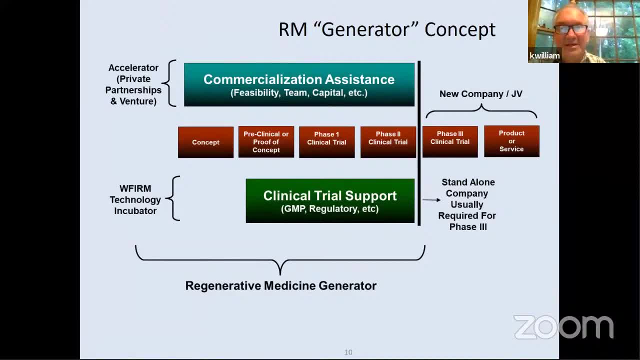 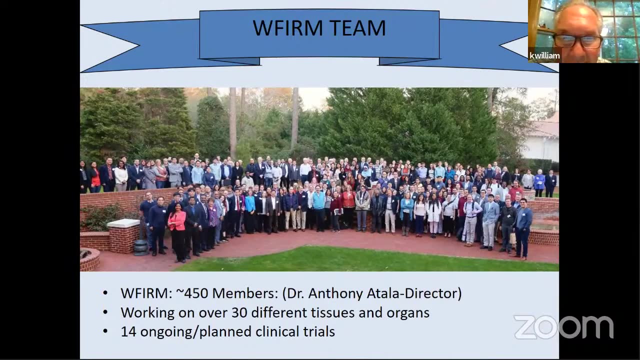 into phase three clinical trials and a product for surface. We have several standalone companies usually required for phase three studies, And this really accelerates our ability to translate our studies. 450 members- I'm in there somewhere, I'm not quite sure where. 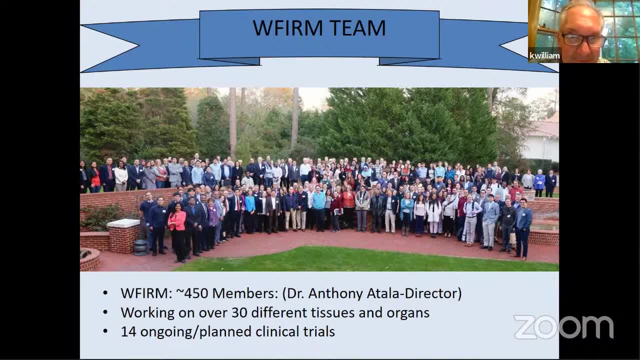 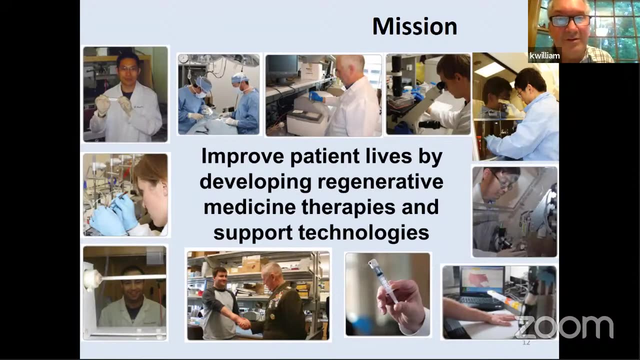 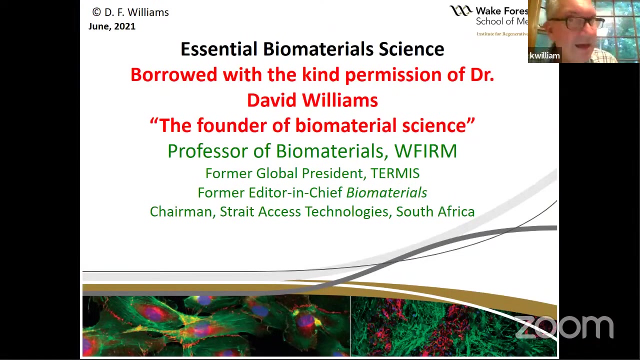 I'm Anthony Atala is our director. We have 14.. Actually, we have about 17 ongoing planned clinical trials right now And again, our objective is to improve patient lives by developing regenerative medicine therapies and support technology. Okay, So today I'm going to talk to you about one aspect of regenerative medicine. 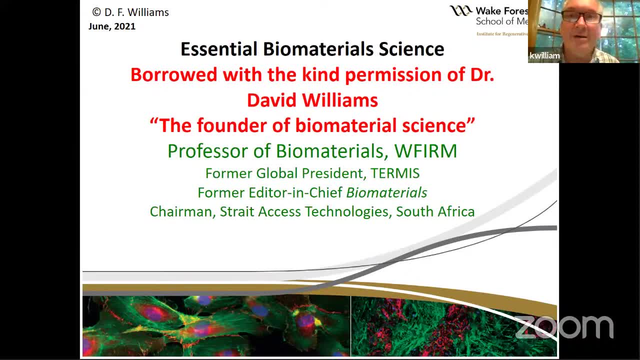 And that is the role of regenerative medicine, And that is the role of regenerative medicine And that's biomaterial science. I borrowed these slides with time permission of Dr David Williams, who is basically the founder of biomaterial science. He has written many. 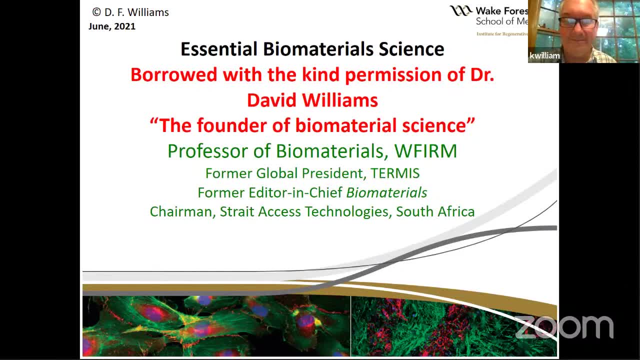 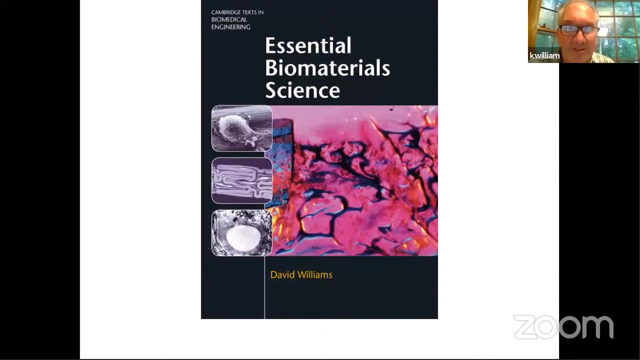 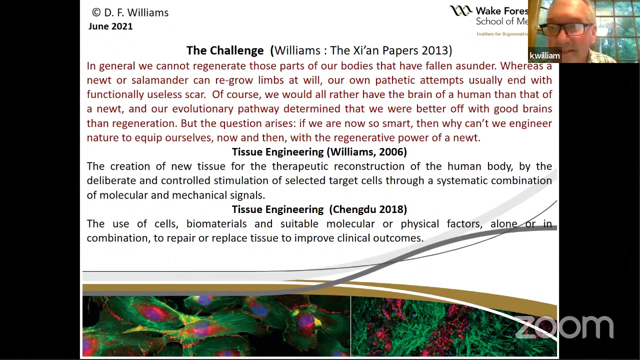 many books. He is the leading. He lives in South Africa, works with us and is just a leader in this. He has written many books, including the essential biomaterial science books, And he has really defined this new science which began rather simply And I think, if you get 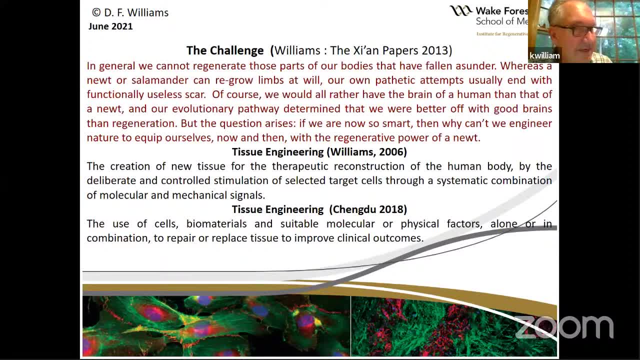 anything out of this. I want you to get the idea of the challenge of trying to define what tissue engineering is and how intricate and advanced, and how much further we need to go in order to bioengineer tissues. In general, we cannot regenerate those parts of our bodies that have 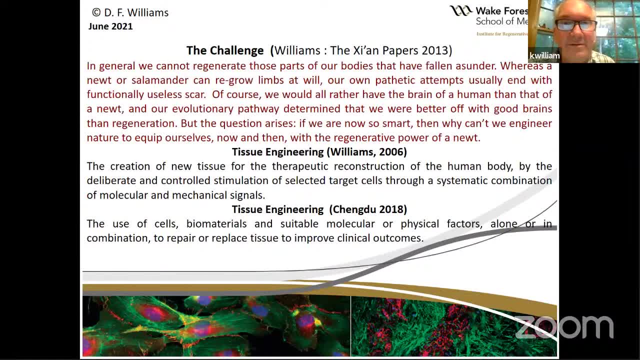 fallen asunder, Whereas a newt or salamander can regrow limbs at will. our own pathetic attempts usually end with functionally useless scar. Of course, we'd rather have the brain of a human than a newt, And our evolutionary pathway determined that we were better off with good. 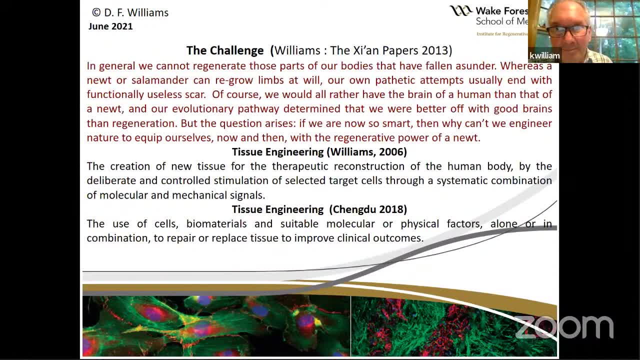 brains. But the question arises: if we're so smart, then why can't we engineer nature to equip ourselves now and then with regenerative medicine, And I think that's a really important offering. As a recurrent question, people want to know how they can prepare themselves for the 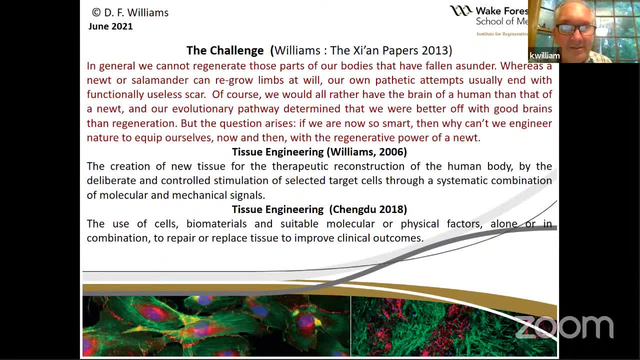 future And why Define you 만들어 off? tissue engineering is defined as a creation of new tissue for the therapeutic reconstruction of the body by the deliberate and controlled stimulation. Stay at home. do plastic surgery at home. ozone is physical factors alone or in combination to repair or replace tissue to improve clinical outcome. 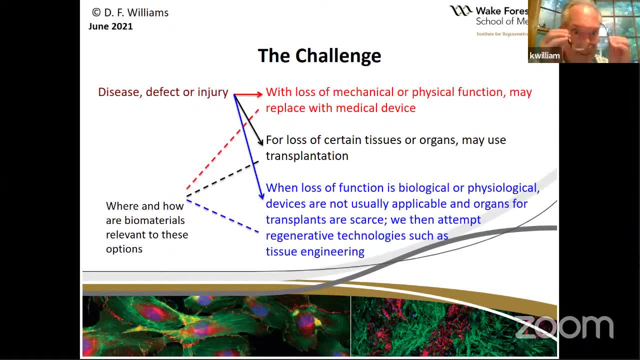 So what's the challenge? Well, you have a disease, a defect or injury. you either need to replace the organ or tissue with a loss of mechanical or physical function. may replace with it, might be able to replace it with a medical device For a loss of certain organs. may be able to. 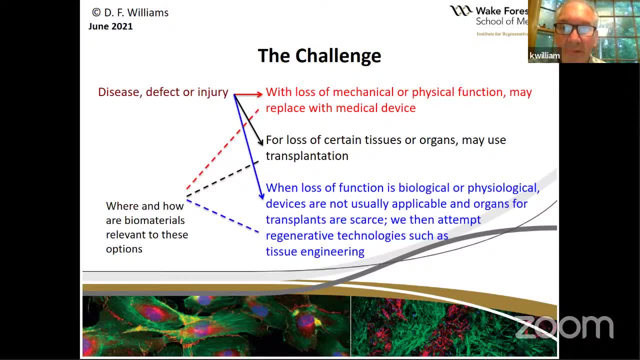 go to transplantation When a loss of function is biological or physiological. devices are not usually applicable And organs for transplants are scarce. For instance, for every seven people that need a kidney transplant, there's only one available. So that means six people did not get it. 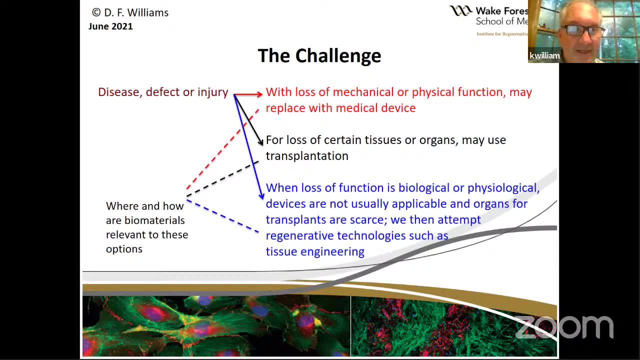 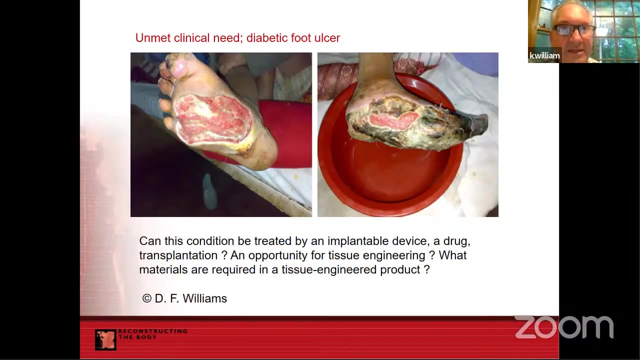 We attempt to regenerate technologies such as tissue engineering. So, as you can see, where and how are biomaterials relevant to the these options? So that's what we're going to talk about. So this is a unmet clinical need by diabetic foot ulcers. Can this condition be treated by an implantable device? 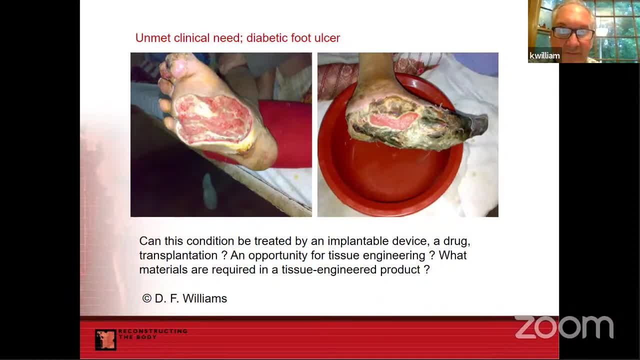 or a drug, The opportunity for tissue engineering? what materials are required to engineer tissues to repair this horrific injury? Well, one of the things we have to do is we have to do a lot of work, We have to do a lot of work. We have to do a lot of work. 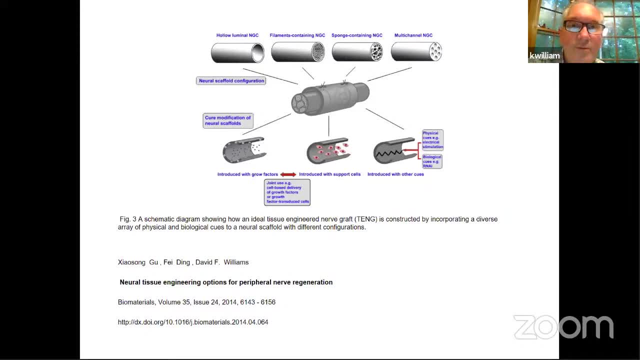 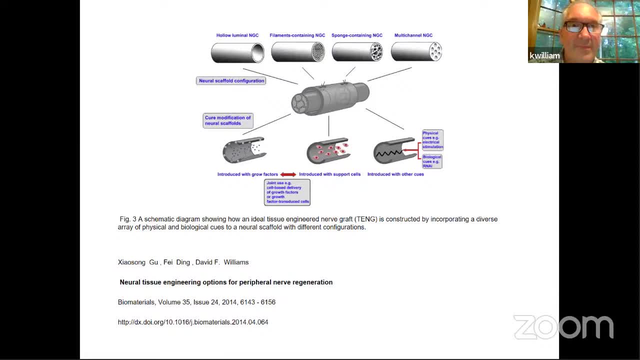 I don't know if you can see my cursor here, but if you look along the top there there are several different conduits. You put two ends of a nerve in there and then you create a nice environment for that nerve to regrow. You can do that by creating little honeycombs, little other different kinds of 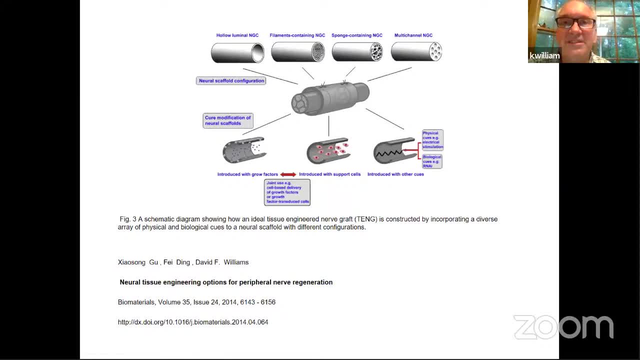 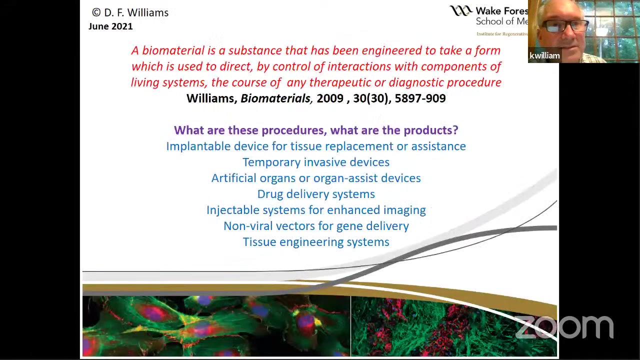 spaces for cells to grow. You can charge this with molecules that promote growth, put cells in there that promote growth and then you apply physical or like electrical stimulation across it to cause those nerves to go together. So biomaterial. I just showed you one. 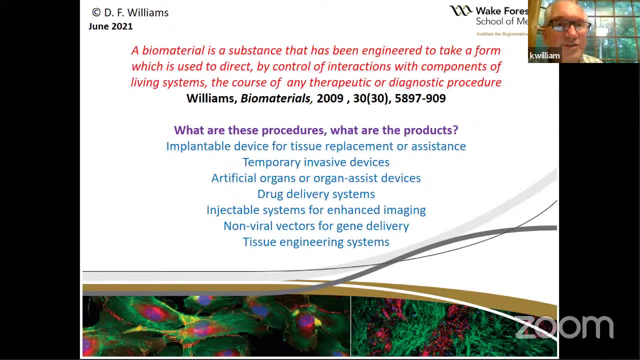 is a substance that has been engineered to take the form which is used to direct by controlled interactions with components of living systems. For instance, that conduit is in the shape of a nerve. you put two ends of the nerve in and you stimulate it to go together. What are these? 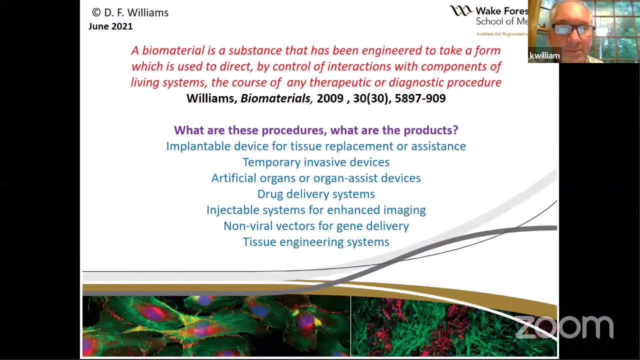 procedures. What are the products? Well, implantable device for tissue replacement or assistance, temporary invasive devices, artificial organs or organ assist devices, drug delivery systems, injectable systems for enhancing imaging, non-viral vectors for gene delivery and tissue engineering systems. That's a lot. I mean, that is really a lot you have to. 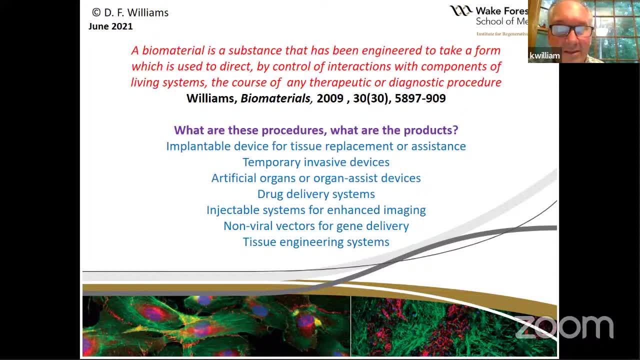 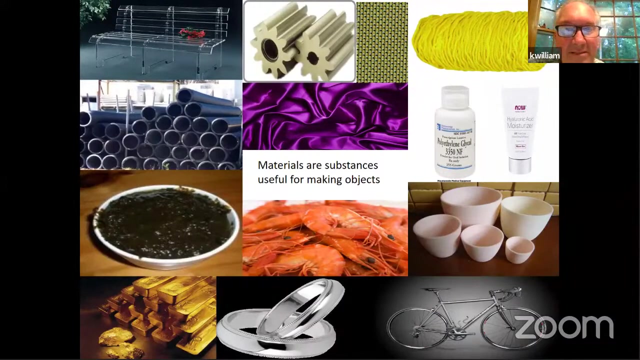 bring to bear on this problem, And it is getting more and more complex The more we know. they always say: the more you know, the less you know. And what we're finding is: all these things must be brought together. So what kind of materials do we have? Well, many, Anywhere, from plastics. I'll give you a little bit. 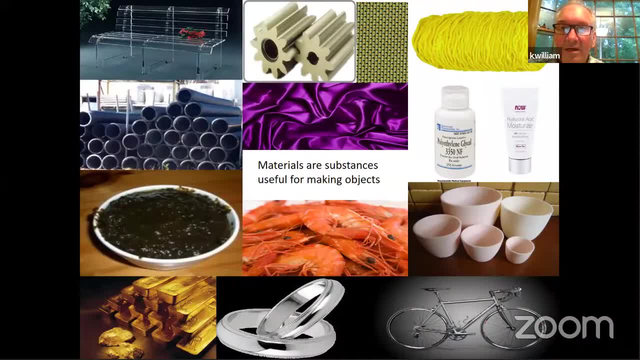 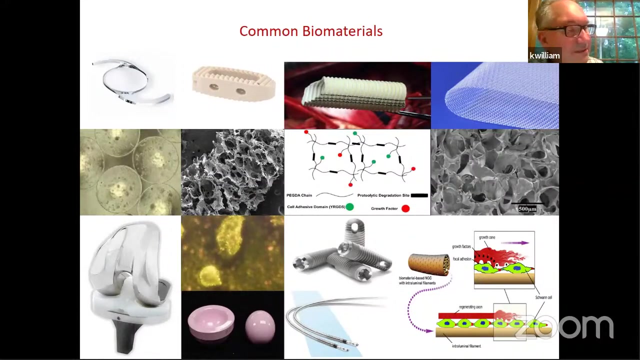 more detail on this: Mechanicals, ceramics, polyethylene glycol. there are chemicals: chitosan from udang, seaweed, ceramics, gold, silver, Many, many different types of materials, chemicals- And let me just show you For instance, last one. 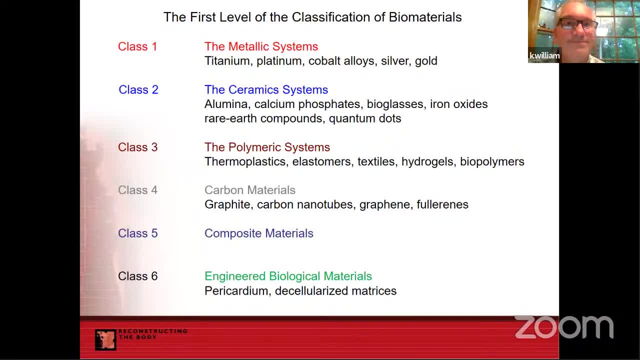 there are metallic systems made up of titanium. I don't know if any of you had a joint replacement or had to have something fixed- that they put in titanium plates nowadays- Platinum, cobalt alloys, silver, gold. I'll explain to you how all these come together. The ceramic systems with alumina calcium. 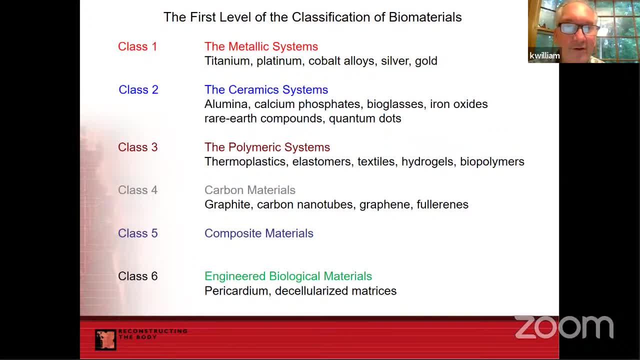 phosphates, bioglasses, iron oxides, rare earth compounds, quantum dots, polymer systems, thermoplastics, elastomers, textiles, hydrogels, biopolymers, carbon materials like graphite and carbon nanotubes, composite materials that are some combination of the class one through four. 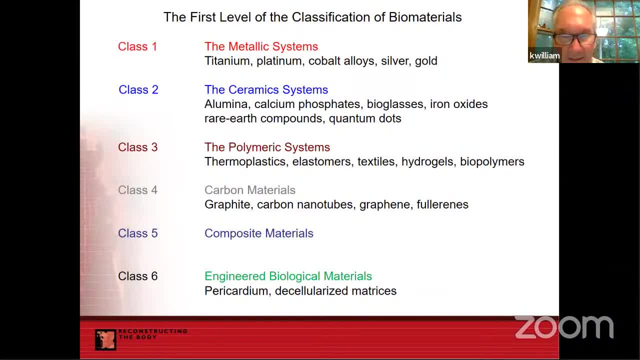 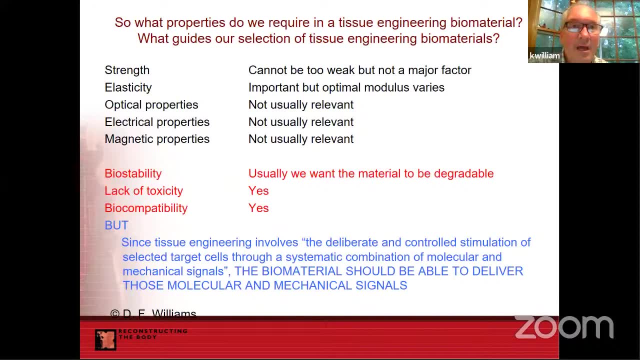 and engineered biological materials, And I'm going to talk to you right at the end. talk to you about pericardium and decellularized matrices that we're using now. Okay, so what should these materials have in them If you're going to put them in the body? 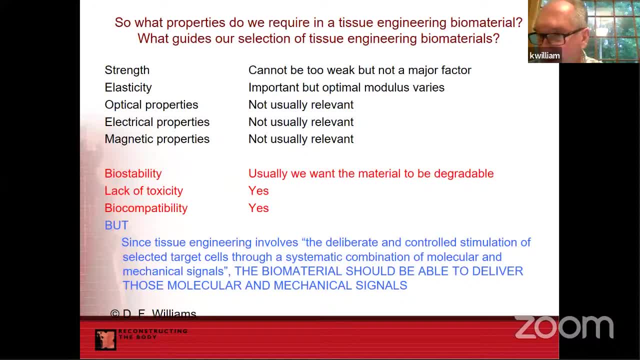 and you want them to regenerate tissue, you want them to be functional. what, what, what guides it? Well, it's kind of impossible, but you have to have strength. Can't be too weak, but not a major factor, For instance, if you put in an artificial. 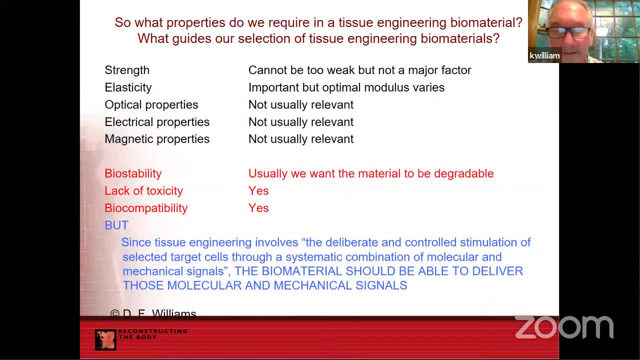 artery into the arterial side of the body. it must withstand all the stress forces and pressures that are on the left side of the body. Elasticity: that artery has to expand and contract Optical properties, usually not relevant Electrical properties, unless you're trying to stimulate growth with electricity, not that important. 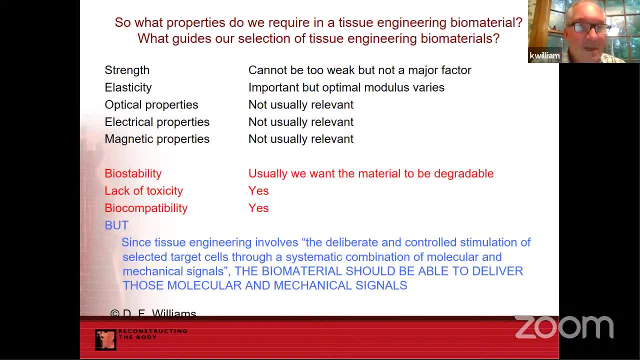 Magnetic properties, not usually relevant, Now here are important ones. Hmm, Biostability: The trick is: get a polymer, get a material. we want it to degrade eventually because we want it to be taken over by natural tissue. 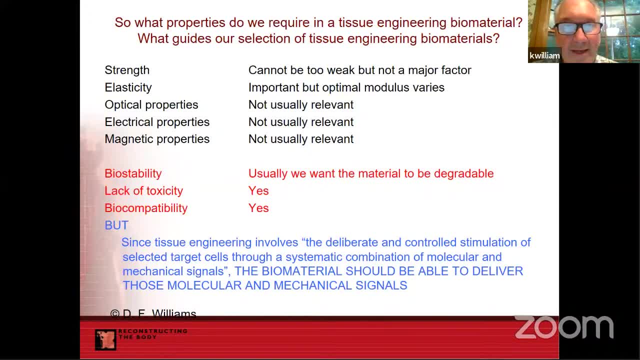 But it can't degrade too fast, or it's gone away and the new tissue hasn't formed and it falls apart. Lack of toxicity, of course you can't have that Biocompatibility. The body cannot build a horrendous immune response to it and basically destroy it before it ever has a chance. 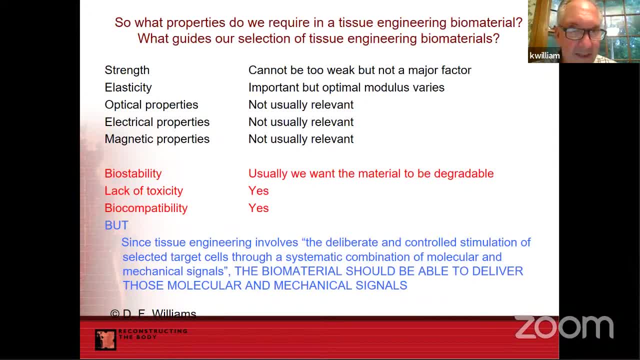 to uh form. But since tissue engineering involves the deliberate and controlled stimulation of selected target cells through a systematic combination of molecular and mechanical signals, the biomaterial should be able to deliver those molecular and mechanical signals. So it's not good enough just to put in a polymer and hope something good happens. 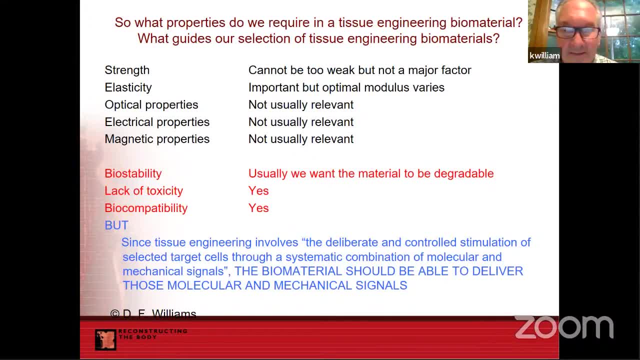 Kind of where uh regenerative medicine started. but we've expanded and gotten much, much more sophisticated since then and are now incorporating molecular and mechanical signals to aid in the regeneration of that tissue. Can't just put in the biomaterial and let it sit there. 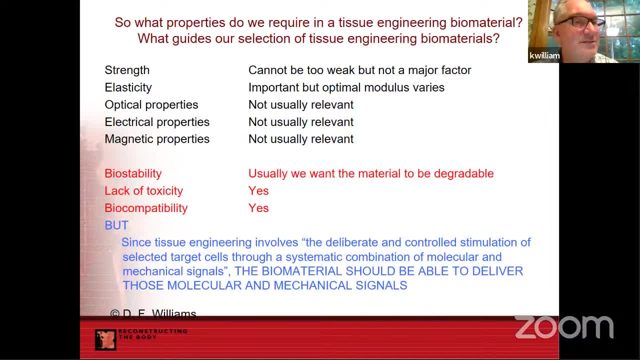 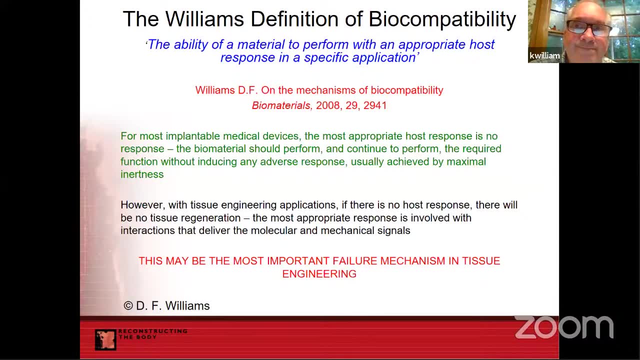 There has to be added things like cells and growth factors, and I'll talk a little bit more about that. Okay, for most implantable medical devices, the most appropriate host response is no response. right, You don't want to, um uh, attack it and wipe it out? 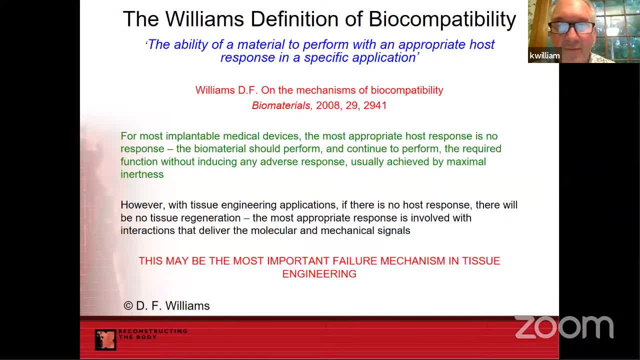 The biomaterial should perform, and continue to perform, the required function without inducing any adverse response, usually achieved by maximal inertness. However, that's- it's- it's a problem With tissue engineering applications. if there's no host response, there'll be no tissue regeneration. It'll just sit there like an inert putting in something inert. 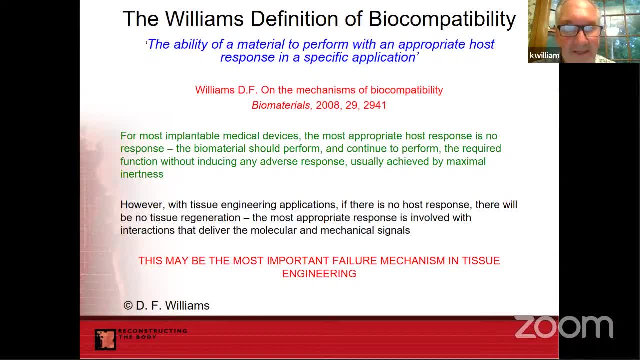 and just leaving it underneath the skin. nothing's going to happen to it. So the most appropriate response is involved with interactions that deliver molecular and mechanical signals. So you want it to interact with the body, but only in a good way. Again, you want it to interact, but only in a good way. This may be the most important failure. 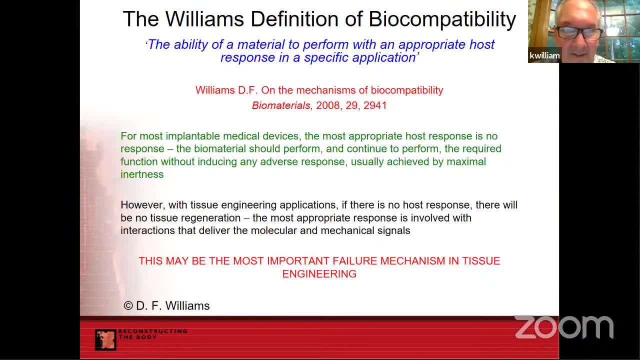 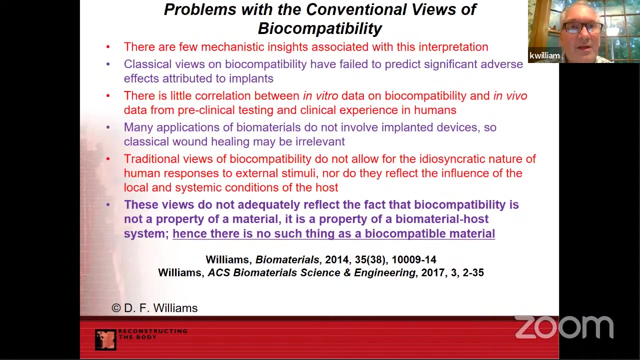 mechanism in tissue engineering Very, very important to failure is that you put in something that body attacks it but it doesn't have a chance to release those signals that talk to the body, basically So that you get regeneration. Okay, Let me move this a little bit. 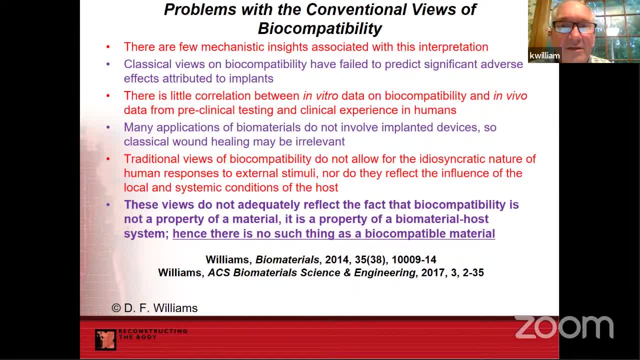 There are a few mechanistic insights associated on what biocompatibility is. Classical views on biocompatibility have failed to predict significant effects attributed to implants. That's because the human body has a very, very sophisticated system to attack worn objects. Even worse, in preclinical studies, the immune system of a cow 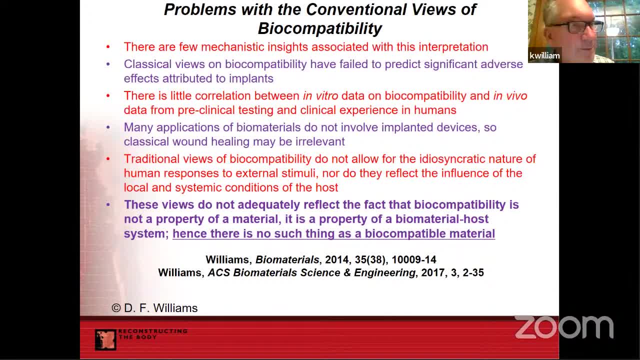 or a sheep is very different than immune, the system of a primate, whether it be a monohuman primate or a human being, and very different from a cat and a dog, And so something out, you got to test it out eventually in the species that you want it to work in. so you 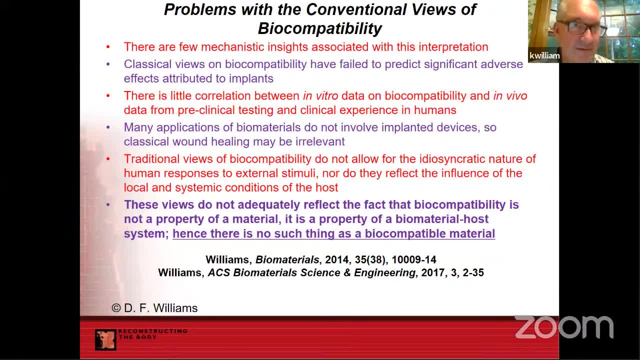 have to. you have to, um, make those uh react with the species you're trying to put them in. there's little correlation between the in vitro data on biocompatibility. that's why i just just just uh, that's just what i just said- is, a lot of times in vitro data do not predict in vivo and a 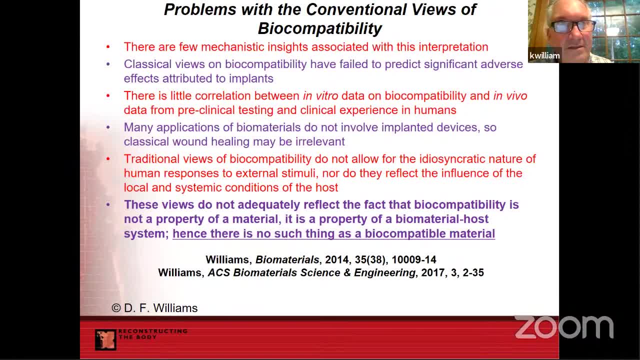 lot of times in vivo clinical, preclinical data don't predict clinical studies. oh many applications of biomaterials do not involve implanted devices, so classical wood healing may be irrelevant. traditional views of biocompatibility do not allow for the idiosyncratic nature of human responses to external stimuli. 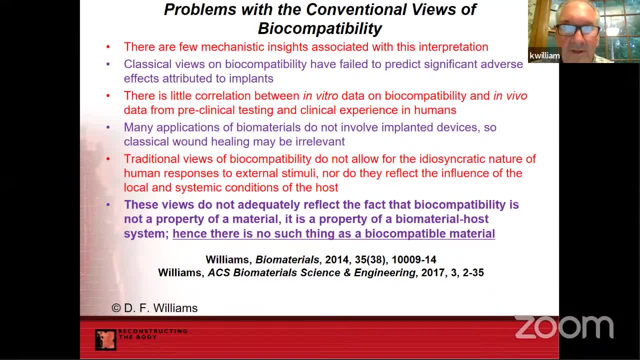 Again, humans are very different. We're not newts, nor do they reflect the influence of the local and systemic conditions of the host. Again, immune system: very different. Humans also have enzymes that other animals do not have. vice versa. 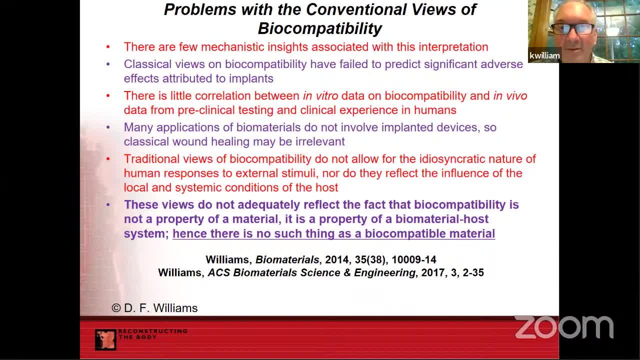 These views do not adequately reflect the fact that biocompatibility is not a property of a material. It is a property of biomaterial host system. Hence, there is no such thing as a biocompatible material. You have to have a biocompatible pair. 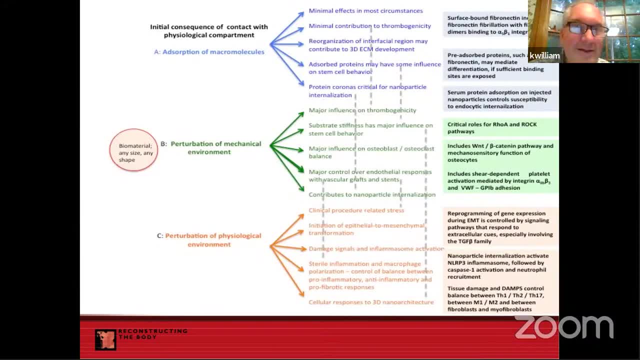 This is a very complicated slide. Don't worry about the details. I think I told Irma, yeah, you can go ahead and get PDFs of these if you want to, and people can go over them in more detail. But what this slide basically? 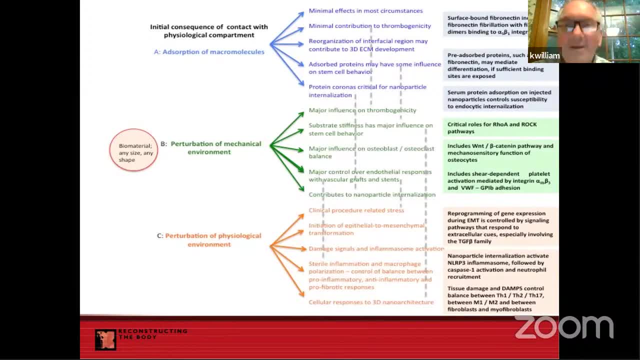 points out, there's blue, green and sort of yellow red down there at the bottom. What it is is: once you put a biomaterial in, several things must happen. You must have absorption of macromolecules. It's going to be exposed to the body. 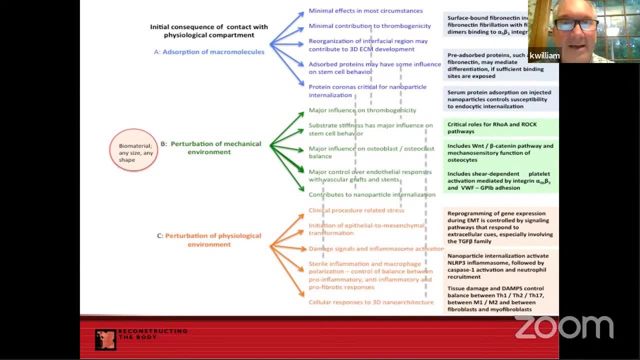 in its initial immune system. It must get used to that. It must survive that. It must also survive mechanical environment, For instance. if you don't have the right cues in there, a implant that you want to become a bone will become collagen, a joint. 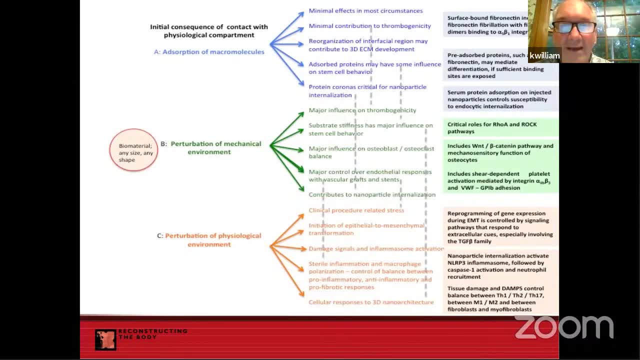 but it will not become bone. So you have to- it has to withstand that. And then the physiologic environment. There's going to be inflammation, There's going to be stresses, clinical procedures related stresses, And you must have the body react to that. 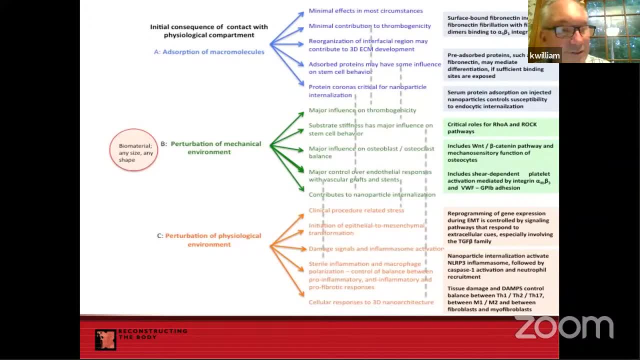 and begin to establish the cell host interaction and bio talk that goes back and forth. Very important Cells and matrix talk to each other And if you don't have a biomaterial that can do that, it's not going to turn out the way you want it to turn out. 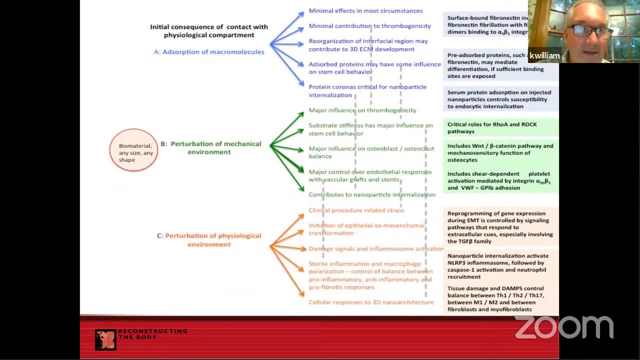 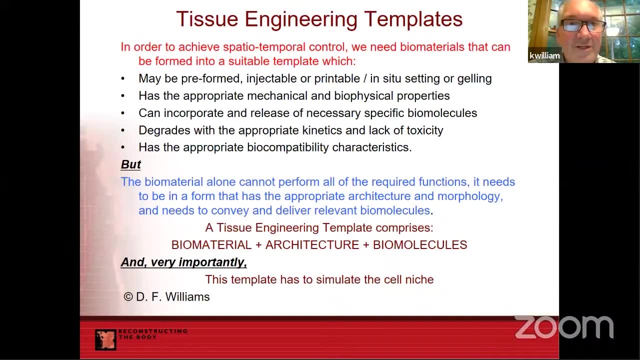 Very important that all three of those are met. Very important that all three of those are met By any biomaterial you put in, of any size and any shape. In order to achieve spatial, temporal control, we need biomaterials that can be formed. 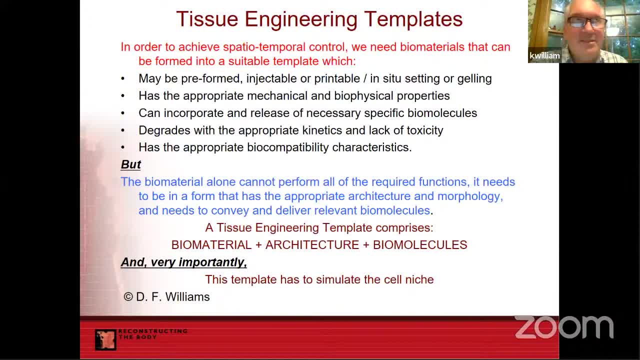 to a suitable template. Okay, One thing that I haven't said yet- and it's very, very important, is: a biomaterial must create a niche for cells to grow in, for nerves to grow in, and it must be spatially correct for those cells to go in. 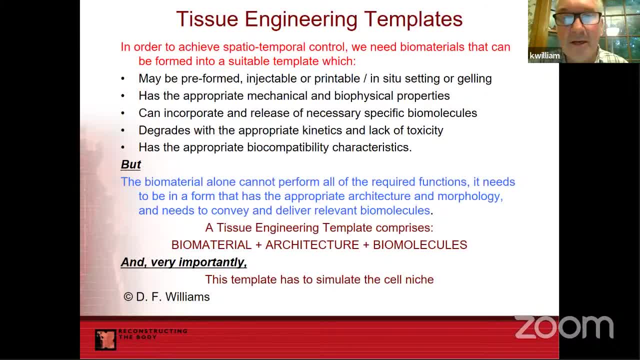 You must make a nice home for them, where they want to live, basically, And it's very important that they have that nice home and that where they are, they are beginning to produce the biomolecules that you want them to. Biomaterials must be formed with a suitable template. 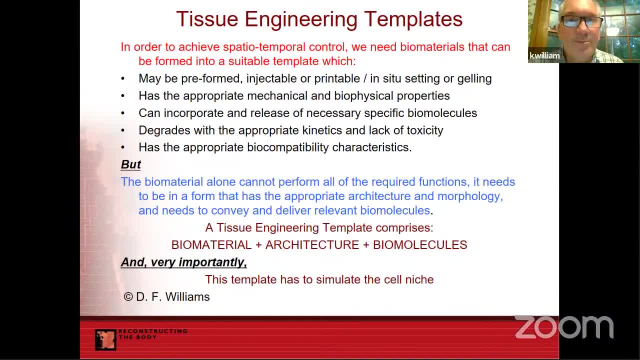 which may be preformed, injectable or printable. has the ability to produce the biomolecules and so forth. appropriate mechanical and biophysiologic properties can incorporate and release necessary specific biomolecules. degrades with the appropriate kinetics, not too fast, not too. 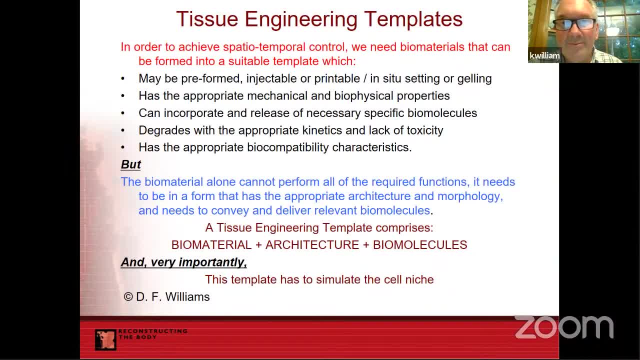 slow and lacks of toxicity. When those materials degrade, they can't produce toxic chemicals. It has the appropriate biocompatibility characteristics, but the biomaterial alone cannot perform all the required functions. It needs to be in the form that has appropriate architecture. 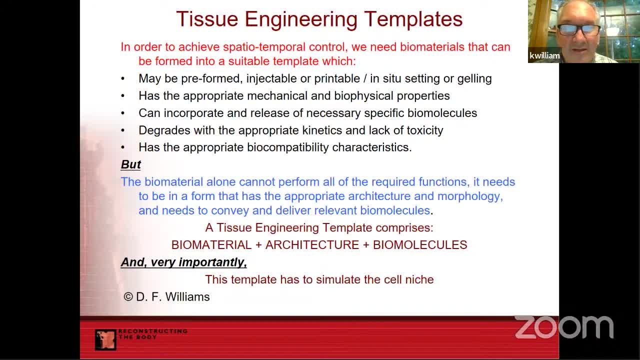 forms a niche and morphology and needs to convey and deliver relevant biomolecules. A tissue engineering template comprises a biomaterial, a proper architecture and biomolecules. Sometimes those biomolecules are produced by the cells you put in there. And, very important, this template has to stimulate the cell niche. 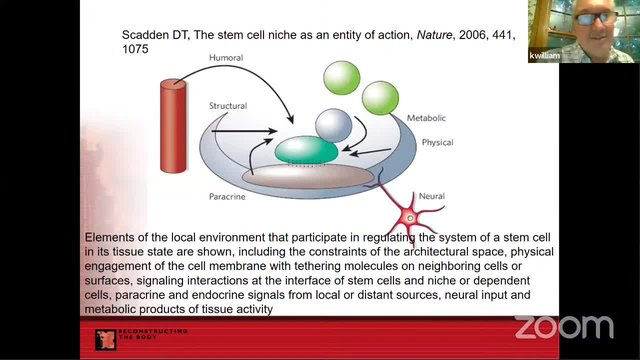 We'll talk about that. This slide basically just outlines this. So if you look at the kind of crescent-shaped blue there, that is basically the space that the tissue must form. It must interact with neural, metabolic, physical forces, paracrine forces, structural constraints. 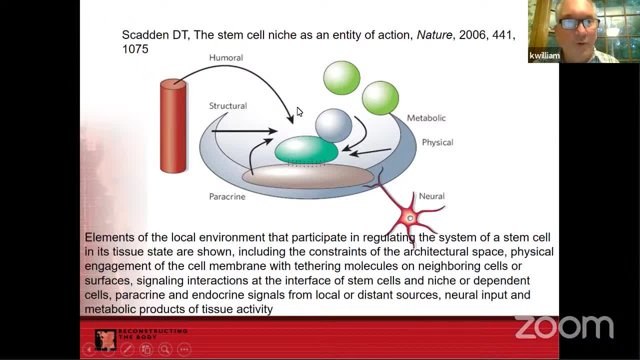 and humoral from outside that body form, forming hormones et cetera, to make that all work And, as you can see, that's a lot of things to bring together for a tissue to grow. So it's getting more and more complicated as we begin to. 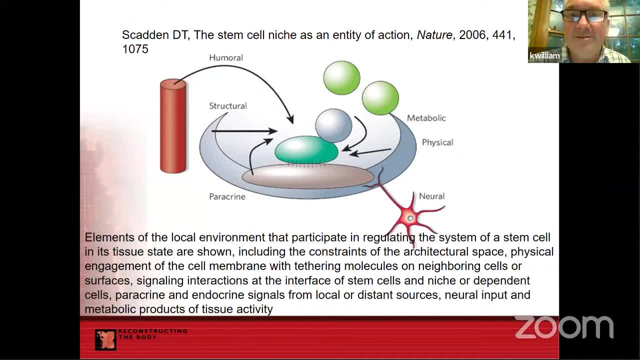 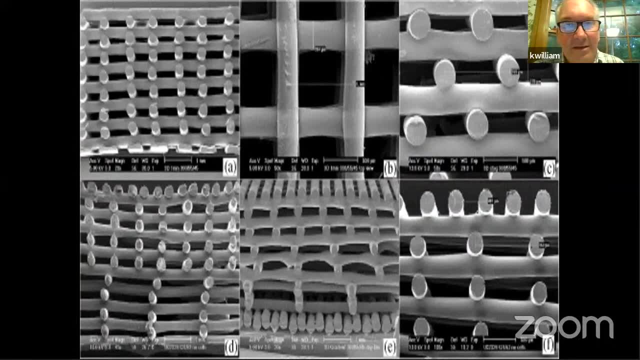 understand more of what these cells and these biomaterials must have to be successful. This is what some of them look like. You can make these. You can make little nanoparticles You can make I think this is more silver and probably a maybe gold and maybe some kind of side. I'm not quite sure what else is in there, But can you see? 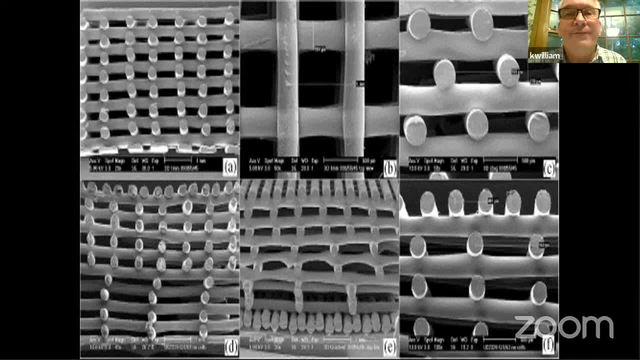 the different forms and the different little squares. It looks like a checkerboard And you can make a biomaterial. have these little compartments where cells can crawl in and matrix can crawl in and it can form, And then you want that checkerboard. 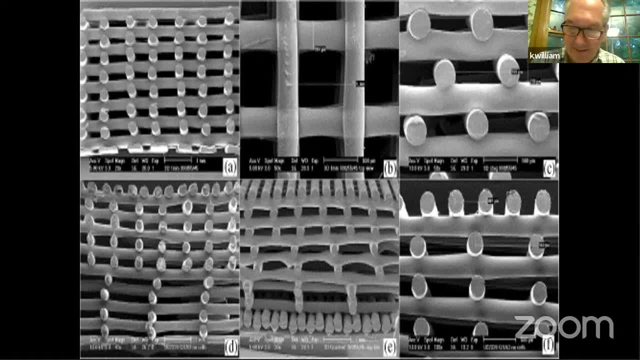 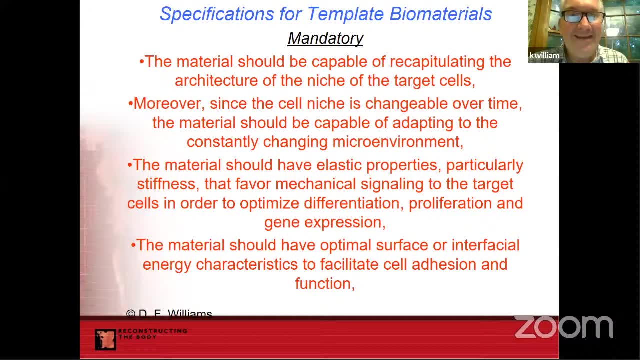 to disappear someday. So it's complicated, Mandatory. The materials should be capable of recapitulating, Recapitulating, excuse me the architecture of the niche of a target cell, Moreover, since the cell niche is changeable over time. 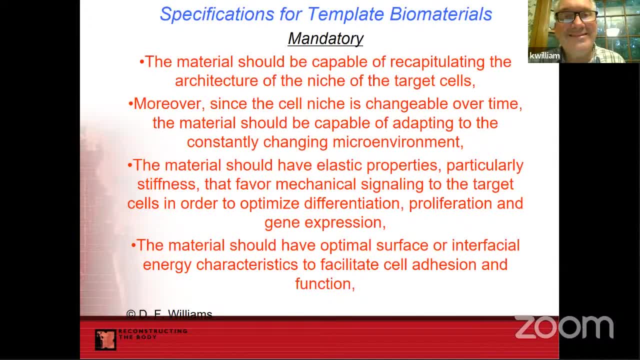 the material should be capable of adapting, constantly changing microenvironment. For instance, if you put something in for the first week, first two weeks, it's going to have a very different metabolism associated with that implant than it is later. Things are going to change. There's going to be changes in the amount. 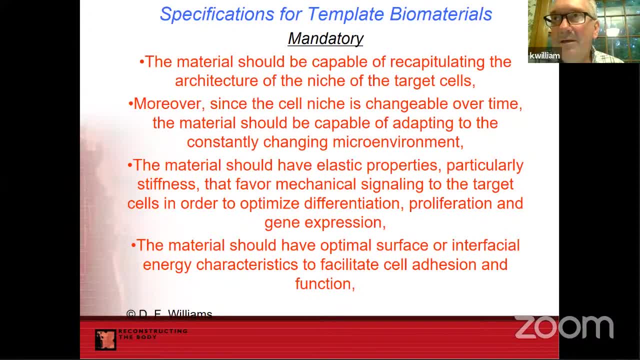 of oxygen available to that implant. the growth factors that are being formed As the cells begin to talk to each other. they're going to create a whole metabolic environment there and the implant must be able to adapt to that. It should have elastic properties, particularly stiffness. 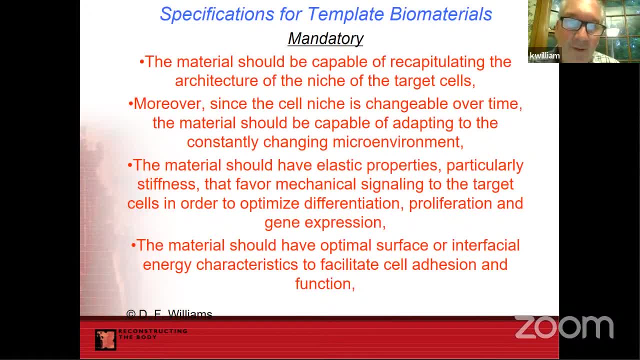 For instance, you put in an artery or a heart valve, it has to be able to withstand the pressures of the heart. If you put in a bone implant, it must be able to hold and maintain the limb or wherever it's put. It should have optimal surface or interfacial energy. 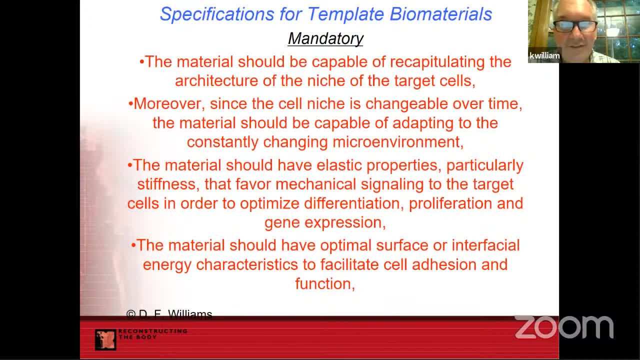 characteristics to facilitate the implant Cell adhesion in function. What that means is the surface of that biomaterial has to be- for a better word- charged so that it can accept and will attract cell adhesion. It can be done now with nanoparticles. We used to not be able to. 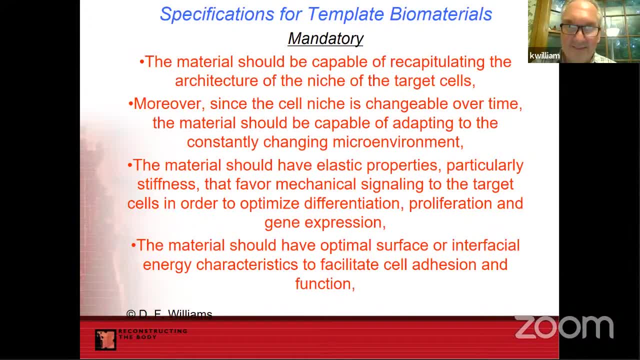 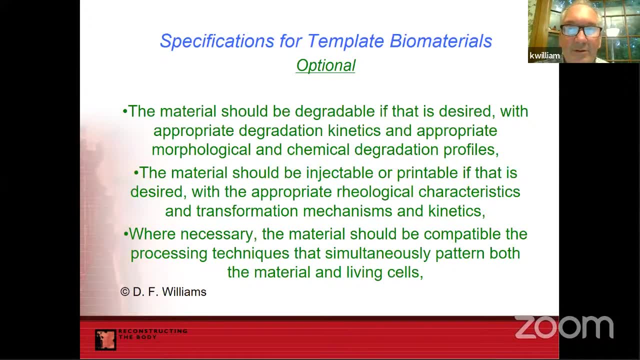 use those. but we can now- Very important that all that happens. Okay, a specific Indications for template biomaterials. The material should be degradable if that's desired. Some: you don't want them to go away, most of them you do with appropriate degradation kinetics. not too fast, not too slow. 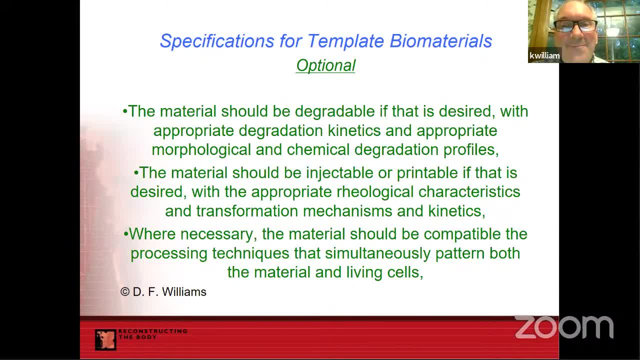 And I know I'm repeating myself, but these are important factors- Appropriate morphological and chemical degradation profiles. You don't want it to degrade and create something toxic that will chew up the tissue around it. The material should be injectable or printable. 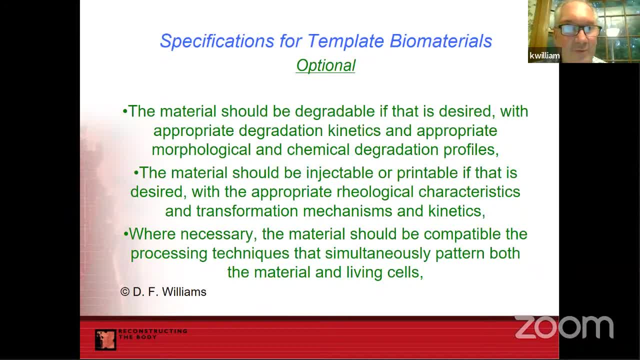 If that's desired, with the appropriate rheologic characteristics and transformation mechanics and kinetics Where necessary. the material should be compatible with the processing techniques that simultaneously pattern both material and living cells. What that means is you got to be able to successfully reproduce that design that you want from implant to implant to implant to implant. You can't vary. 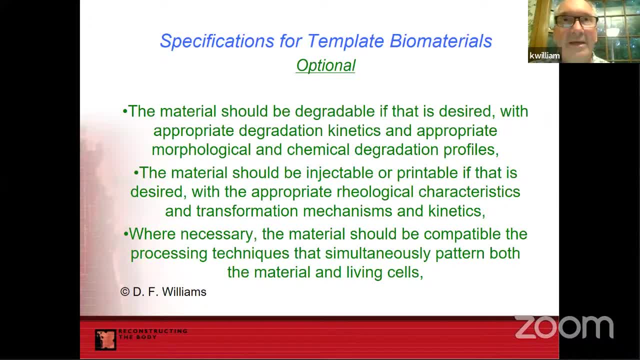 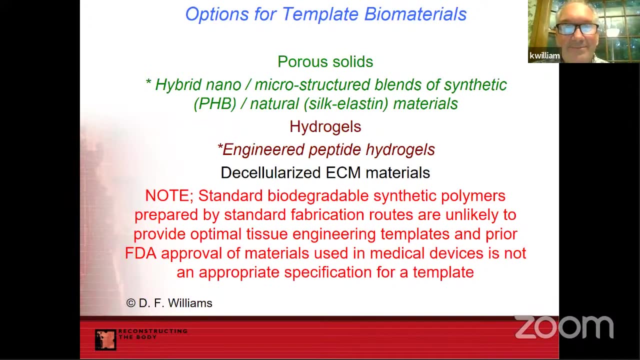 a lot of the things and expect that implant to behave the same. It has to be consistent, It has to be the same if you want it to react the same. Okay, porous solids. This is kind of where we began. I think you've probably heard about biospinning, where they used 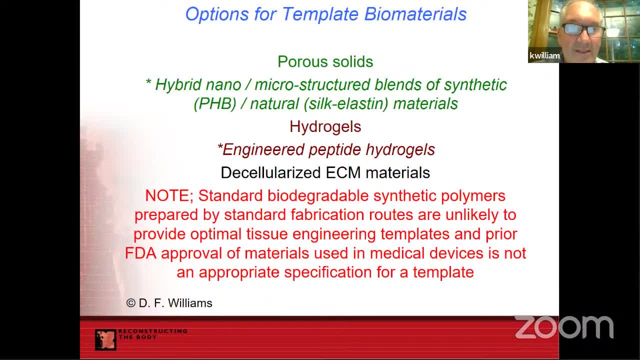 hydrogels, and I think I have a picture of it coming up. but the standard biodegradable synthetic polymers prepared by standard fabrication routes are unlikely to provide optimal tissue engineering templates and prior FDA approval. Prior FDA approval of the materials used in a medical device. 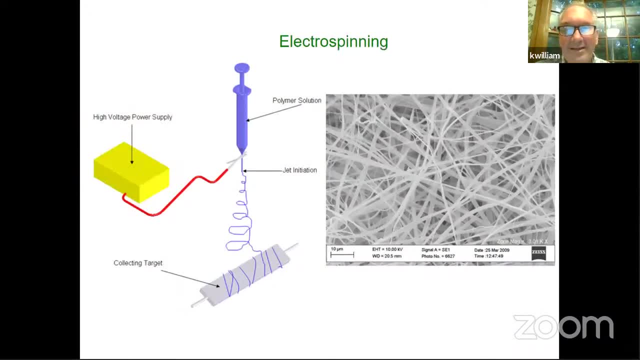 is not an appropriate specification or template. This is how we did electrospinning. It's like a spider web And the polymer solution comes out of the syringe. It's jet initiated high voltage power supply. It turns it into basically string, a collecting target. It can be round, It can be flat, And this is the 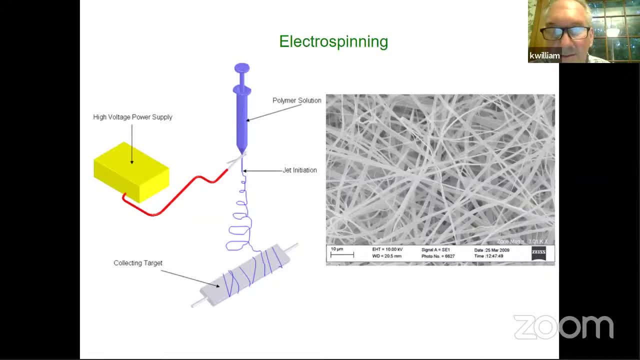 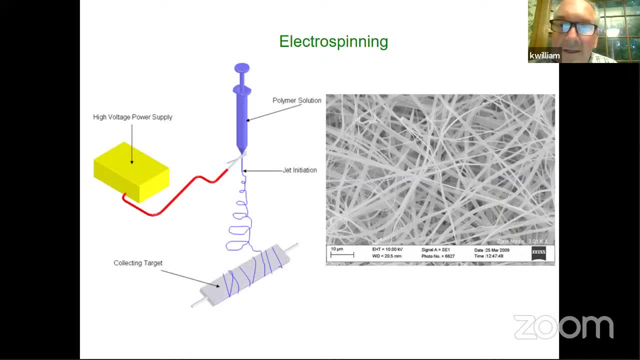 They're usually not very strong if it's just a simple polymer solution. But I hope you can understand. each one of those is going to look different. You can control the diameter a little bit, You can control how it's made, But the next one picture I could show you it'll look different. 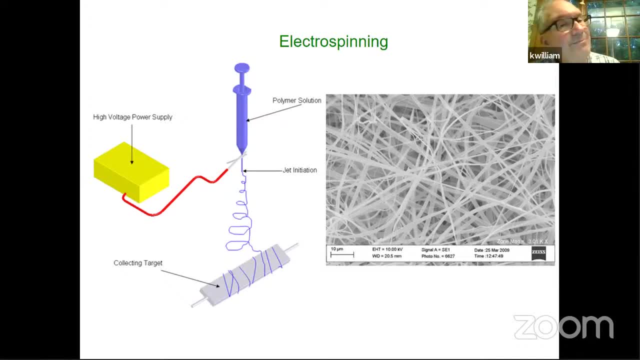 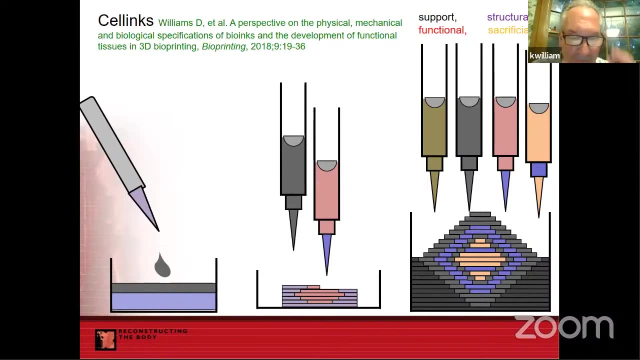 And that means you have the potential of it not behaving similarly. This is kind of here's where we've gotten with it And this is really cool. This first one is basically: you put a polymer on a plate. it spreads out and doesn't have much strength. It. 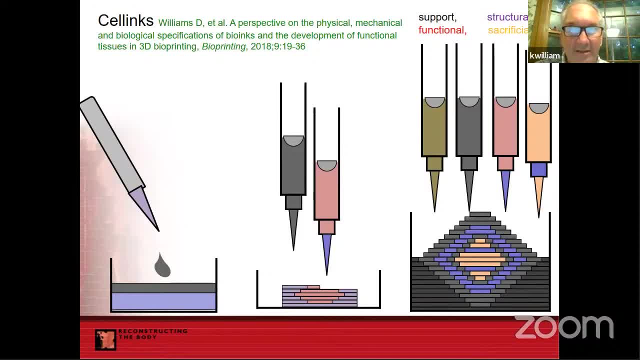 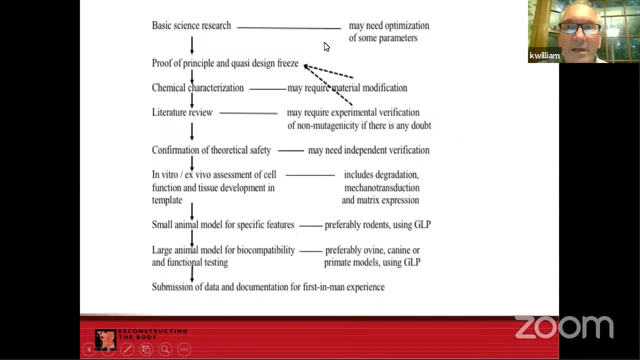 doesn't really have much form. So what they do now is they have a series of biomechanical. Let's see if I can do that. Let's see. Sorry, How am I going to do that now? No, I cannot. I wonder if I can. 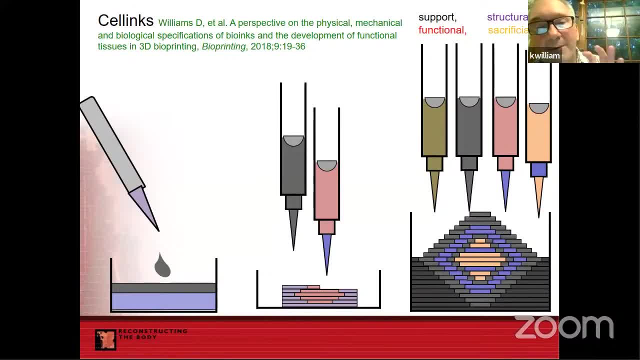 That's all right, I can wing it. What they put now to make something is they do a lot of inkjet printing And they will put down various aspects of a tissue. They will put down structural here in blue, which could be anywhere from gold, silver. 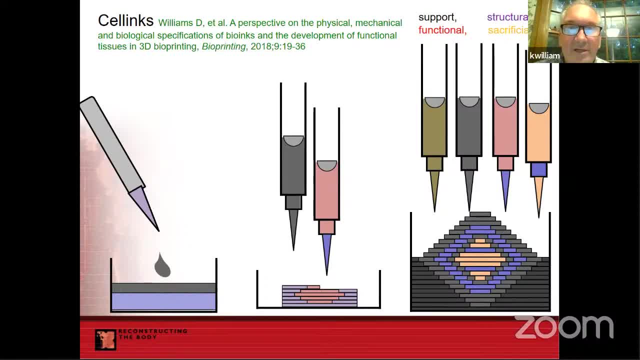 something to give it form. It can be collagen, It can be fibrin, And then they also put down here in pink. they'll put down something that's functional, For instance a girl factor, And they'll make it into a plate or a circle. 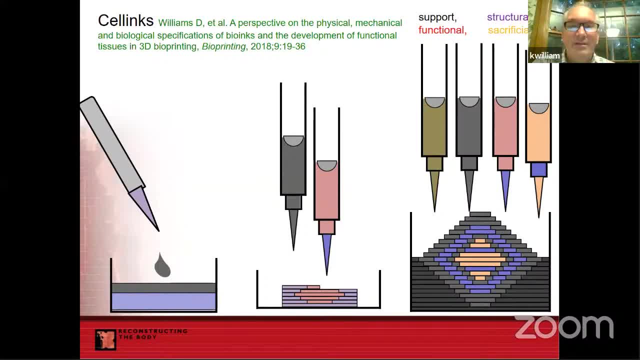 And so what you want is you want that structure to support the functional aspects for a while until it goes away. Now they've gotten more sophisticated and they put in sacrificial structural thing. so here's something you kind of want to keep around. that can be gold, that can be. 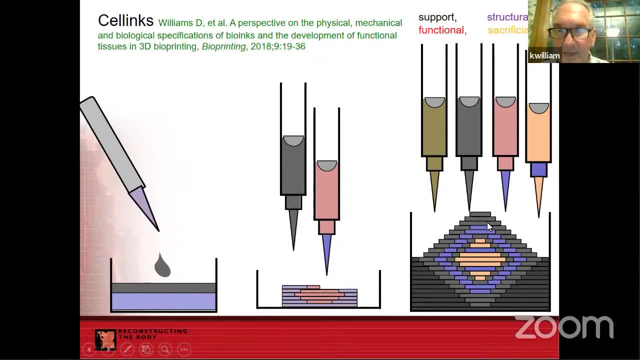 silver. that can be something that just really doesn't go away very much. then you have functional and then they have what are called sacrificial biopolymers and those are strong for a while and they are put in there simply so they'll go away. they'll go away pretty quick and allow the 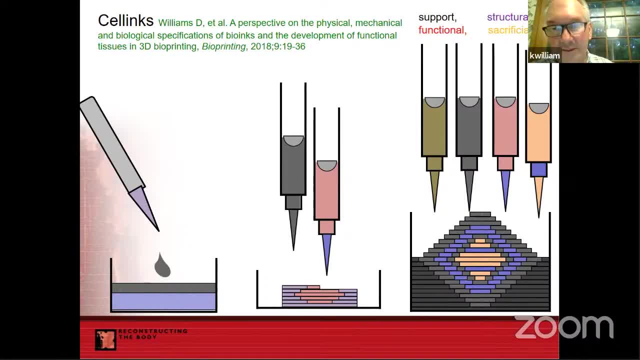 function to occur, while the ones that the structural things they put in there to last a little bit longer stay there longer. so this is like a very complex sandwich that they put in which contains functional structural, sacrificial chemicals to make a implant. so, as you can see, 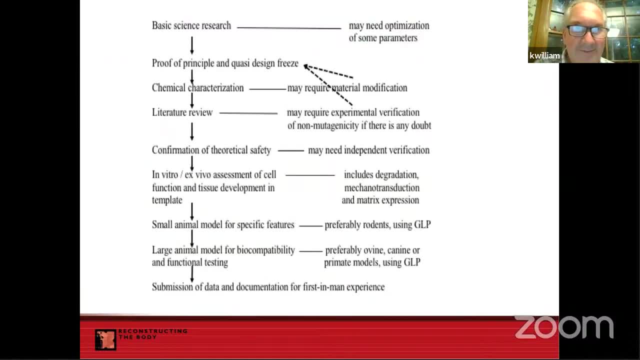 this is getting very, very, very sophisticated. so what's the process of all of this? you get some yellow. it seems to be working. your biochemist, your chemistry people came up with something really good. so what do you have to do? well, i have to do some proof of principle studies, then some chemical. 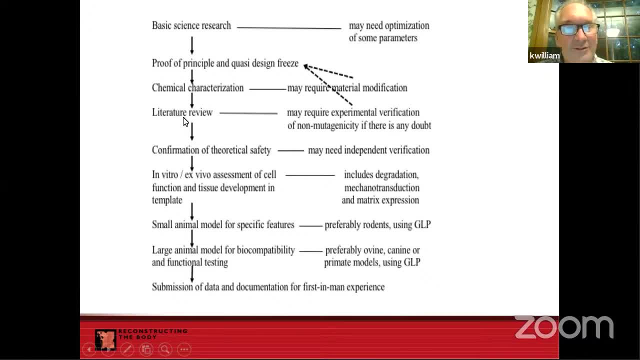 characterization. always do literature reviews to make sure somebody didn't do it first. confirmation of theoretical safety may need independent verification in vitro. ex vivo assessment of cell function and tissue development in the template includes degradation, mechanical transduction and matrix expression. then you got to do some small animal studies, usually rodents, then large animal models for biocompatibility. 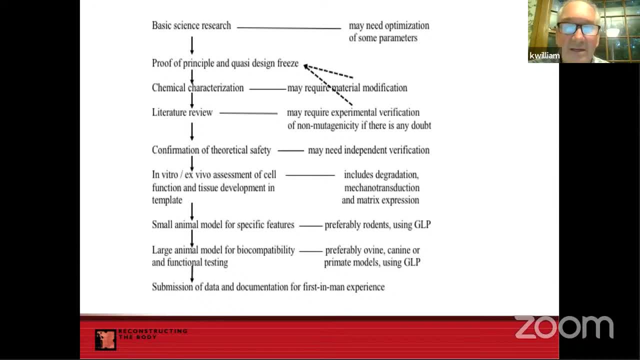 functional testing. and one thing: this did not include safety. first of all, safety. a lot of times i use sheep, dogs or primate models doing good laboratory practices, and then you submit the data and documentation to the fda for sacrifice, and then you submit the data and documentation. 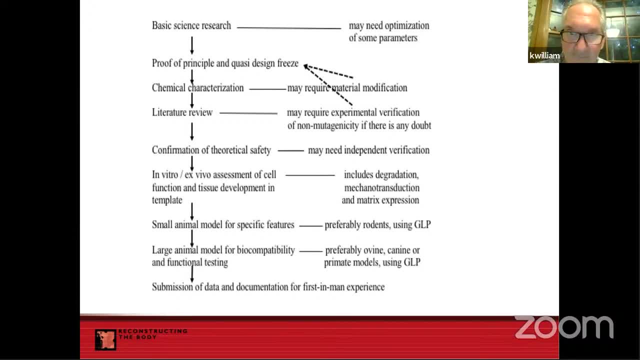 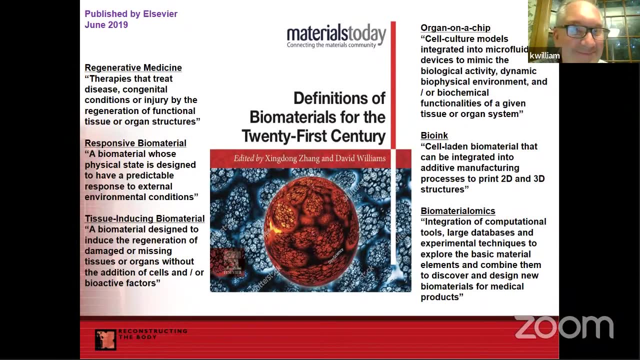 to the fda for sacrifice, and then you submit the data and documentation to the fda for first-in-man experience. So what are the definitions of materials for the 21st century? Well, regenerative medicine are therapies that treat disease, congenital conditions. 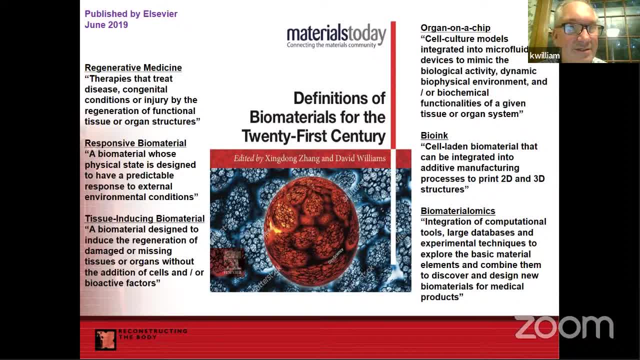 or injury by the regeneration of functional tissue or organ structures. Functional, not just space-taking. Responsive biomaterials are as a biomaterial whose physical state is designed to have predictable responses to an external environmental condition. They must be painstakingly put together, They must be consistent so that when you go from person, 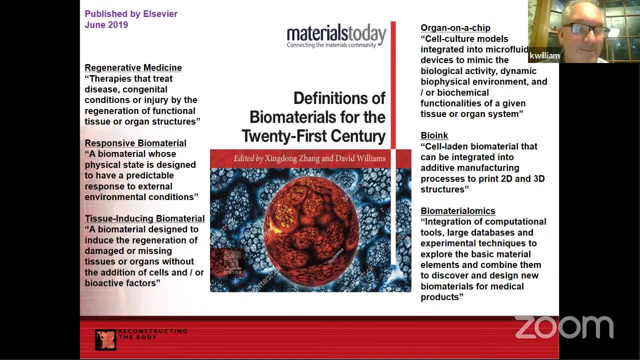 to person to person or animal to animal. you're putting in the same thing. It's like you want to put in the same chemical to a reaction in the same concentration. It's the same principle there, It's just. this is a whole bunch of. 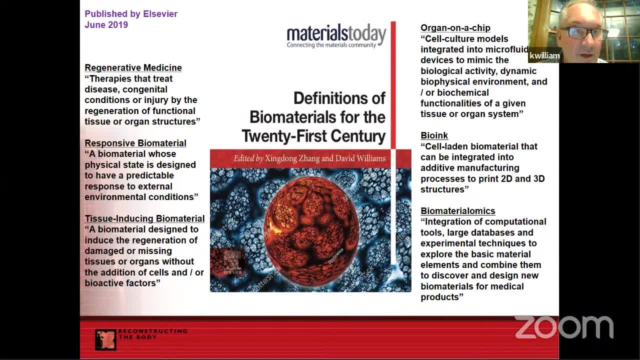 chemicals put together. A tissue-inducing biomaterial is a biomaterial designed to induce the regeneration of damaged or missing tissue organs, with the addition of cells and bioactive factors. Okay, organ-on-a-chip Cell culture models. This is really cool. This is. 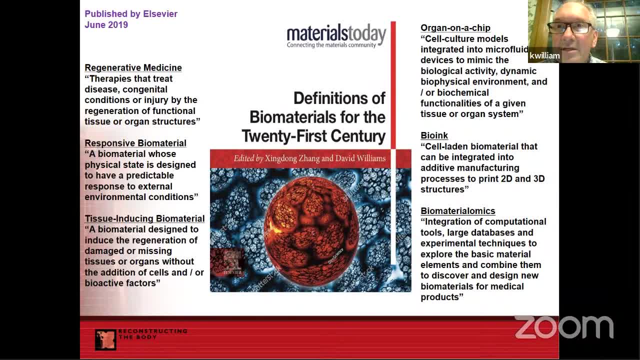 an up-and-coming technology. They're cell cultures integrated into a microfluidic device to mimic biological activity, dynamic biophysical environment and the ability to detect and detect and detect biochemical experiments and biochemical functions given tissue and organ system. These are three-dimensional and they consist of a variety of cells and they've actually 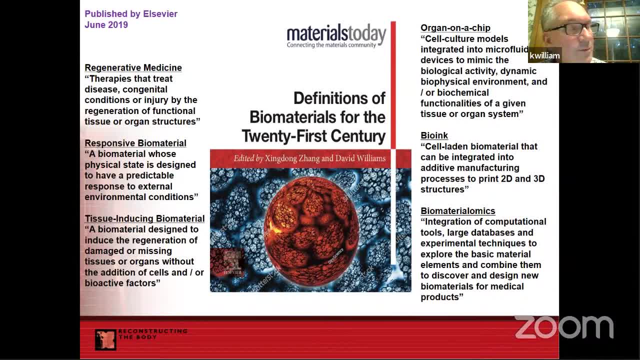 been shown to predict reactions to drugs very, very well, which might be a very important part of the development process for any kind of technology: Bio-ink, Cell-laden biomaterial that can be integrated into a tissue-inducing biomaterial that can be integrated into a tissue-inducing biomaterial that can be integrated into a tissue-inducing biomaterial that can be integrated. 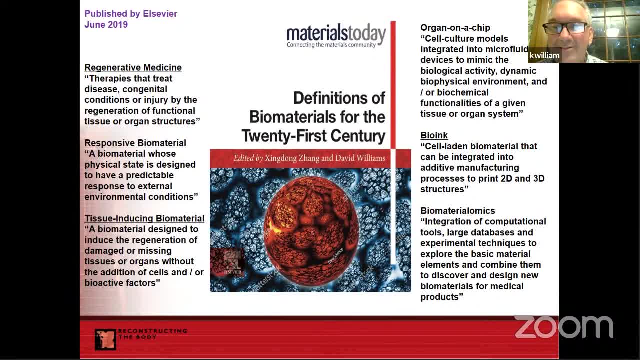 into additive manufacturing processes to print 2D and 3D structures. Excuse me, Biteriomelomics are the integration of computational tools, large databases and experimental techniques to explore the basic material elements and combine them to discover and design new biomaterials and medical products. 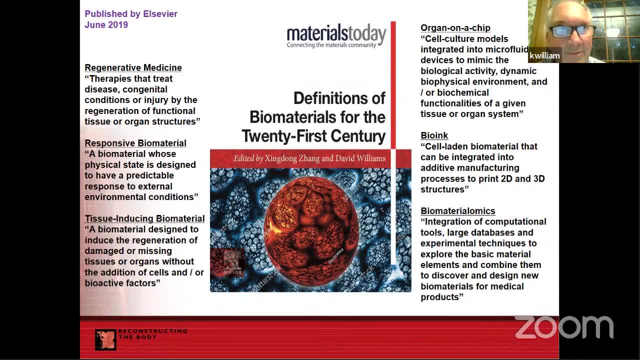 That would be, for instance, when I was talking to you about making those very complex multiple sandwiches of combinations of active support structure, all those different kind of chemicals that come together to make an ideal implant that will stay around for a while but will degrade. 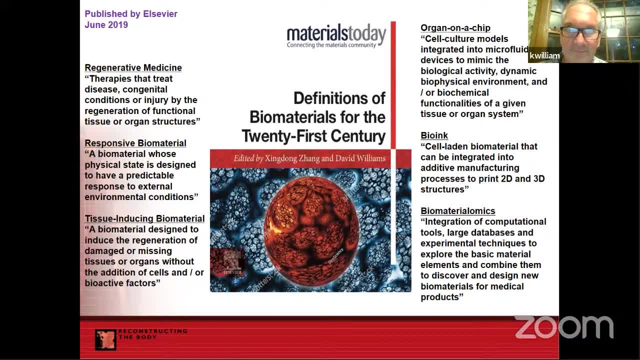 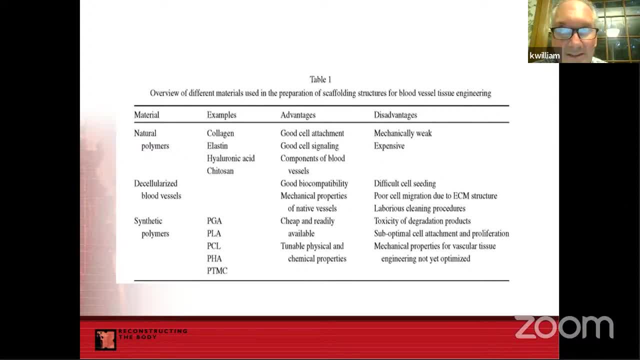 over time and provide the important support I suppose. So I've been talking in generalities but very, very important concepts there And I hope you got that. So let's just talk about blood vessel engineering. What materials have they used? 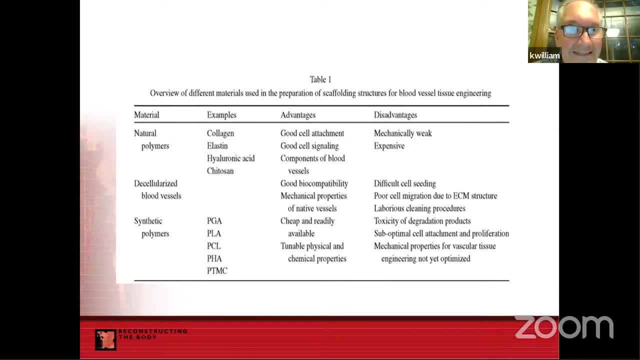 Natural polymers like collagen, elastin, hyaluronic acid, titicin. The advantages are good cell attachment, good cell signaling components of blood vessels, but they're mechanically weak and very expensive. Decellularized blood vessels- We've been doing that quite a bit. Good compatibility. 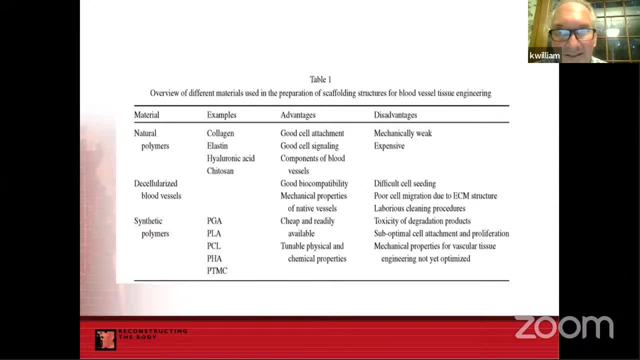 Mechanical properties of native vessels. Difficult cell seedings. A lot of times once you take the cells out of it it has to go through a decellularization product And sometimes it does not create that niche that cells like, So they don't go in and set up home and grow. 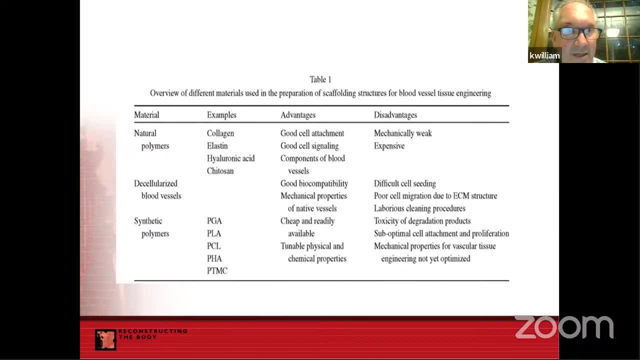 Poor cell migration due to the ECM structure. Synthetic polymers like PGA, PLA, PCL are cheap, ready, available, tunable. physical And chemical properties are important. You can make them kind of any size you want to. They can be toxic. Their mechanical properties for vascular tissue are not optimized yet. 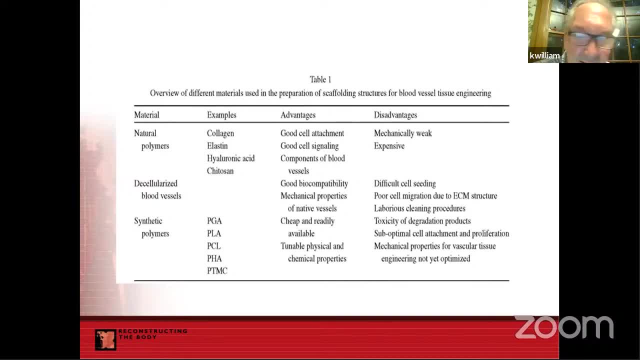 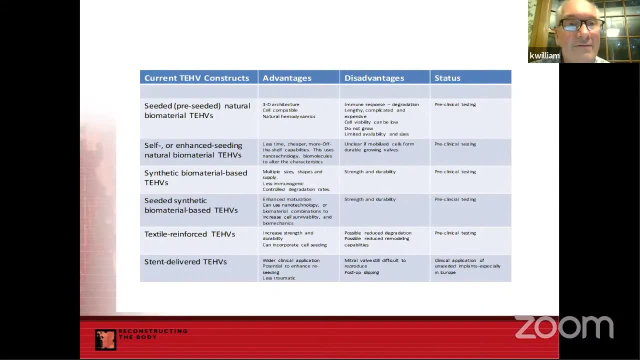 Suboptimal cell attachment and proliferation, at least so far, But they're getting better Now. current constructs for tissue engineered heart valves, Seeded or pre-seeded natural biomaterials. Advantages: are you got the 3D architecture there? Disadvantages: immune response. 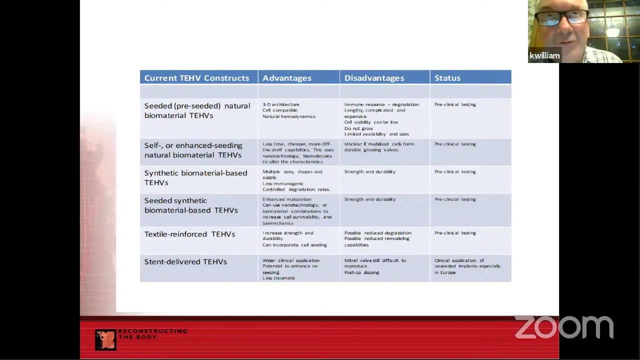 If you put in a decell valve into a child, chances are that decell heart valve is going to have to be replaced three, four times. Cannot grow. It is going to slowly degrade And is now being tested. Sell for enhanced seeding natural biomaterials. Less time Uses nanotechnology and biomaterials. 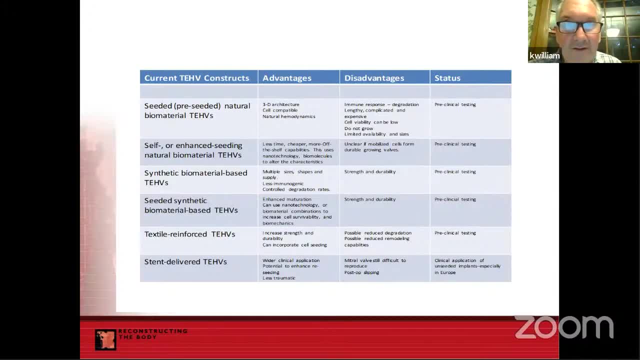 Biomechanical to alter the characteristics Unclear if mobilized cells form durable growing valves. Preclinical testing: We've actually done a little bit of work with that, where we've used decell valves And conjugate them with CD133, which attracts endothelial progenitor cells. 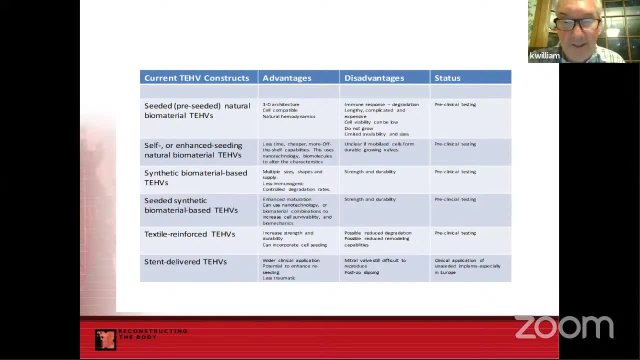 And conjugate it on to the decell valve, Put it in Rebuke sheep and the things will resell your rice on its own. You don't have to add cells, You don't have to do anything. It will resell your rice on its own and that is under further testing right. 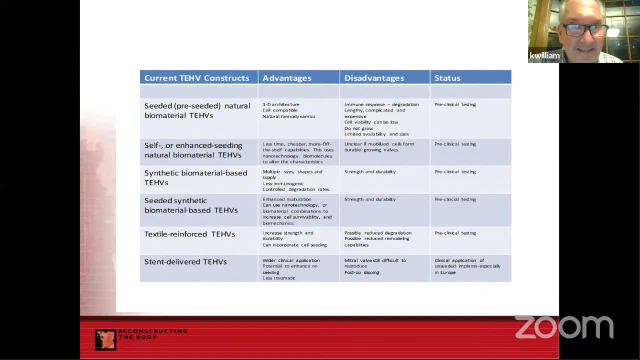 now You can use seeded synthetic biomaterials, textile-reinforced heart valves and stent-delivered heart valves. Now that's really cool, because many countries do not have the ability to do open-heart surgery. A lot of people don't have the money and the country don't have it. 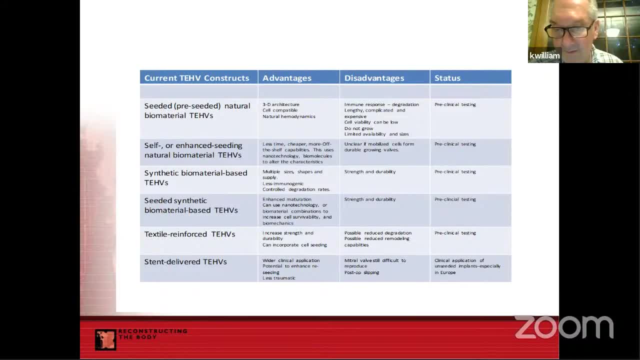 the ability. They don't have that many hospitals and that many trained open-heart surgeons. so they've developed stent-delivered tissue-engineered heart valves. They go in through the groin and into the artery and they can go up and plant them right. 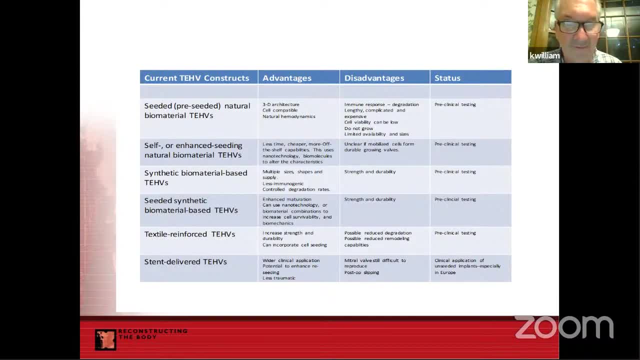 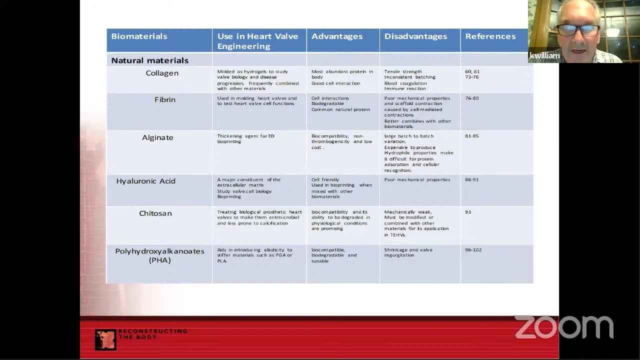 in the aortic position Or the AV valve position, and that is a lot cheaper, can be done in most hospitals, and so that is very good. Let me talk a little bit more about some of the biomaterials. Collagen is used quite a bit, actually quite a bit. Most abundant protein in the body. 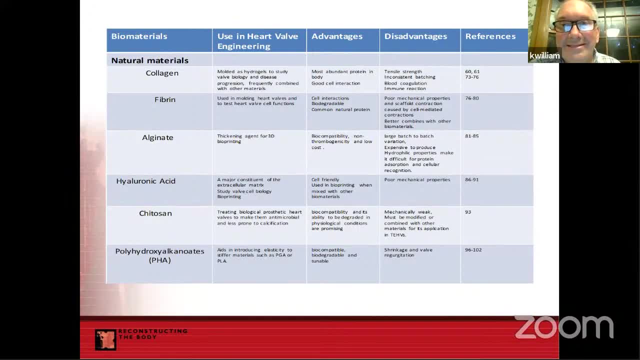 good cell interaction. tensile strength is consistent, but it is going to. it's going to degrade Vibrin, biodegradable, common natural product but poor mechanical properties. It's very weak Alginate thickening agent. for 3D bioprinting It seems to be a good. 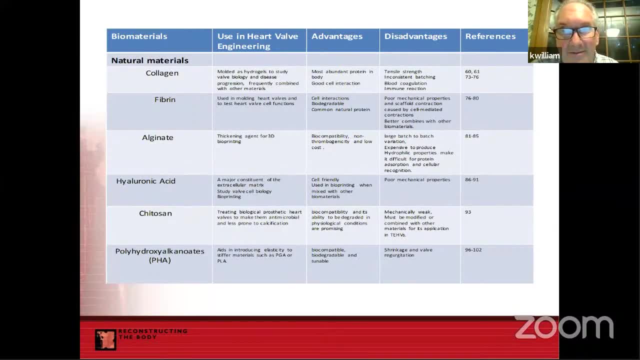 but there's large batch-to-batch variation, expensive to produce, and so that kind of takes away some of the advantages. Polyuronic acid, poor mechanical properties, cell-friendly, using bioprinting, Right knee and they have a new injection they can use to put right into your knee. 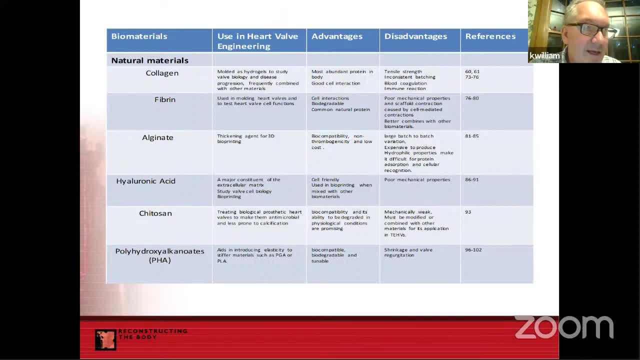 which is basically hyaluronic acid, which forms has your knee. try to regenerate itself. Hopefully it'll work. Chitosan biocompatibility is okay. It's mechanically weak: PHA shrinkage and valve regurgitation can be a problem. So, as you can see, 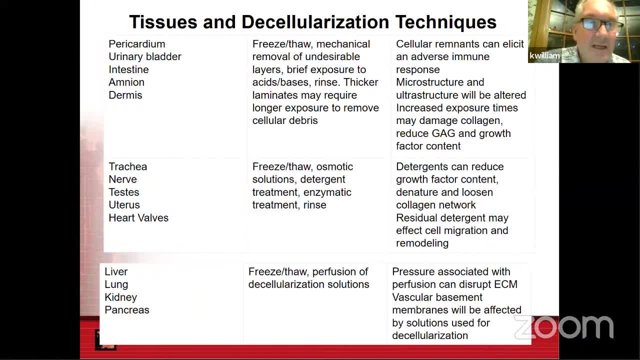 there are a variety of things. they can use. nothing perfect yet. So if you go the route of getting a valve, or you get something and you want to get rid of the cells, and let's say you don't want to make a biomaterial, you just want to use the shape that's already there, you got to get. 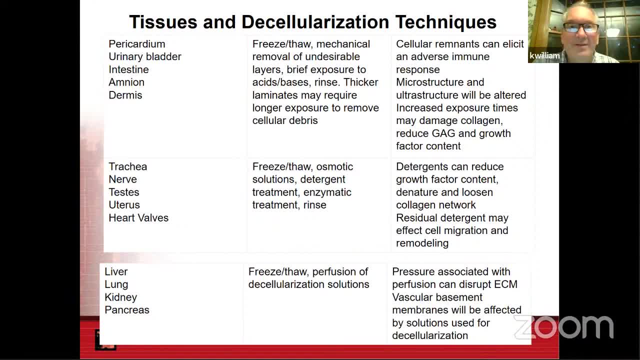 rid of the cells. And there are various ways to get rid of the cells: with series of detergents, freeze, thaw on osmotic solutions which will blow up the cells or shrink them. detergents, enzymatic treatments, various things you can use. Nothing is perfect, Most of the time. 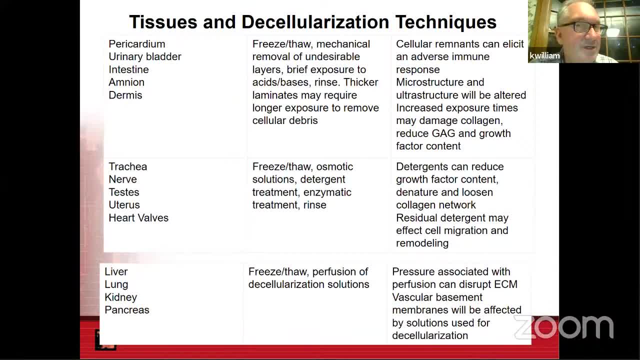 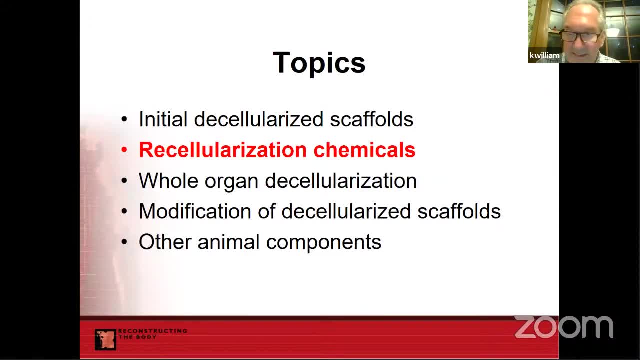 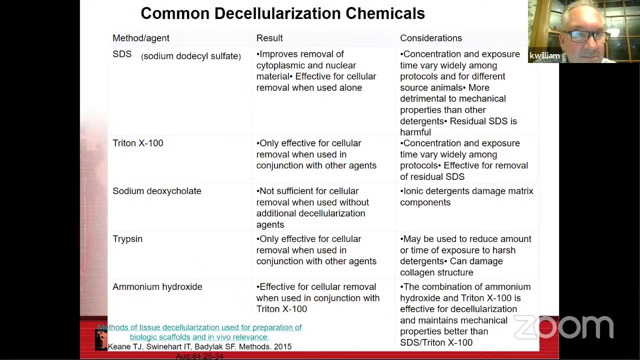 it leaves some residue and causes the existing collagen to cross-link, which reduces the ability of it to expand. Okay, resellularization chemicals. These are some of the chemicals they use: SDS, Triton, sodium, deoxycholate, trypsin, ammonium hydroxide or some. 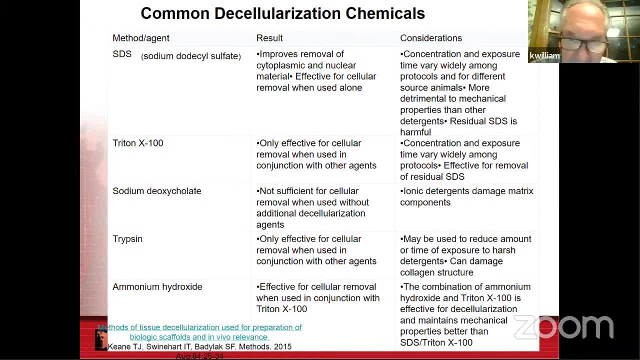 compounds, And then there's a lot of other chemicals that they use. So, for example, they all have their advantages, They all have their disadvantages. Nothing is perfect. Again, I think Irma can give you a copy of these slides so you can read them more carefully. 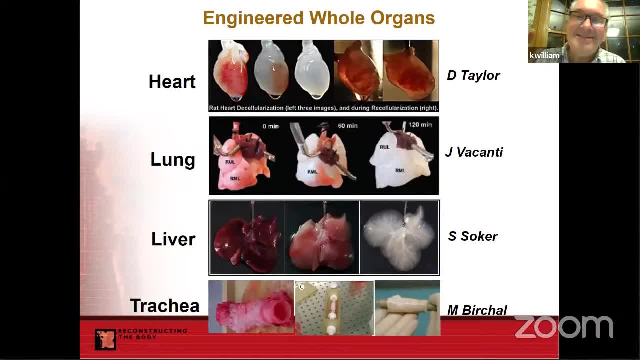 Okay, whole organ desellularization. This is really cool. Instead of going with part of the organ, let's just desellularize the whole organ And then try to if it has bad cells or it has some data. let's just desellularize the whole organ And then try to resell if it has bad cells or it has some data. 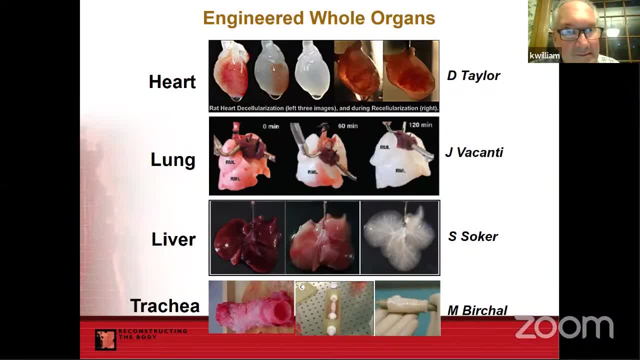 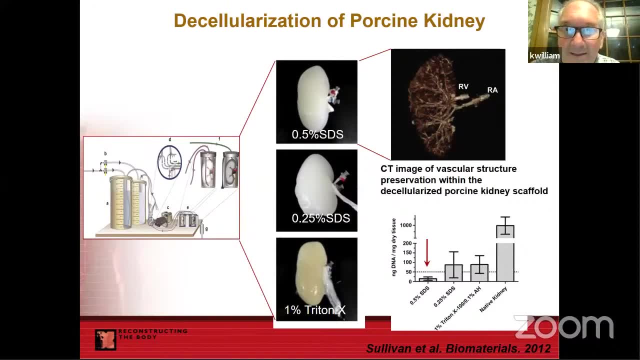 if it has damaged cells. So they've been doing this in the heart, the lung, the liver, the trachea, taking the cells out And then trying to put them back in. Here's one where they have taken all the. 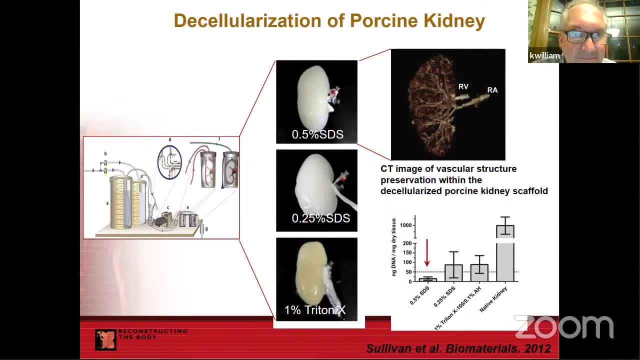 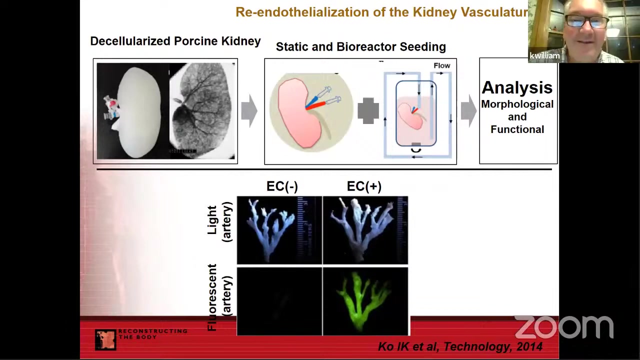 cells out of a kidney. This is in a rat And it's very, very still very, very micro-organized. right now You can't get real big arteries or big. excuse me, you can see that you take away the cells, you leave the vasculature which lets you there. once you get rid of the cells, maybe you can. 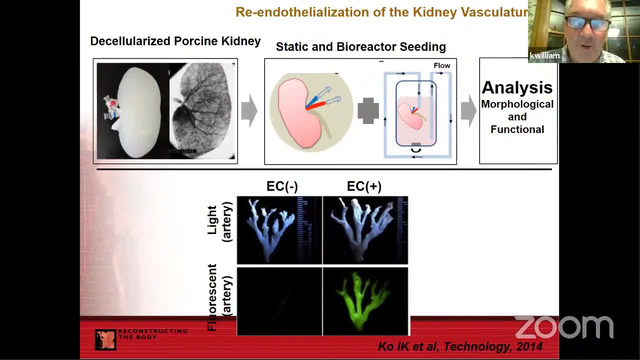 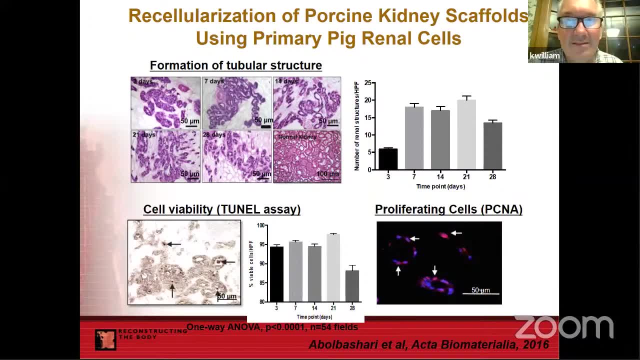 put bad cells. you can regrow that by putting cells back into the vasculature and, lo and behold, it seems to work. um. this is in renal cells putting- uh, they re, excuse me, decelerize the kidney and then put them back in, um healthy cells back in and we're able basically to form um kidney structures. 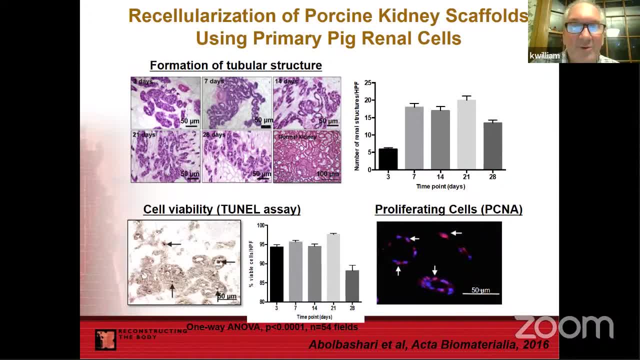 by infusing normal cells into a decelerized uh kidney. that way you don't have to go and try to make a kidney structure. you don't have to worry about putting together complex biomaterial. you can get rid of the sick cells and put in healthy cells. there's some advantages to that. we've been 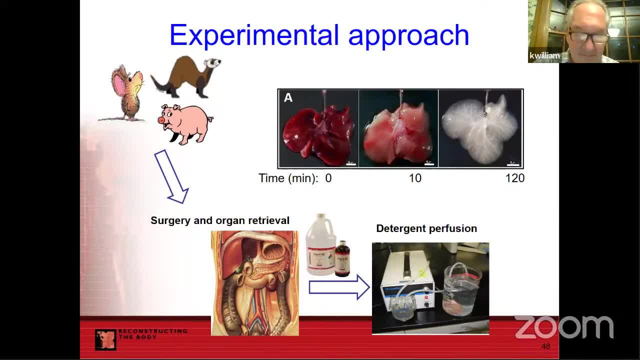 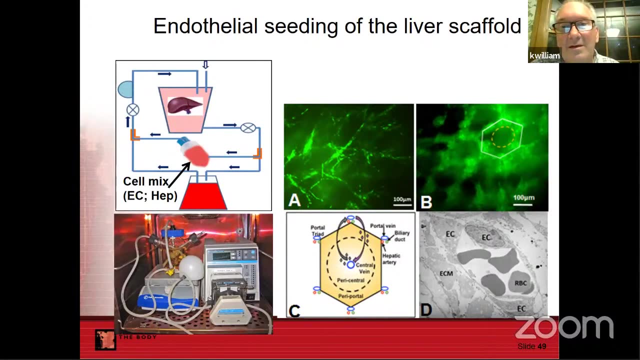 doing um liver studies where we slowly a taking away the cells. you can see it turns red to basically translucent as we get rid of the cells and then re-put in endothelial cells and you can see over there in the uh right the green fluorescence of uh putting in endothelial cells which light up. 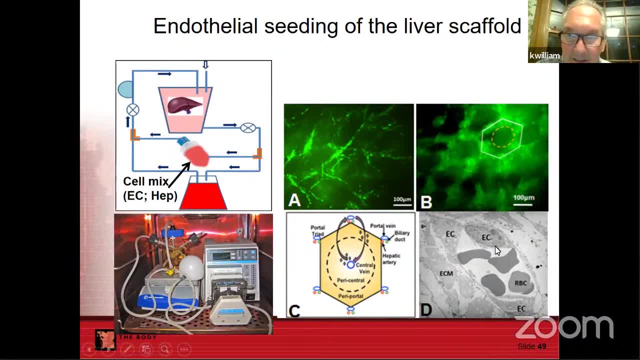 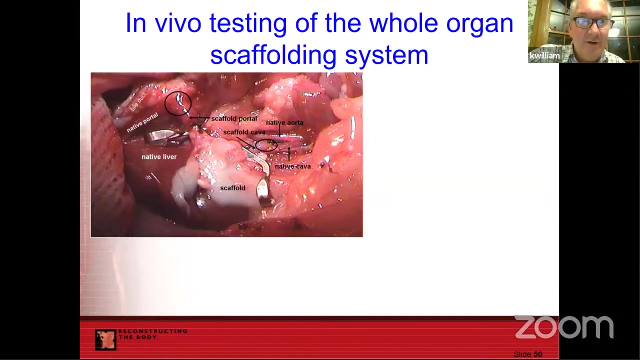 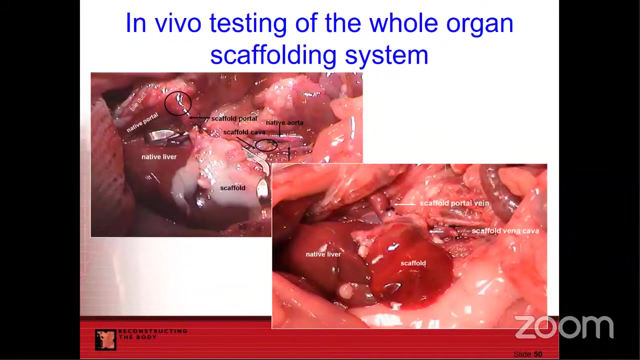 the vasculature and form um. they form uh vessels. once you get the vessels in there, you have a chance of making that tissue healthy. okay, i'm back. hopefully here we've done uh, where we we have native liver put in a decelularized scaffold- you can see scaffold there- and then we infuse cells. let it go for a long time and you 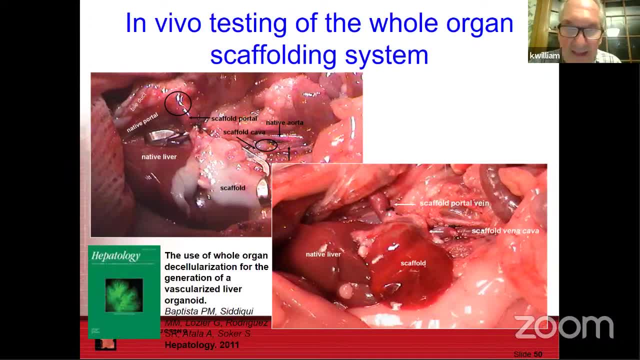 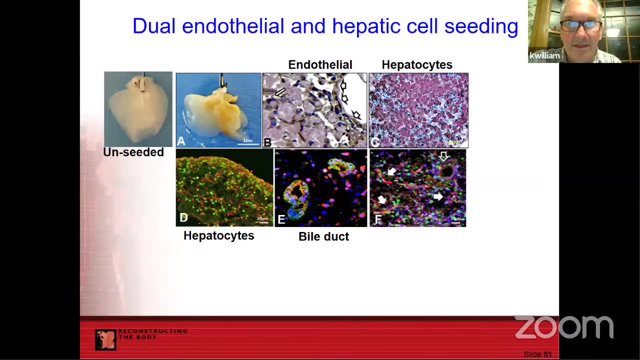 can see that scaffold is looking pretty much like a native liver and it is acting like a normal liver. It produces hepatocytes, bile ducts, endothelial cells and creates fairly normal albumin secretion and urea secretion, which is very typical of normal liver. 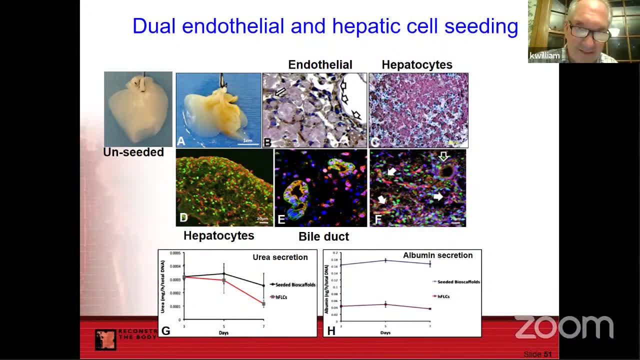 So this is another option for a biomaterial: Just take the cells out of a sick or even a cadaver, like a kidney or a liver. get rid of the cells that would cause an immune response and put it in a person's own cells. 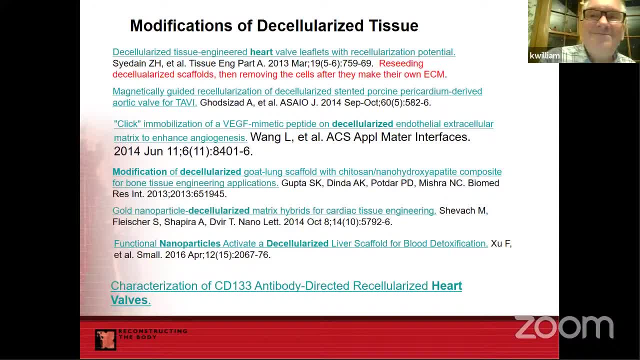 Now modifications of normal cells, So decellularized heart valve leaflets with recellularization potential. We've done that with the CD133.. They've used magnetically guided rebase recellularization of decellularized stented porcine pericardium-derived aortic valves. 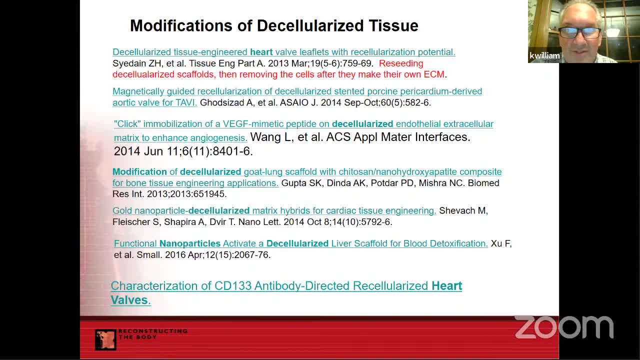 Modification of the decellularized goat lung scaffold with chitosan and nanohydroxyapatite composite for bone engineering applications. So you can see. what they're doing here is they are using decellularized tissue as their biomaterial and then trying to activate them to regrow. 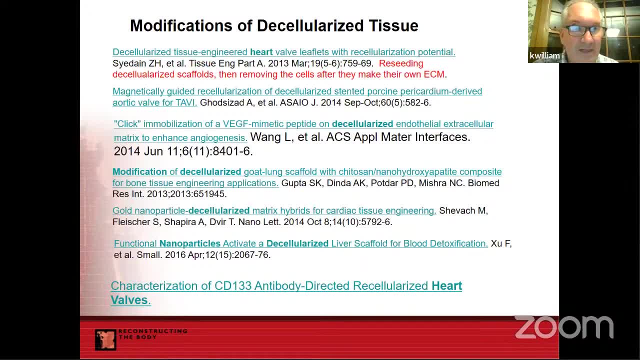 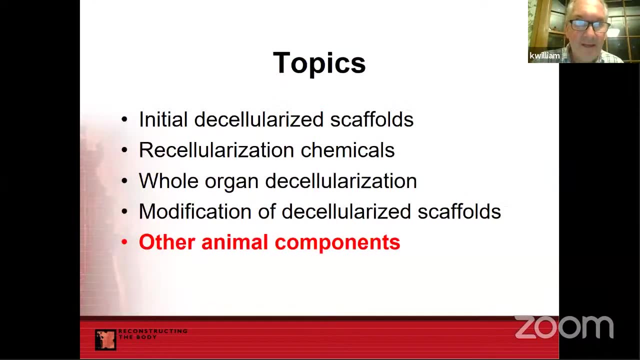 And they do that with nanoparticles. they can do that with a variety of other biomaterials like chitosan. They can use growth factors like VEGF- We've used CD133 antibody to do that- And other animal components. This is where I want to leave you. 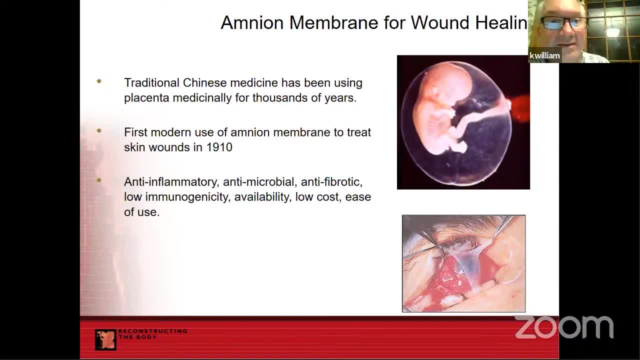 Traditional Chinese medicine's been using placenta medicinally for thousands of years. The first modern use of amniotic membrane was to treat skin wounds in 1910, long time ago. Anti-inflammatory, antimicrobial, antifibrotic, low immunogenicity because it is from the placenta. 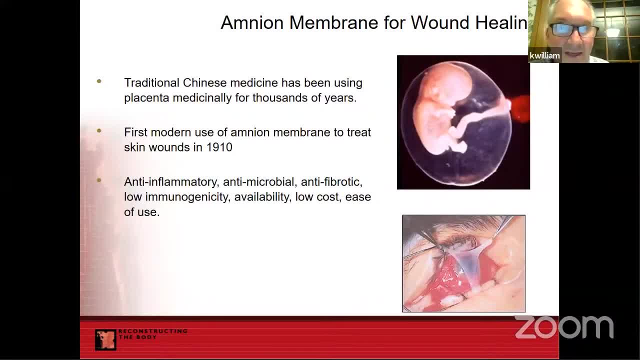 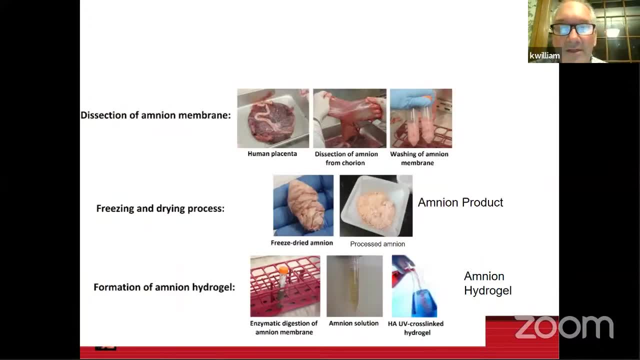 and hasn't seen a lot of immune cells, A lot of available, low cost ease of use. So what they've done, what we've done here at Dundee Affirm, is: dissection of an amniotic membrane, make a product. 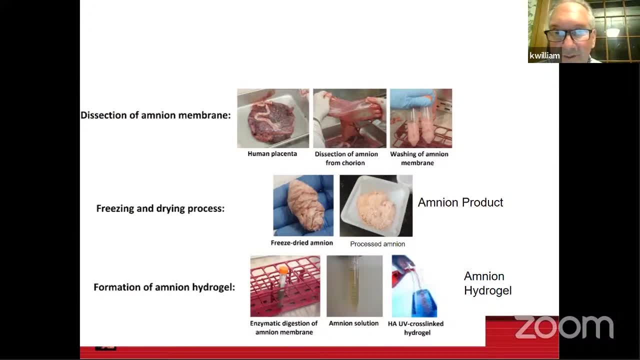 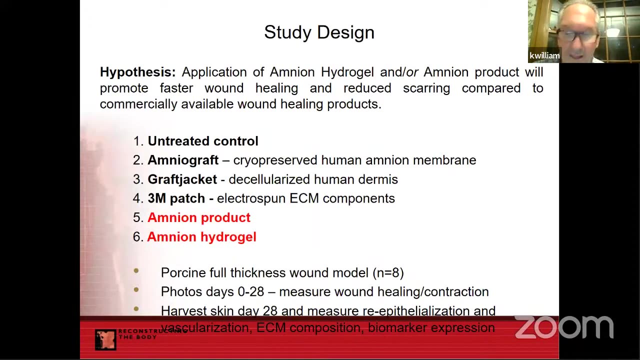 basically freeze, dry it and make it into a hydrogel or just an amnion. So that's your biomaterial, That's your. so it's amnion hydrogel or an amnion product and used it in here. okay, used it to try to heal. 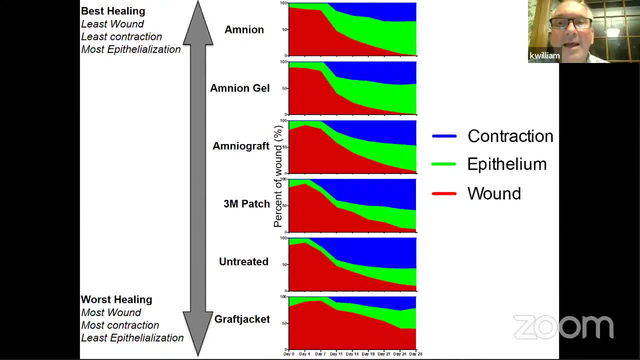 skin lesions that we've created in pigs and to look at the healing of these skin lesions. And these are just some pictures and images of what we have with the amniotic gel, the amniograph, which is just the amniotic tissue- 3M patch. 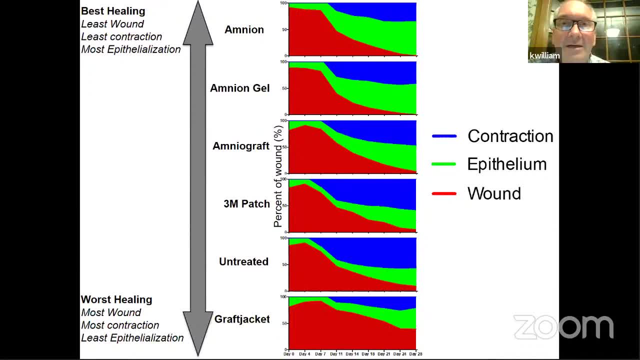 which is kind of standard that you put on wounds And what you can see is the amniotic gel or the amniotic graph do a very good job of reducing contraction while forming epithelium, but reducing the size of the wound a lot better. 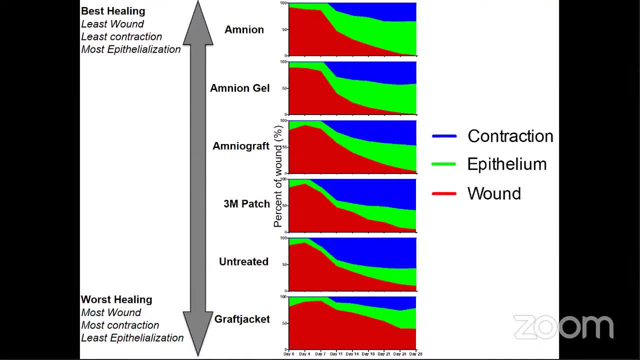 than a lot of the things that are on the market right now: A graph jackets, 3M patches do not do a very good job. So this is the using a biomaterial that is from the amniotic membrane. So taking a natural amniotic membrane. 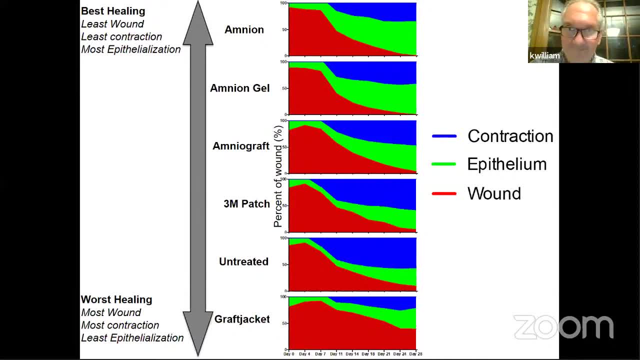 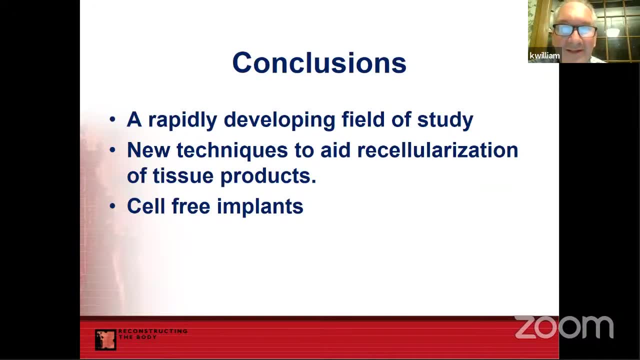 and there's lots of those, and using that. So conclusions: well, it's a rapidly developing field to study, that's for sure. New techniques to aid re-cellularization of tissue products, cell-free implants, complicated, very sophisticated bio implants made of a variety of biopolymers. 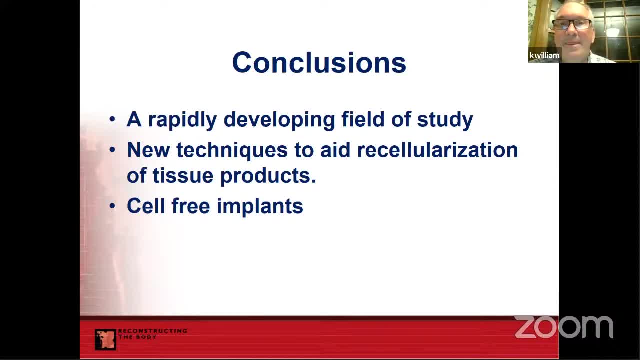 metals, ceramics, and we're just beginning to realize that if we're going to do this, we have to produce a very consistent product that has the strength that it needs to the biocompatibility that it needs to Be able to crosstalk with the cells in the body. 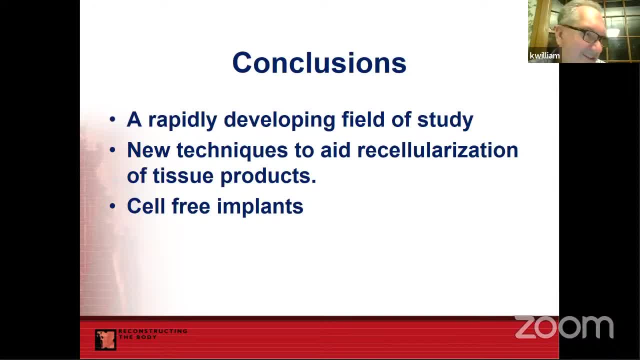 Degrade at a rate that you want it to degrade, Get replaced with natural functional tissue. That is a tall order. That is a tall order. That is a hard thing to do, but that's where we are right now and that's what we're realizing. we need to do So. with that, I will leave you. 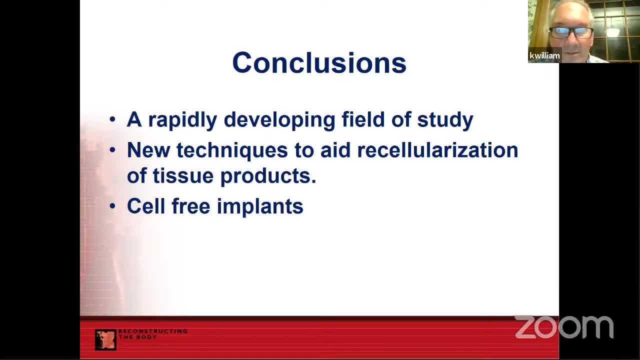 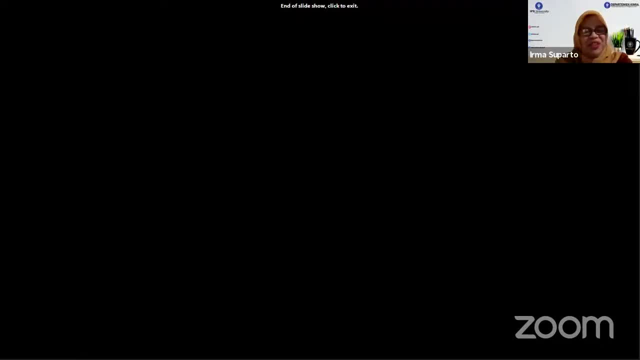 Um, and certainly if you have any questions I'll try to answer them, but remember I got to see him, Thank you. Thank you for coding. Wow, that's a lot to take, but I'm so happy that the student already had some classes of some of the topics about your biomaterials and about concept of compatibility, so I I bet they can interact. 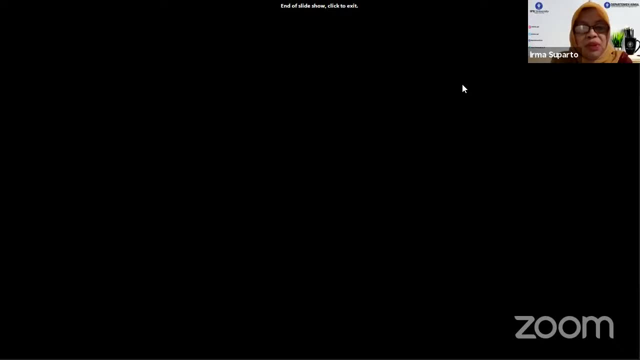 And I know you have several questions already on the chats. Would you like me to read, or would you like to for them to directly ask question? Please, If you could, if you could get their questions and then ask me. Okay, I will read it to you. So, from Dr Nafian Darmawan, I have two questions. One you mentioned in your talk: the template of biomaterial is critical for biomaterial cell interaction. 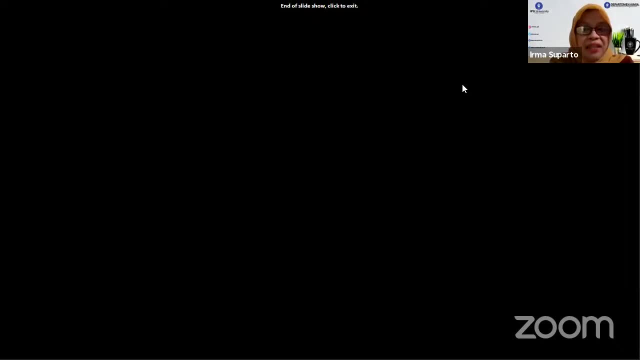 Is there any general guidance for designing the ideal template, such as porosity or large surface area? Yes, Yeah, you know. if you look in the literature, people use a variety of porosities is a variety of biomaterials. I just wanted to point out to you what they should do. 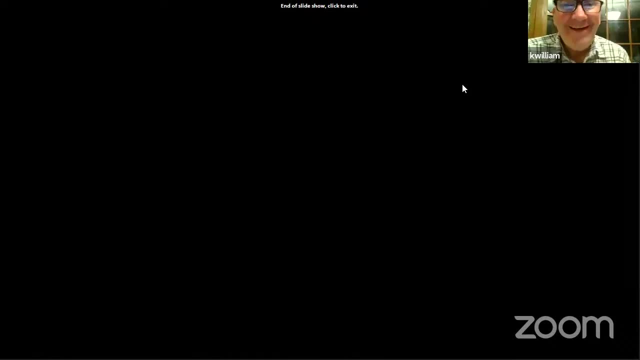 And you gotta go searching for something that will do it. There are thousands of publications out there, people using various things. there's some of the nanoparticles going on. right now. They're making biomaterials that contain nanoparticles that then direct the cells are very, very interesting. 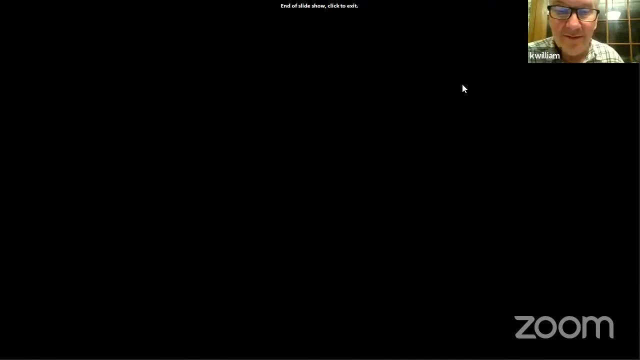 I'm not going to say one is better than the other, but porosity is an important issue. it has to be big enough to let the cells in, but not so big that they go in and then come right back out. You want them to adhere, you want them to be happy in there and you want them to start producing the biomolecules. 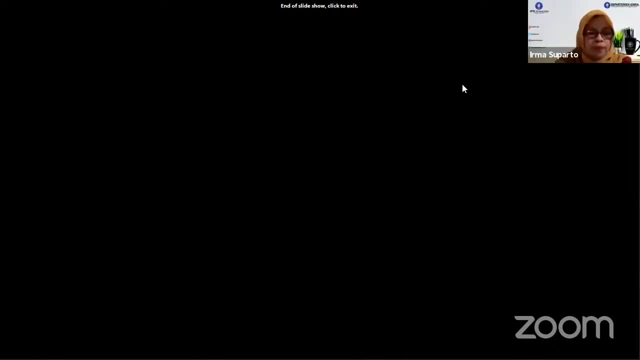 They're supposed to. I don't have you know what the ideal pore size or the ideal biomaterial is for sure, So it depends also on what you're going to design. right, Absolutely. It's very case by case, almost Right for a bone. you want it to get hard. Right, Yeah, I mean you want it to get hard, Some of the things you might want to keep elastic and with a lot of compliance, But a bone you want it to basically calcify in and become a bone that can support weight. So it really depends on the tissue that you're trying to regenerate. 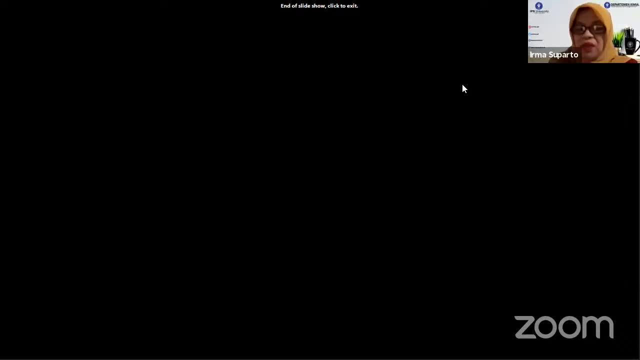 Okay, The second question from Dr Nafian also: is the decellularized method practical for real world use? You know, how long does it take to get a full organ, Because I was thinking about that too. If you take it from a cadaver and then 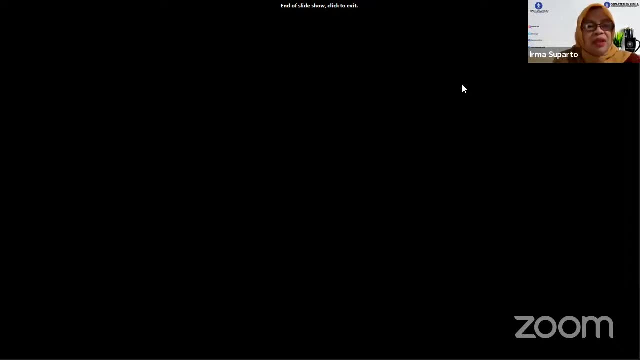 Have how. what do you think? Yeah, I think. Well, to get. there's about a thousand different decellularization techniques that people say is the right one to use. That's for sure, And it takes a long time. 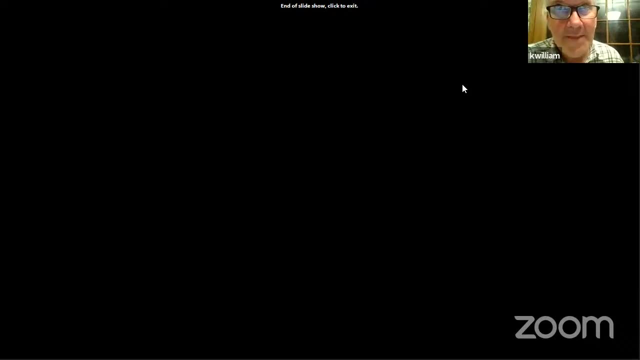 In it There there's no doubt that there It creates some change in the tissue that you're decellularizing. It's expensive, For instance, a cadaver heart valve That's been decellularized. They have these now that you can put it. 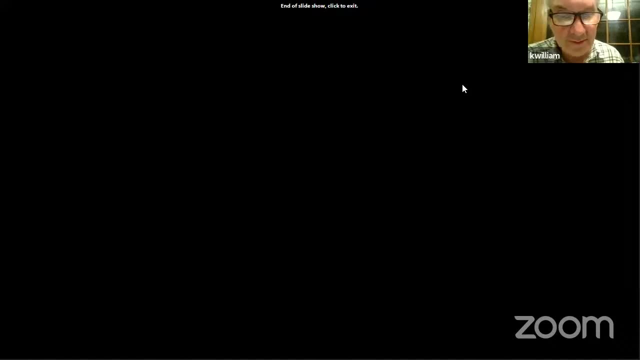 Well, pig valves and and but a human valve. If you get a decellularized human valve That's been decellularized the right way And according to the FDA and all that, You can get a decellularized human valve. That's been decellularized And that can cost upwards of $20,000.. Just for the One valve, One valve. And so it's very, very expensive to do that. That is why- And the other thing is- is it's hard? 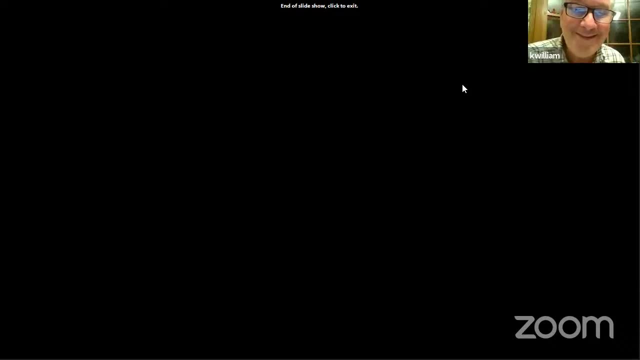 If you're trying to put a valve in a child, Most of the valves out there that are decellularized and come from adults. Right, You get old and you take it from somebody that's that's elderly and died, So the valve is way too big. 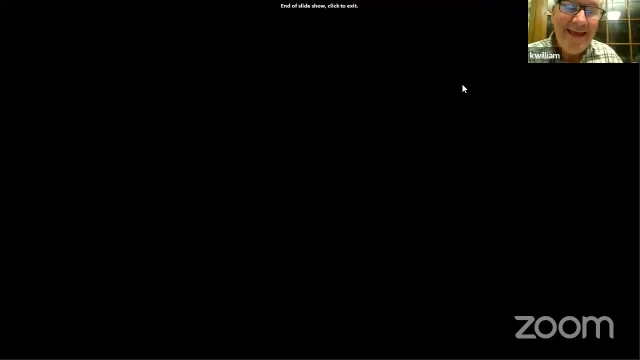 That's why they like the bio material that they can make and they could, And to make it in the size it's supposed to be, I think decellularized Tissues. I sort of get the feeling that we've seen the best of them. 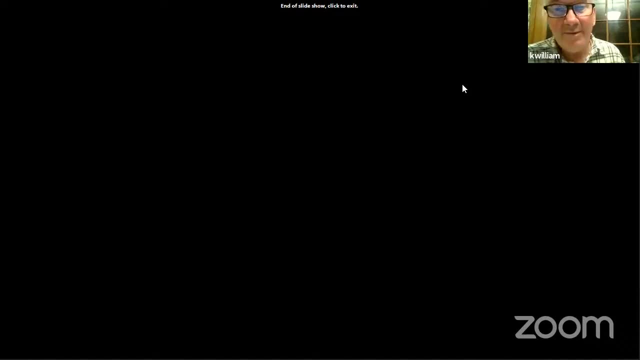 And they might be going away, But not until we get better with our bio materials. I think it's Not going to last that much longer, but we have to come up, Thank you, Thank you. That was the last question For Mr. 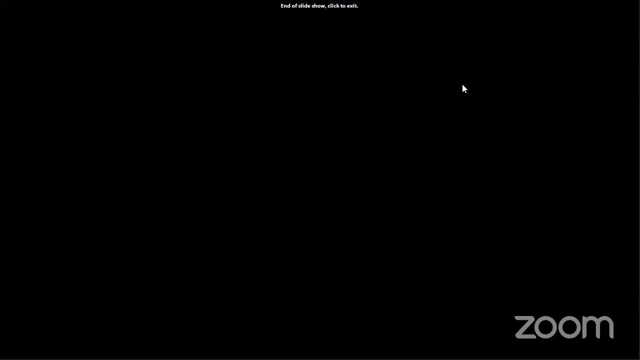 Novi. But yeah, Thank you, Professor Kelly. Okay, Thank you. So well, I was thinking also. the same question is, Dr, I cannot imagine You have too late, It's more Cheaper to just make one ride. 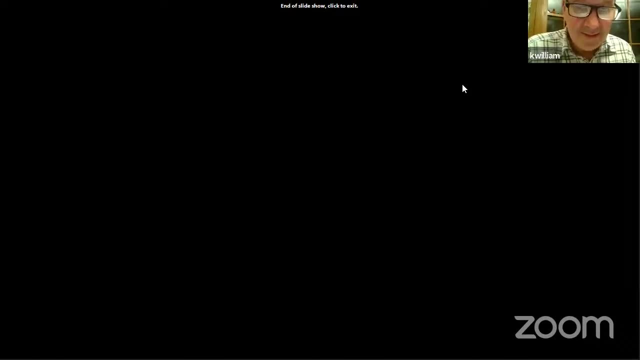 Then Well, it's certainly cheaper to do it, But again, you also countries out there that do not have advanced biomaterial science and able to make something like this. The trick will be to make them and have them been popular enough that the 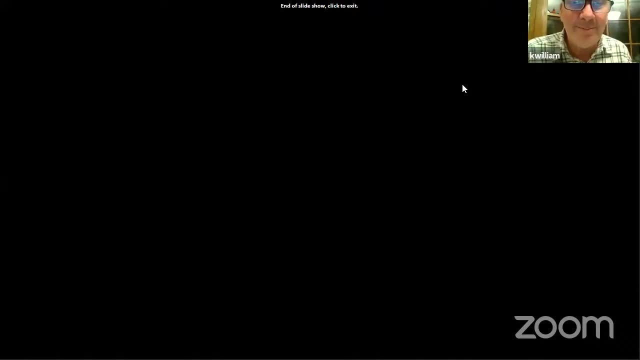 cost will go down. Kind of like those computers we used to buy that well, the handheld computers that could add, subtract, multiply and divide, maybe do a cosine and do some square roots, for it used to be $300, and now they give them away. So hopefully, the more you use them, 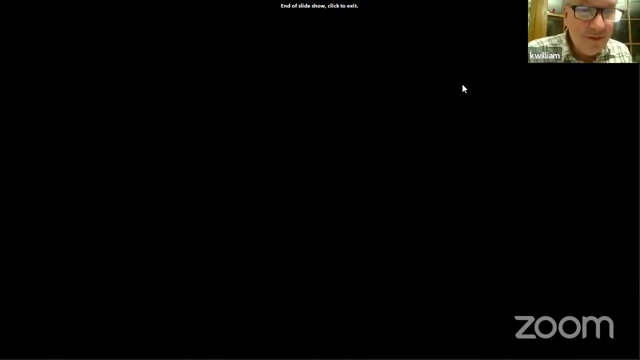 the better they are. The price will go down over time, like everything. when you and your color TVs, The plasma screen TVs, used to be $7,000, $8,000 a piece, and they're $100,000, $200,000,. $300,000 now. It'll get cheaper, but not for a while. There'll still be a room for decelerized tissue. I like the idea of trying to get some tissue to repair itself in vivo. In other words, we're doing some studies with people with a pulmonary disease. They have a lot of fibrosis. 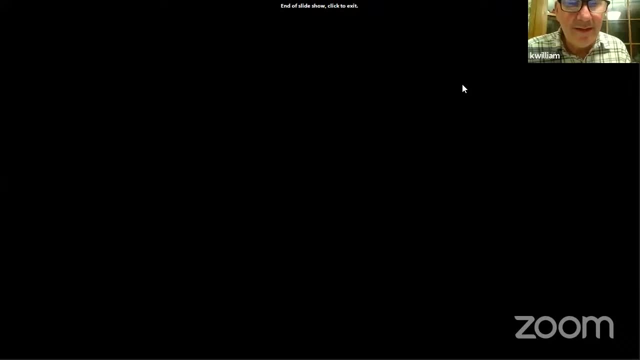 and we're trying to come up with things we can put in to get that lung to repair itself in situ. You don't have to put in anything. You're trying to reprogram that tissue. I think that's cheaper because a lot of these molecules aren't that expensive, For instance, 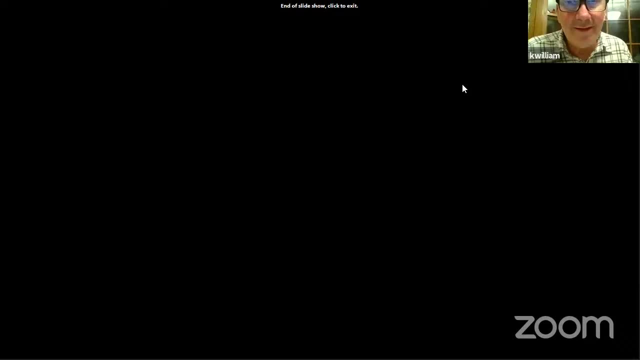 we use, as you know, CXCL12 quite a bit and it's not that expensive to use this stuff And I'm kind of hoping that will tide us over until the biomaterials get up to you know speed of what they need to be. 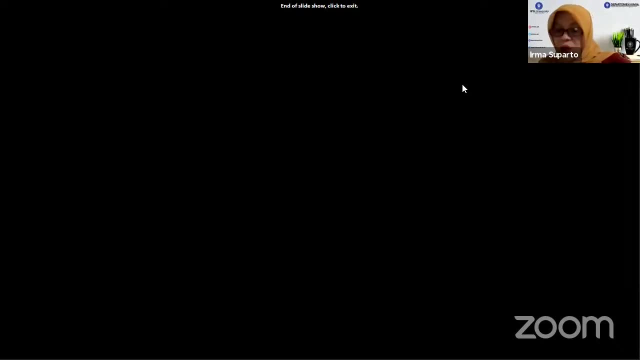 Thank you, Prof Cody. We have four questions waiting for you, So from Hari Noviadi, thank you for the nice presentation. I have a question: What are the challenges in developing biomaterials from tissue engineering, and how long can these biomaterials be used as 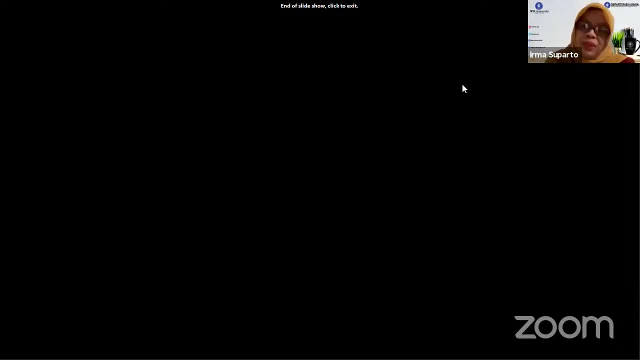 implants based on biostability and biocompatibility data. It's a general question. Where we are now is- and I think David Williams would agree with me- is: I think we finally know what we need to have a biomaterial do, And I think that's very important that you know. 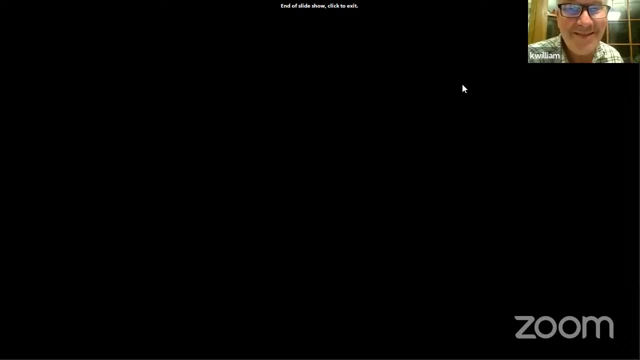 we finally know what we need to know, And that's the beginning. I think we finally realized we got a long way to go, but that's the first part of true knowledge- is you realize where you need to go, And that's why I wanted to do this. 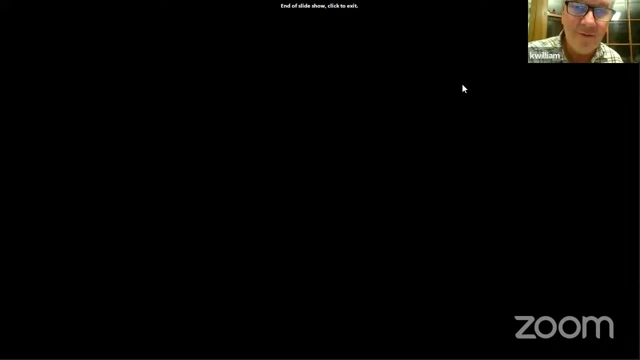 Thank you, Prof Cody. Thank you so much for your presentation to show basically what it is we need to know to have a biomaterial that acts that way. Where are we? We're working on it as fast as we can but, like anything that you produce, you know you're still years away from using these. 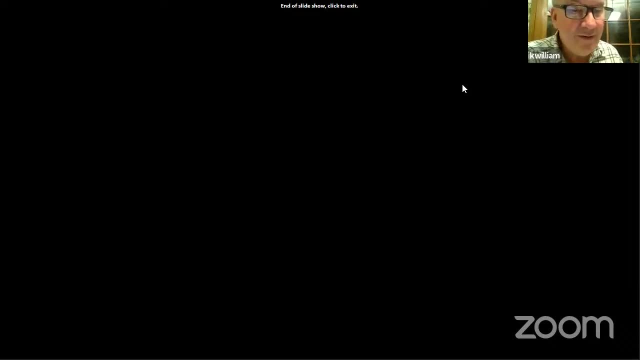 widespread clinically, but it depends what it is. We already have some biomaterials we're using in clinical studies. right now They're more simple. right now They're a lot simpler. You have a lot of decellularized bladders, penile implants, vaginal tissue. As you know, we did a 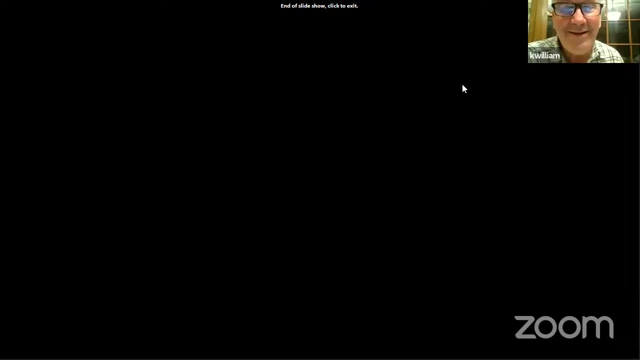 study in cats for kidney disease and that is in clinical study right now. But the actual biomaterials. I think people are finally getting on board with what needs to be done and that will take a while. Yeah, it takes time. Yes, it does. 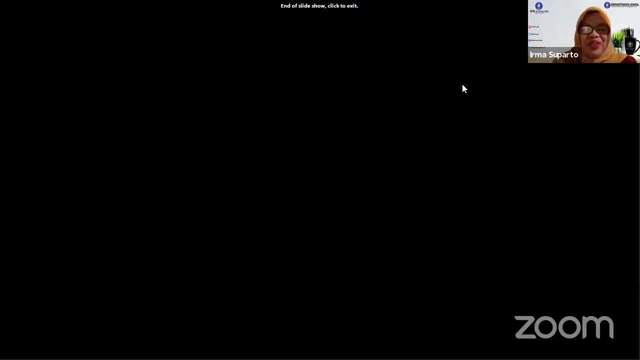 So lots of financial, what's called it financial aid. Well, you know, startup is always expensive And, as you know, I've come to Indonesia and tried to encourage some work done with using biomolecules and using that to help regenerate tissues. 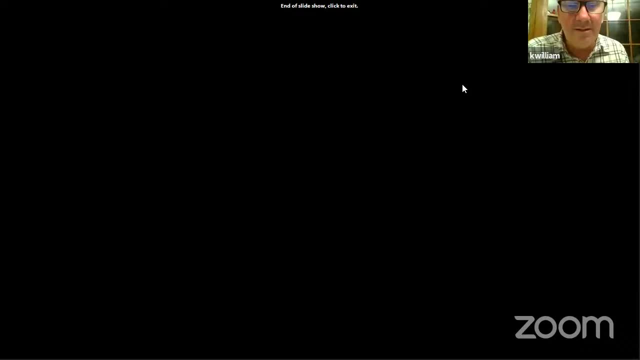 And the biomaterials will come along later. But, as you said, there's a lot of startup money to get that done. The inkjet printers and all that are expensive And it's not impossible, but they're expensive. Yes, Okay, Thank you From Adi Sifriadi. Professor Kaudi, could you please explain? 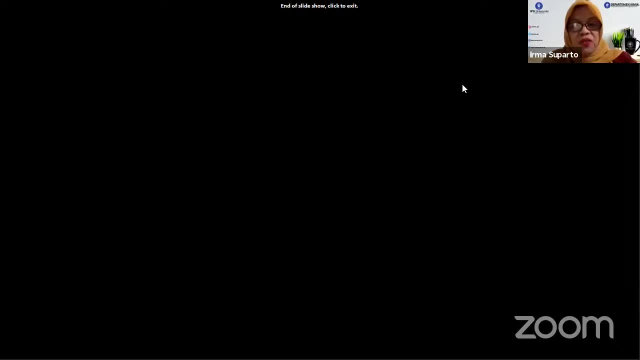 about material characteristics for tissue engineering application, especially based on molecular interaction with the compound. Yes, very, very important, Very important That material you put in. let's say you start with a ceramic or you start with something like that. you know pretty soon you're going to want that. 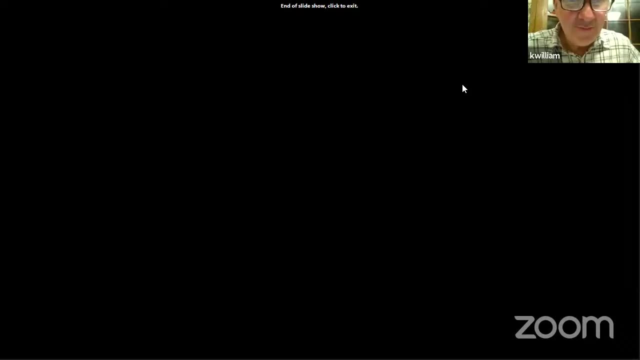 to start interacting with the body, And that's why I showed that one slide, the complicated slide. It's got to know where it is, then it's got to start responding to the pressures that it's under and then it has to start creating. 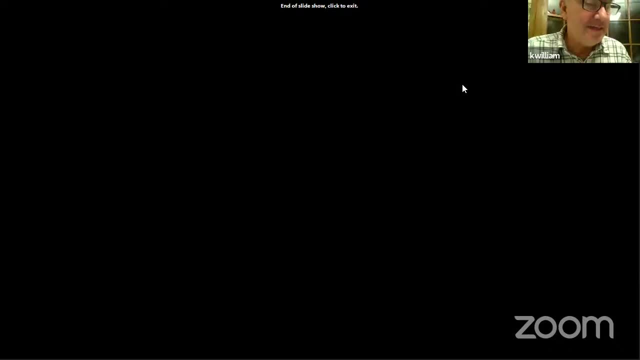 That cell-to-cell interaction and cross-talk. that needs to happen. That is where the small molecules come in. It is where some of the nanoparticle stuff comes in, And you know, there's even stuff where they've created a biomaterial just by the way that it's. 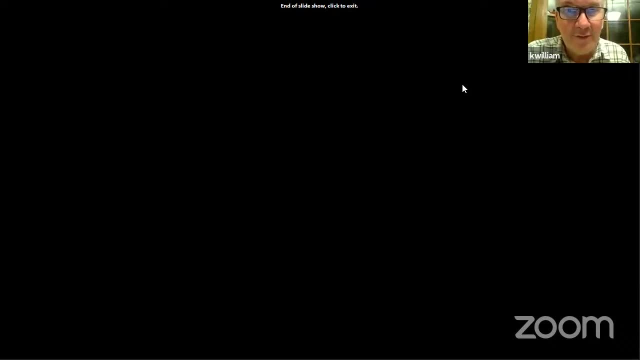 made starts the cells in there and they start cross-talking. They don't add anything to it. It's a very simple, very simple Design and they put it there and the cells start talking to each other. But you know, for heart valve it's very important that the lumen cells talk to the cells inside. 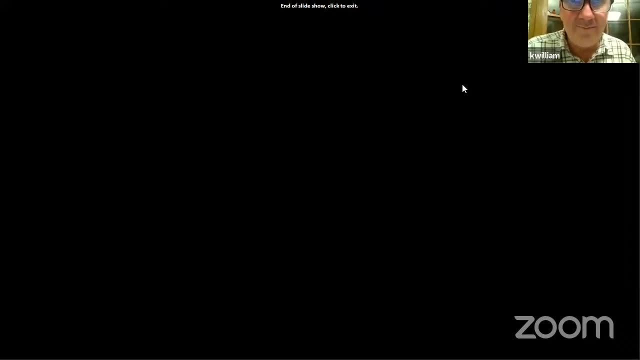 the leaflets for them to work. If they don't, it'll just scar in and you end up with a scar. So they must talk to each other. Very important, Very important, And therefore you have to have a really good idea, molecularly, of what you're trying to do. 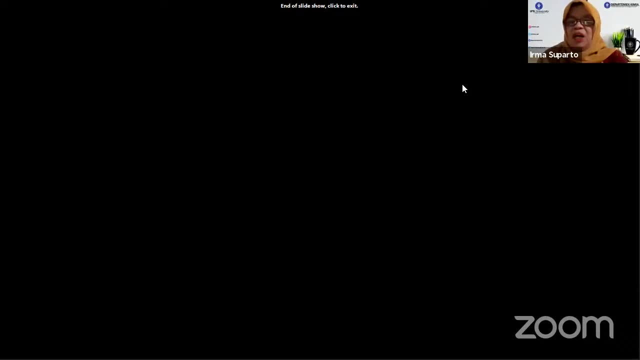 to accomplish. thank you, uh. what interesting question about what is the prospect of to change tissue of hair skin. you know we have problems with our hair, so what do you think about that? it's from uh, okay, this is to grow hair, is it? uh, is that what you mean? 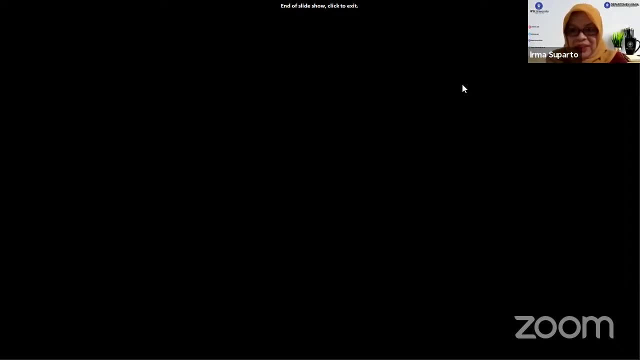 okay, probably, cody. oh okay, well, first of all, you're gonna have to get it lined behind me and but yes, you know, we have um a study ongoing right now. dr atala has a study going on right now with bioengineered uh, basically hair plugs, uh, that they're putting in right now. that, uh, in fact. 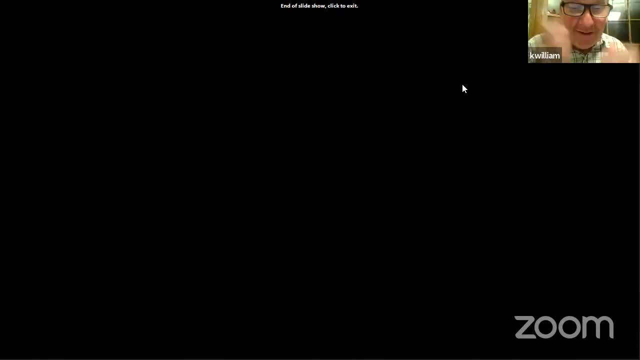 you know, i'm not sure if you can see it, but i'm not sure if you can see it, but i'm not sure if i'm on the animal care and use committee. we just approved it for uh, so they can go ahead and this is, uh, god, what an animal model. you know there's a. yeah, this tumptail macaque gets normal male. 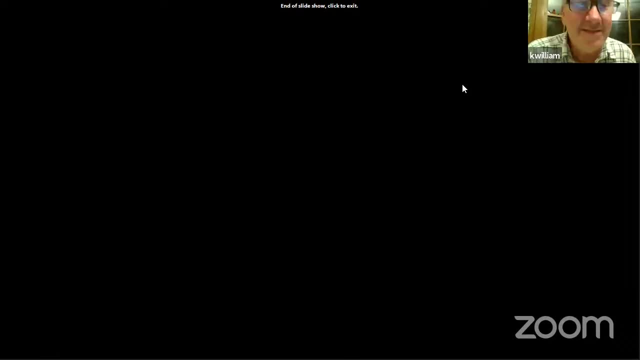 pulp, male pattern baldness. but this is, this is a nude, some kind of nude mouse or rat- that they're going to do this and put in um, basically bioengineered, um, uh, parallel hair follicles and try to get those hair follicles to go. oh, that's a good thing, okay, so i say they're. 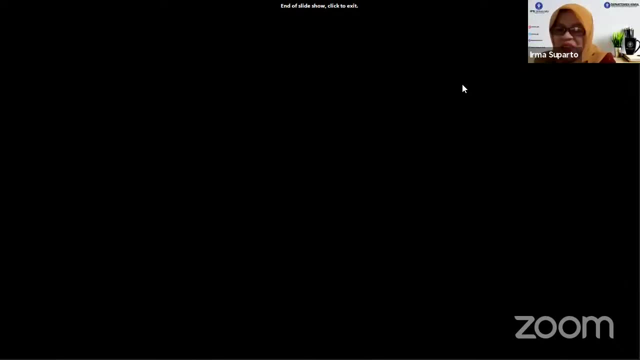 gonna have to get in line behind me, okay. so next is from dr budirisa: uh, i have. uh, what are important criteria need to be passed when you want to use an artificial tissue made of biomaterial? from animal tests to human body tests. so what's the process of going from animals to uh people? 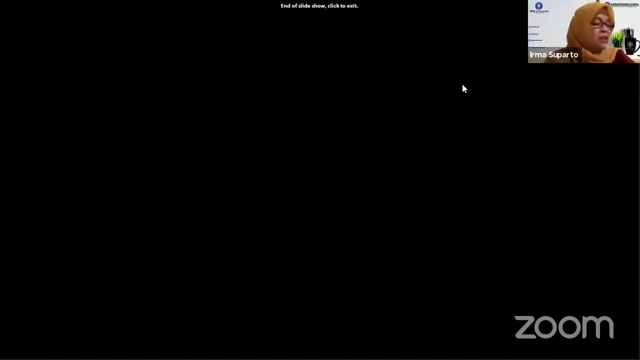 that's right, is the criteria. what is the most? well, um, to go to people, first and foremost. it can do no harm, that's number one. it must be safe, that's absolutely. you must have a biomaterial that is safe and doesn't cause more harm than it helps. in fact, it should not cause harm, so that's, that's a. 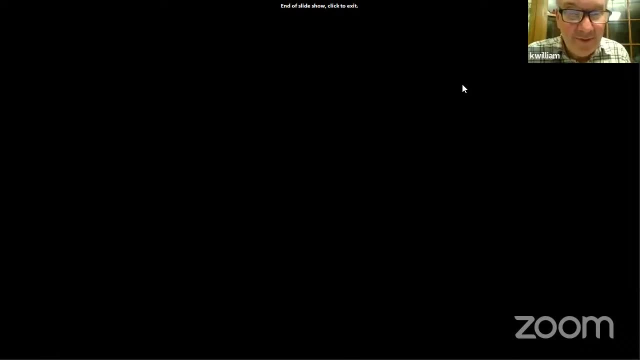 big one and most your last uh steps in getting approval to use it is a safety study. a lot of times those are just the safety studies that you're going to use, and you're going to use it because they have the immune system and and the physiology that's most uh like that of human. 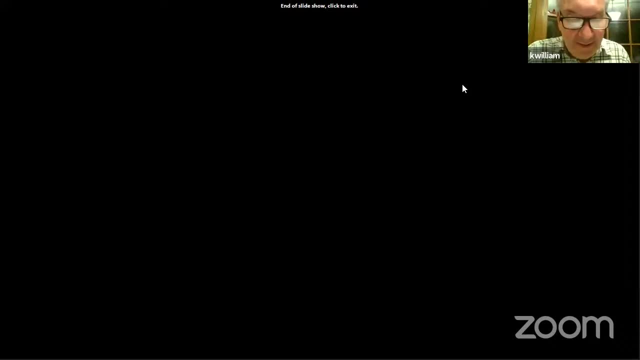 beings. um, it must be biomechanical that is not causing too much of immune response. it cannot cause. um, if there's cells in there, they cannot turn cancerous on you, and so it increases your risk of cancer. um, they cannot cause a new disease. um, right, you, you treat one and then you end up with something else. it can't do that. so to get it to, 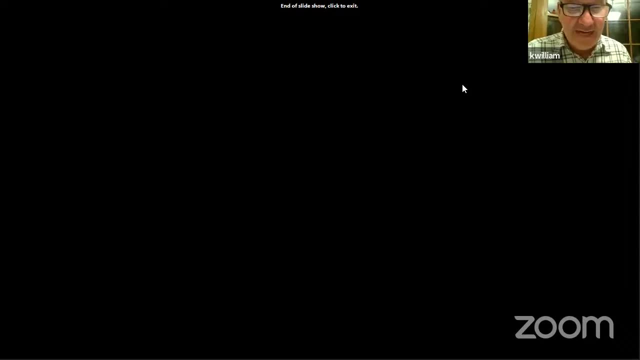 to get it to uh clinics, you got to do a series of safety studies. they might. it must be efficacious. in other words, it must work, gotta work, and, and but most mostly, you got to do a series of safety studies. make sure it's not causing it. thank you, proof, cody. please be patient. i think we have four. 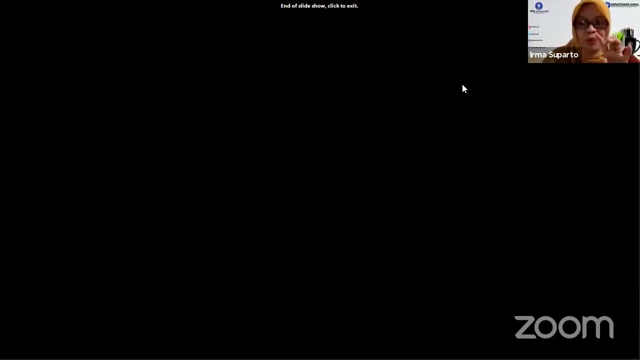 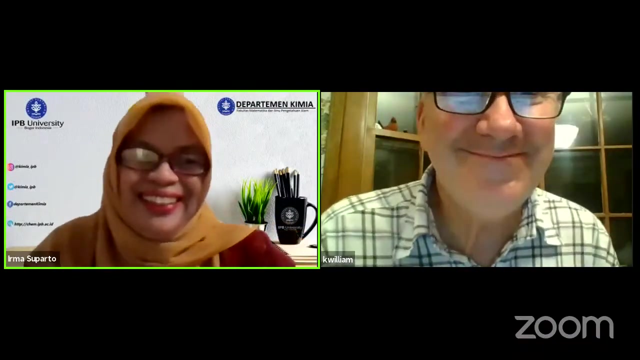 questions: uh, i will uh no more, or maybe we have that for one uh, but could you please uh stop share screen so we can see your uh everybody in one uh template. okay, do do what. uh stop share screen. stop share, stop share. yeah, because we have a black hole there. no, that's right. okay. so the next. 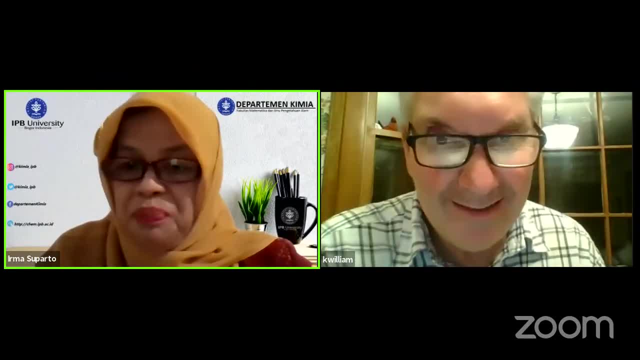 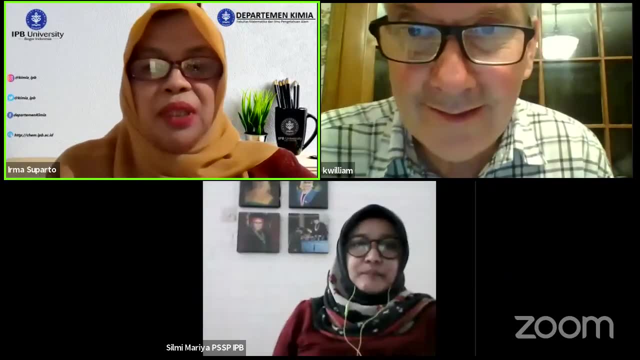 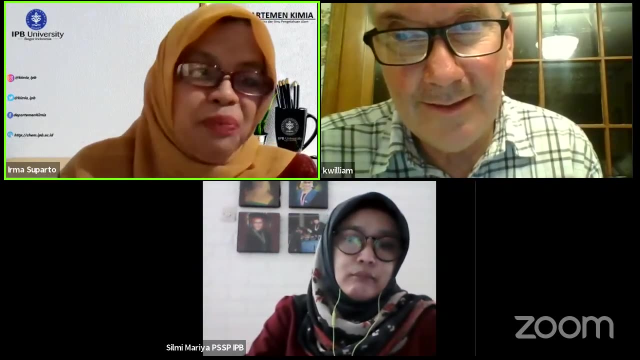 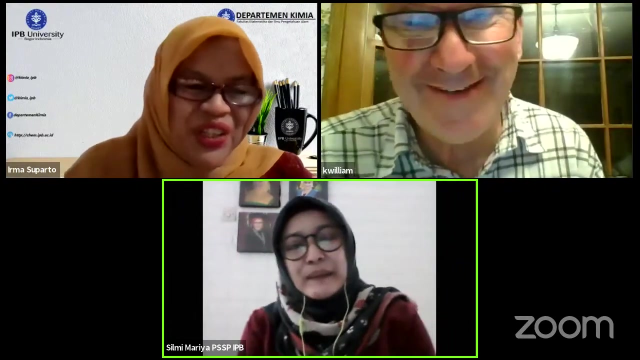 question is from your uh, favorite person, silmi maria: how to confirm the biomaterial is not rejected by the body before transplanted. should be done with a pilot study or just trust the manufacturer that produce it? never trust the manufacturer, never trust the manufacturer. no, you got to do the studies yourself, silmi um you, you've got to do. 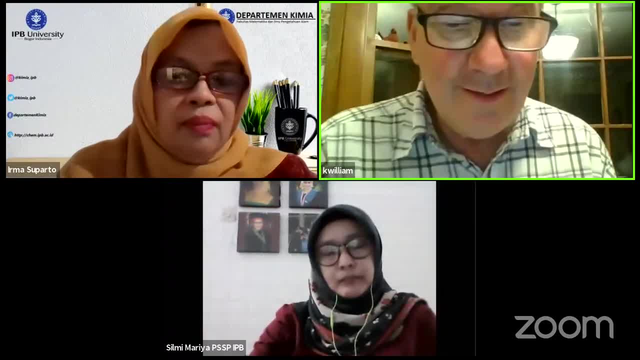 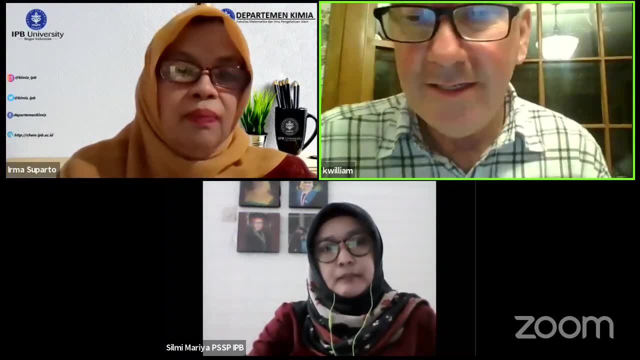 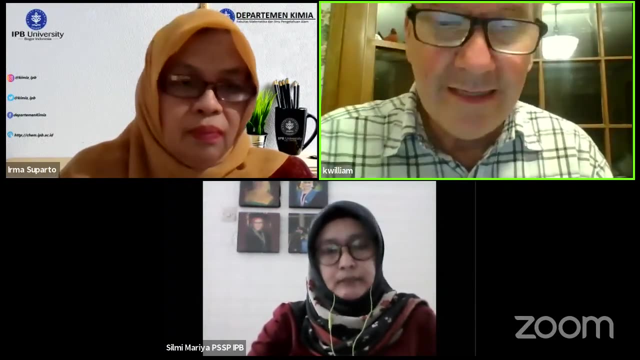 is there any peripheral uh problems with rejection? in other words, you can do some peripheral uh white blood cell uh evaluations to see if you are stimulating uh, various uh types of macrophages or t cells. you got to look around. a lot of people just look at their implant and say: oh, everything looks fine. 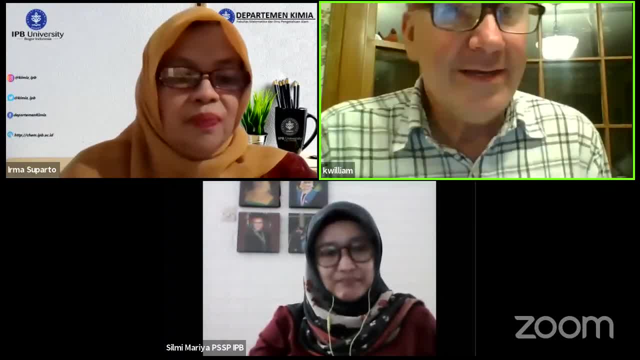 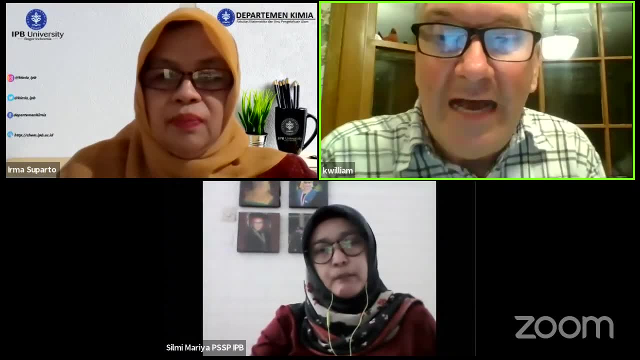 you got to look around there. you put the implant too. you got to see what the um regional lymph nodes are doing, what the spleen is doing, what the lymph nodes are doing, what the lymph nodes are doing, um, you, you've got to do your own and and i know you can do those there. but it's very 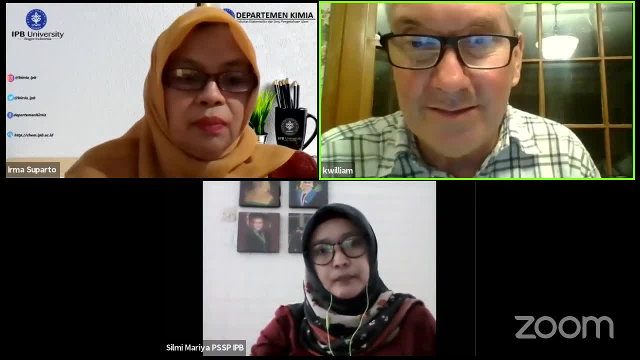 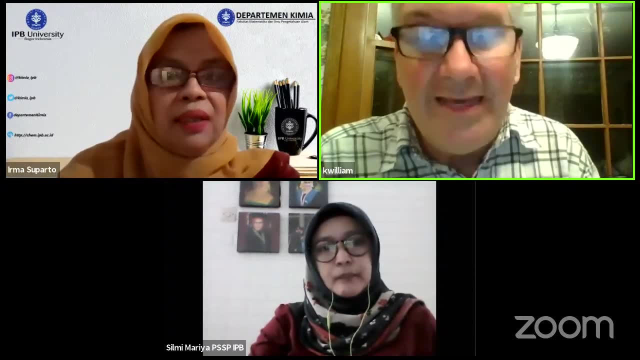 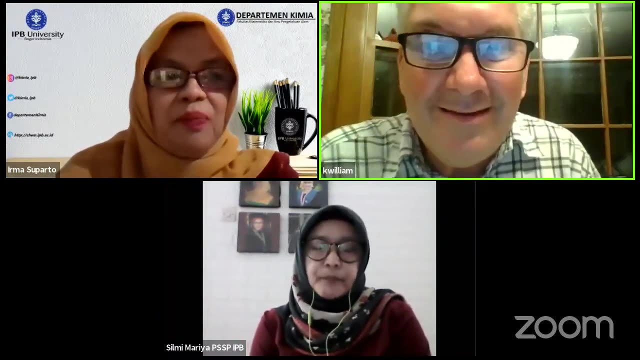 important also to look for activated uh white blood cells in various forms, where they'd be macrophages, t cells, sites, whatever. um, yeah, you got to do your own, so they may make you do more. they may make you do more, yeah, but you got to be around. okay, thank you, thank you okay. so okay, i hope. 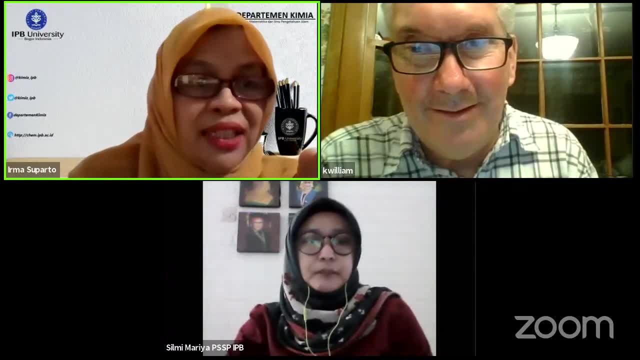 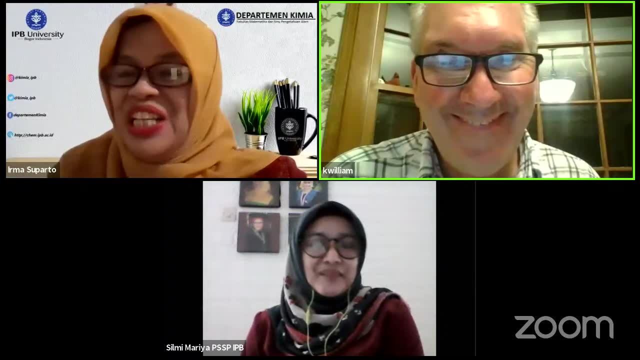 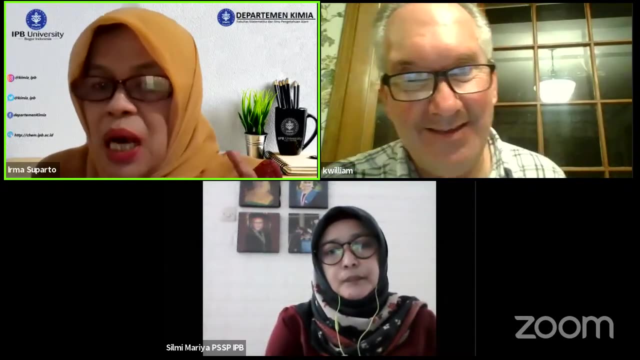 i can see your window is starting to get darker because it's opening, but you stay up, okay, don't go to sleep. i'm not going to sleep, okay, now it's from rifan norfala. hi professor, uh would like to ask about properties of biomaterial and specification for template of biomaterial. 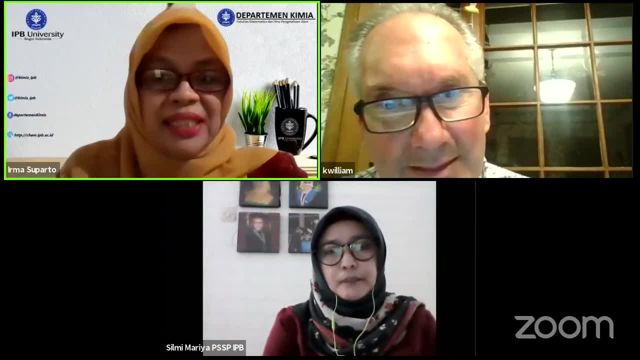 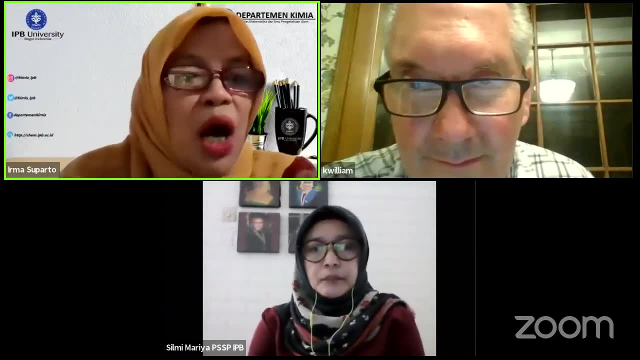 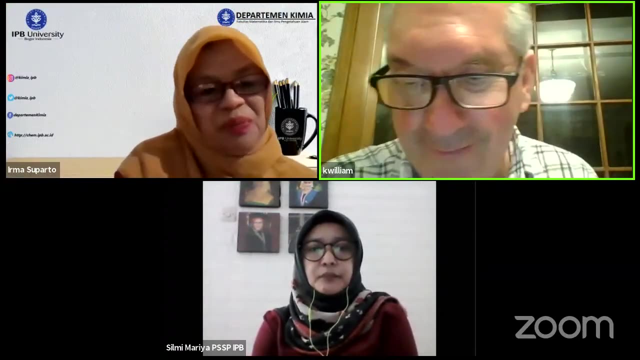 how do we determine the right level of elasticity? and, second, how to prepare, uh, the material according to the rheological characteristic. oh, that's, yeah, that's why you always have um in any study design. you have normal controls. because the normal controls- and remember what i always- 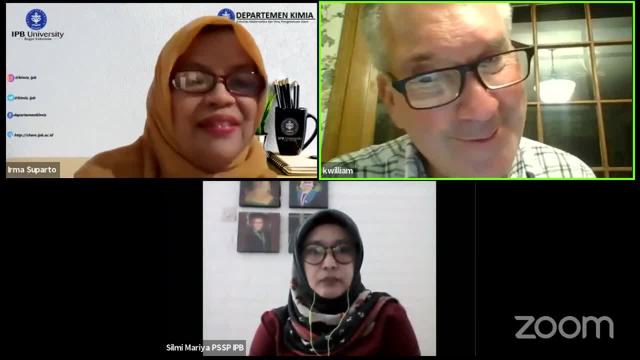 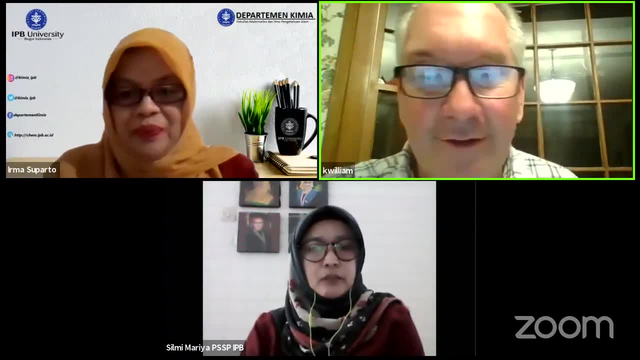 used to tell you your most important group in any study is your control group, and so you have to know what the normal uh is. let's say you're looking at a bioengineered artery. well, you got to get that artery- normal arteries- out, and you got to do some. 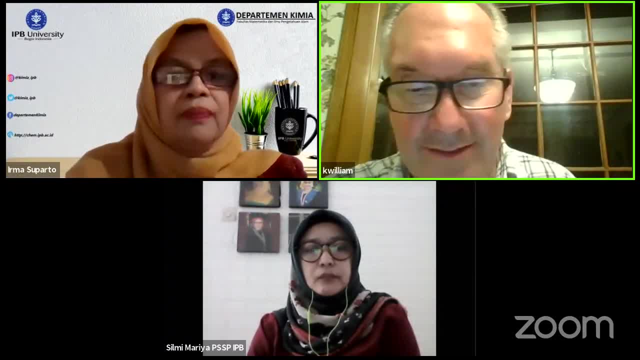 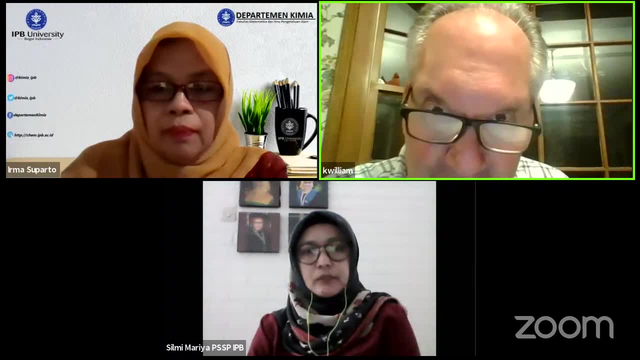 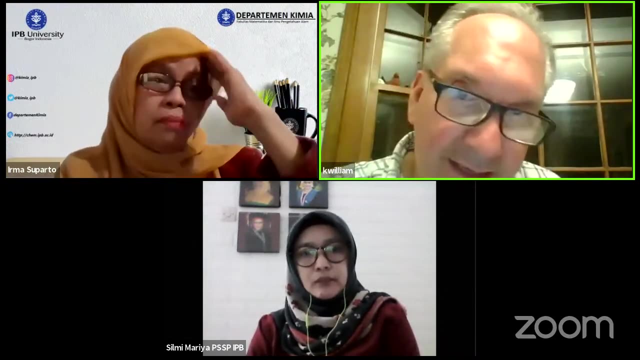 biomechanical testing on it to know what the stress strain uh curves look like. and you, you've got to do that and then test that against your, your implant. and your implant should try to do its best to mimic or recapitulate those biomechanical properties, the strength and the 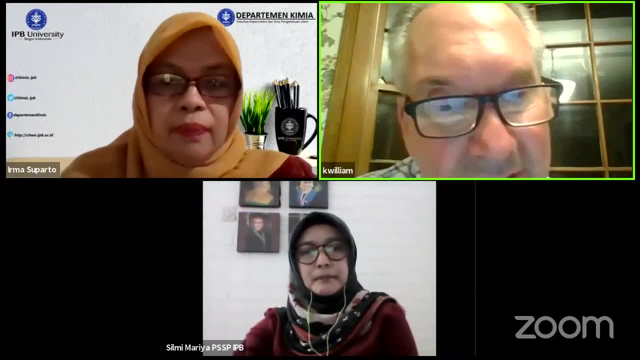 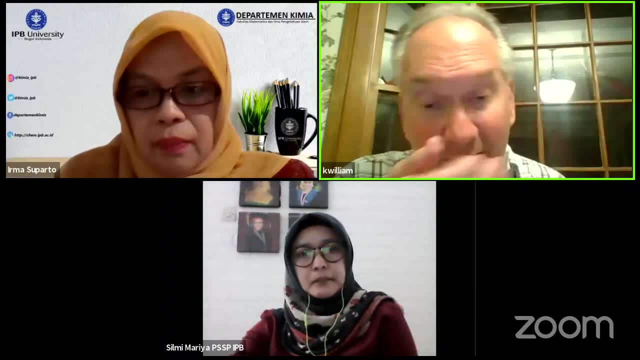 elasticity. so you got to do some, some controls. a lot of that is actually in the literature, um, if you go searching for it, a lot of times people have already done by doing biomechanical tests is not new, um, and so a lot of times you can. 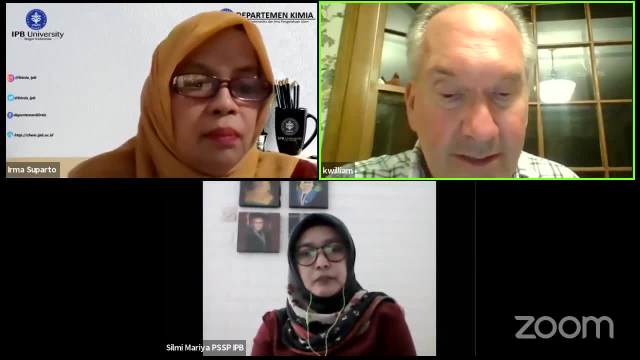 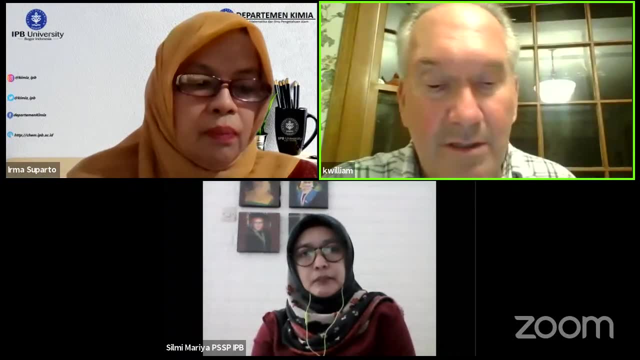 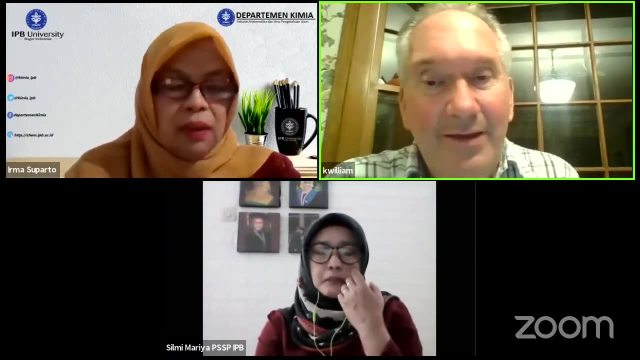 find that stuff. um, you still got to do a control study because you're going to have your own ways of measuring uh, biomechanical properties and it has to be against your own, um, your own controls. but it'll give you an idea where you can start right it. it has to have a certain strain modulus. 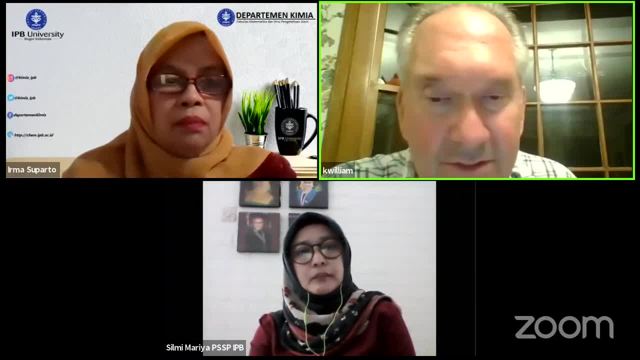 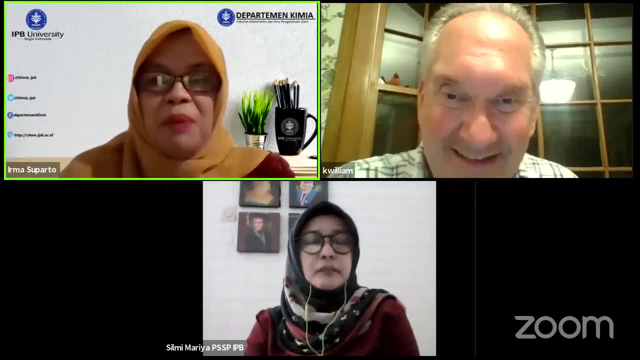 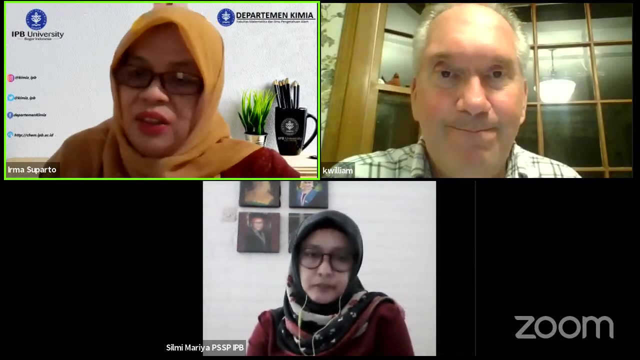 that it will. it will give you a place to start so you don't have to go search for it all over the place. look at the literature control group. yes, i always remember that before you start study, read, read a lot of journals and have a control. yeah, okay now, uh, um, one question from 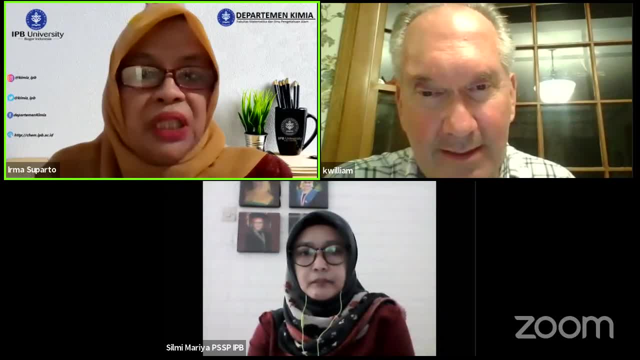 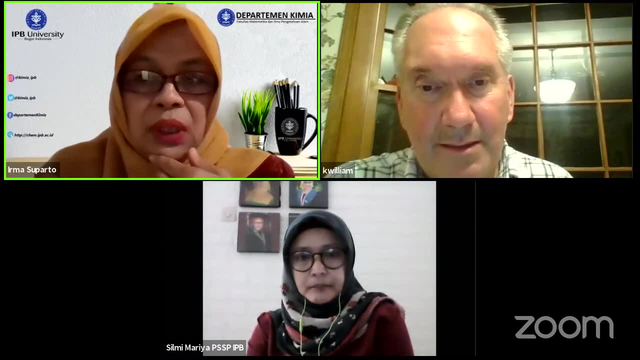 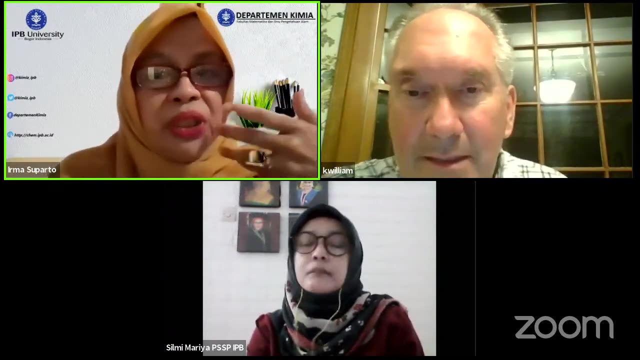 dr nofian about the injectable dermal filler for aesthetic purpose, right, especially for the face, because it's a trend now. what do you think the long-term effect? uh after uh, uh, external exposure like uv and so on, like that- do you think there will be problems? 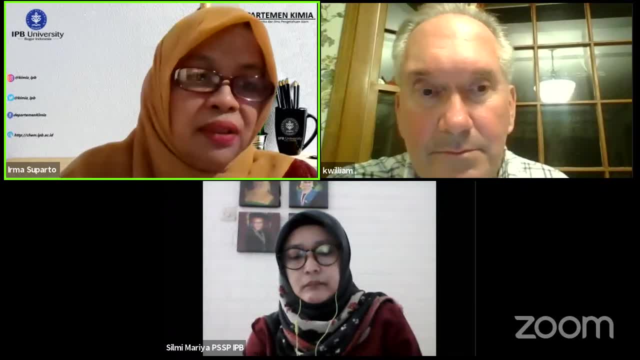 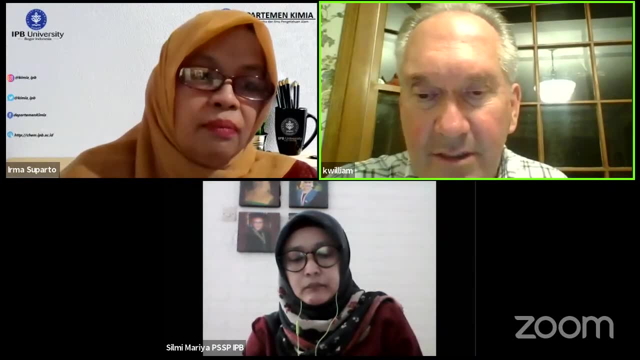 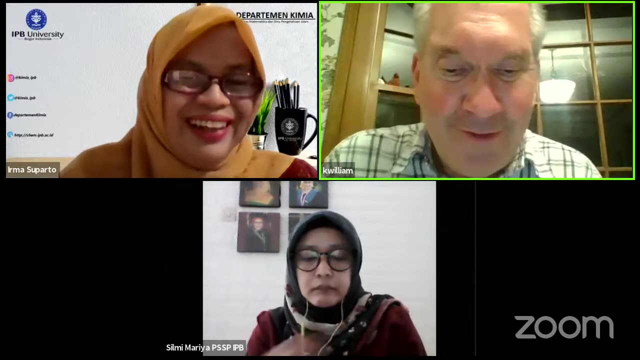 of those injectable, uh, dermal filler i i don't think we'll really know, irma, until these people have had those dermal fillers for years. i don't know what happens to them and you know people are getting them at a younger and younger age. i don't know why they needed that when they're young. 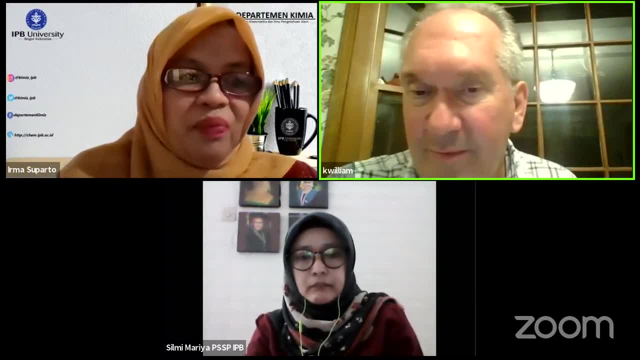 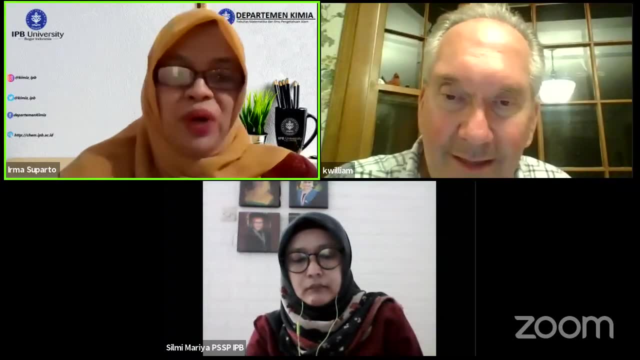 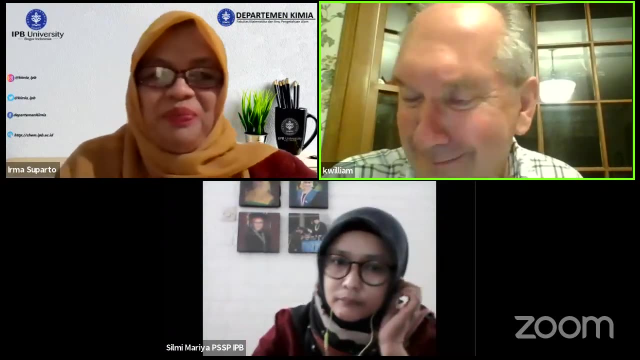 um, but they don't. there are people that are doing it. we won't really know. short term there doesn't seem to be that much problem, but we won't know. we're 10, 20 years out. well, actually, we don't need it right. growing old, uh, elegant, no, no, no, no, i deserve every wrinkle. i. 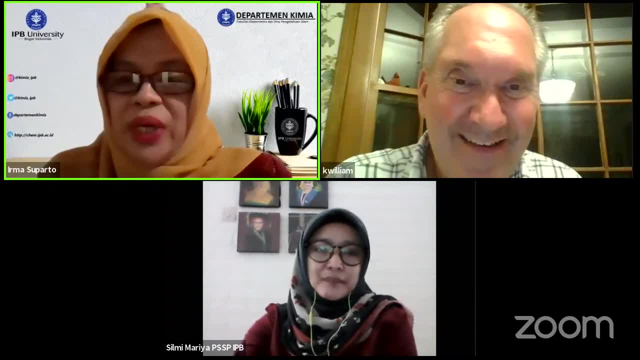 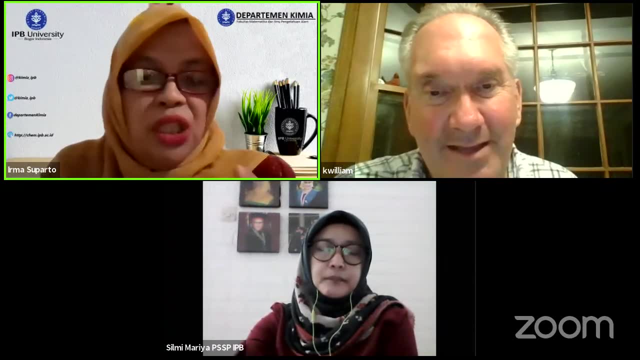 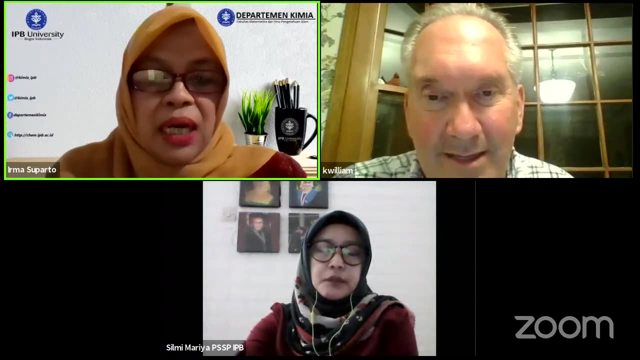 have. yes, okay, i, we don't have one last question, but it's in indonesian, but i will try to translate from ramdan hidayat: so, uh, you mentioned about perturbation physiological environment, right? so we program the program, uh, re-expression of the gene, right? and then, uh, what do you think about this? according, 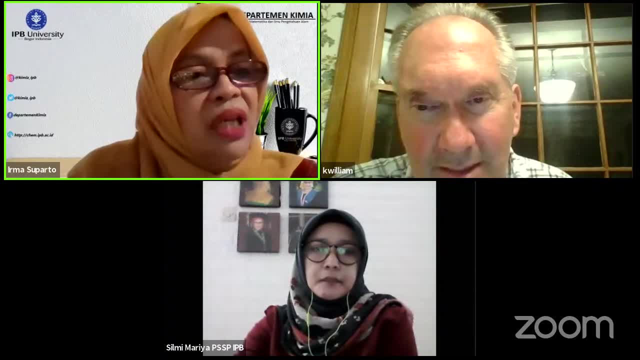 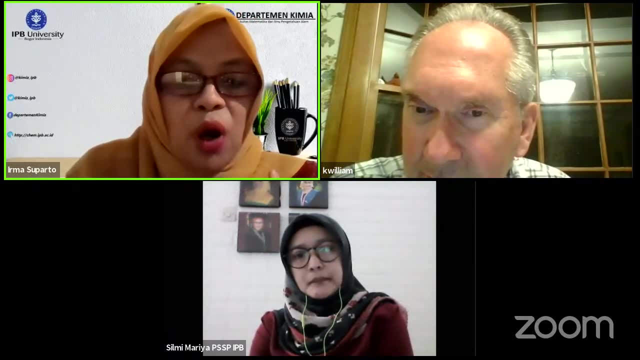 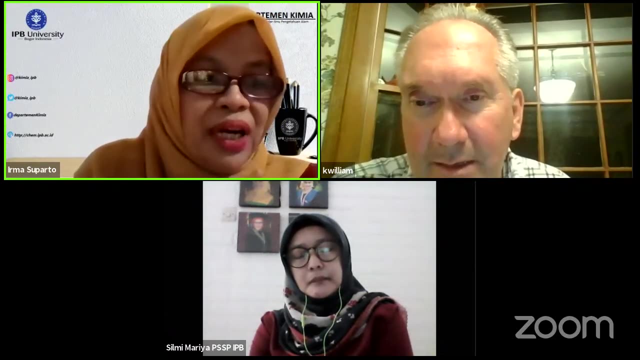 to aesthetic. also, this is about question of dna salmon. have you heard of that? there's so a trend about dna salmon that it can uh from uh, extraction dna sperm of salmon and then they inject it. have you heard of that? so dna from salmon? yes, uh from the sperm. 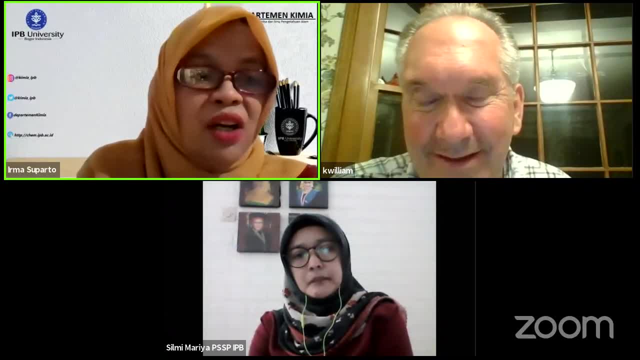 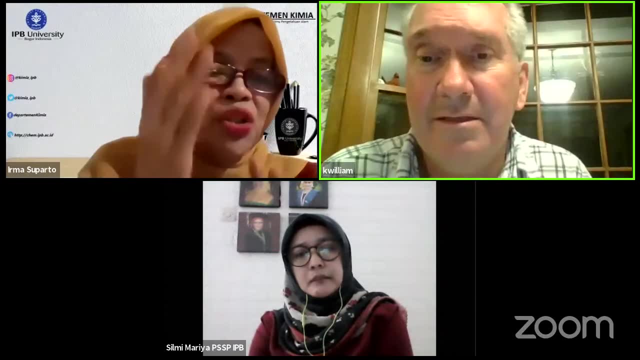 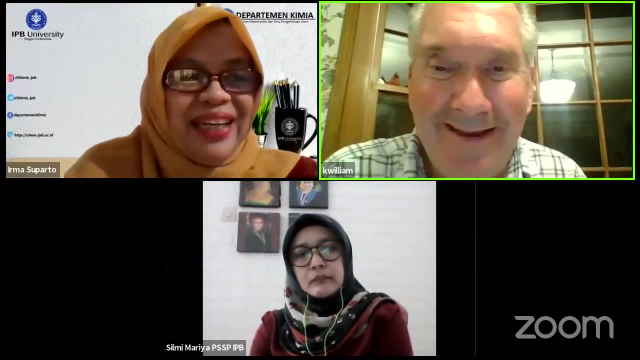 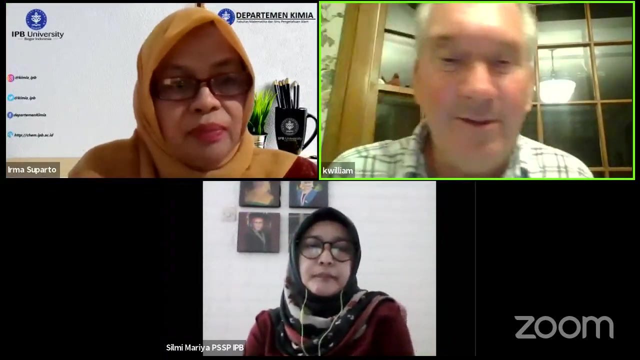 they said is uh to improve the skin also. so it's really a big business for this cosmetic really. so you should be one uh making uh innovation such as i. i can get salmon sperm and make millions of dollars. yes, what do you have you heard of that? uh, prof. cody, i've only read a little. 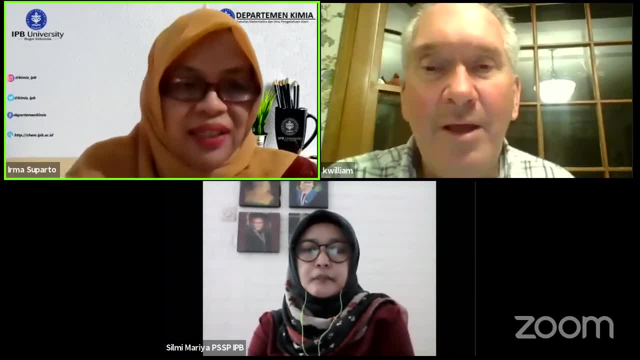 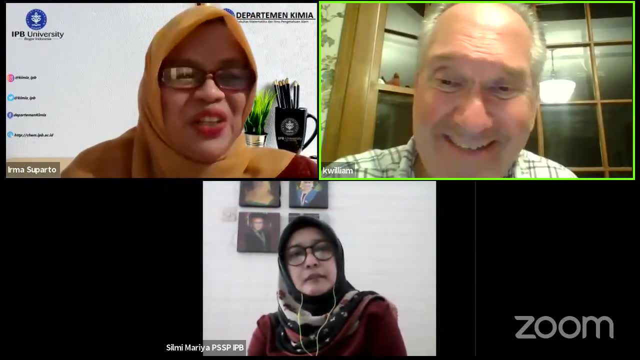 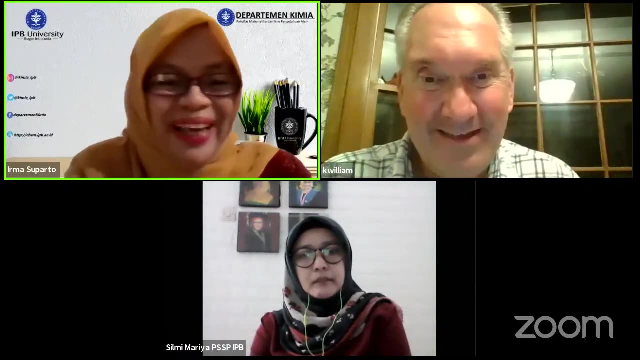 bit about it here. i'm not very conversant on it. i know people are injecting all kinds of stuff into them now trying to stay young. um, i don't know about salmon sperm, that much, okay, but uh, i'm sorry. uh, we need to read more about that. okay, uh, one more. what is it? uh? oh, thank you so much. 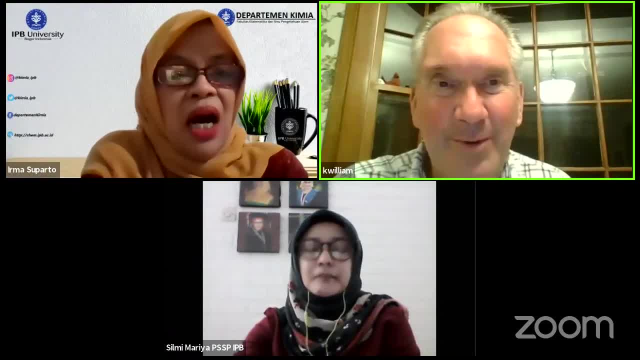 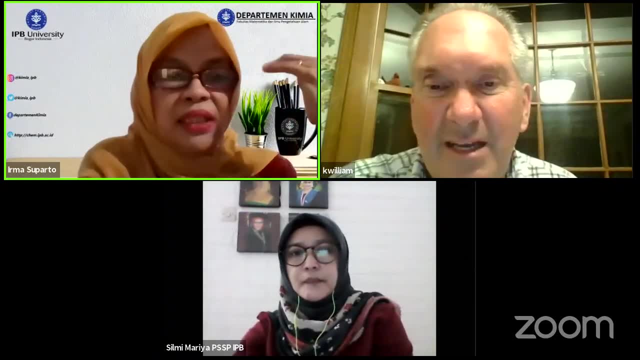 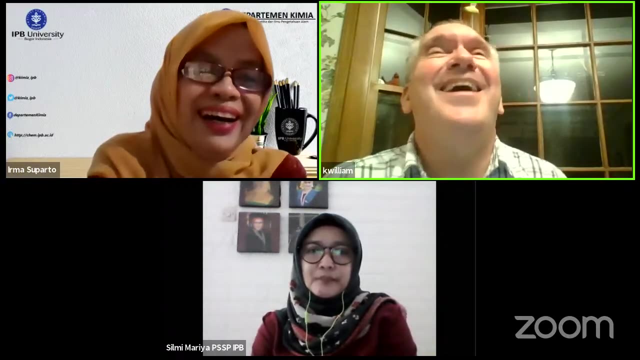 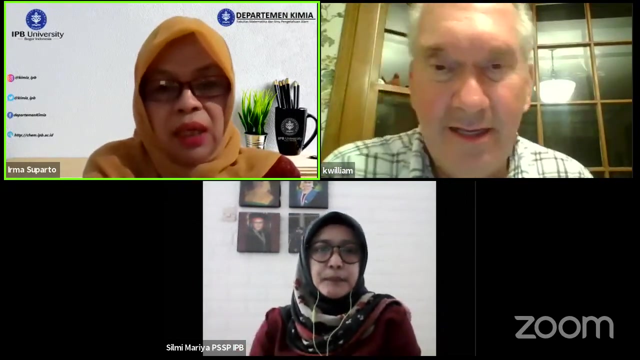 from everybody. oh well, you're very welcome. so many things in our head and we always- you know, you know us- we always want to learn and learn and learn, especially from such a person like you, but we do not want to keep you up, so, uh, it has been such a great uh talk and, uh, i think this is a really good strategy to have you. 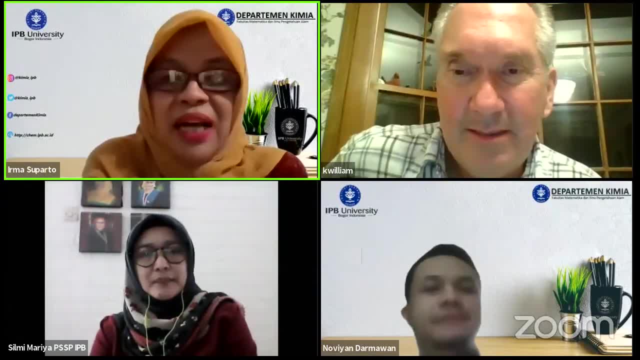 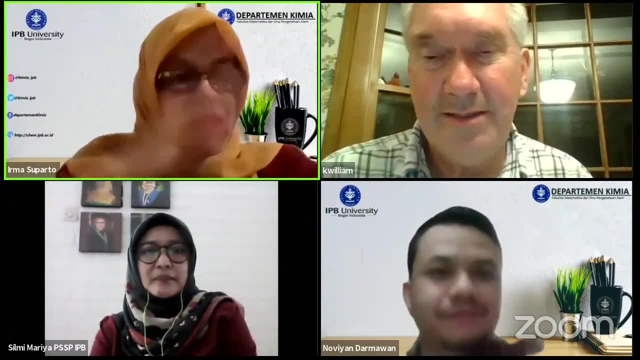 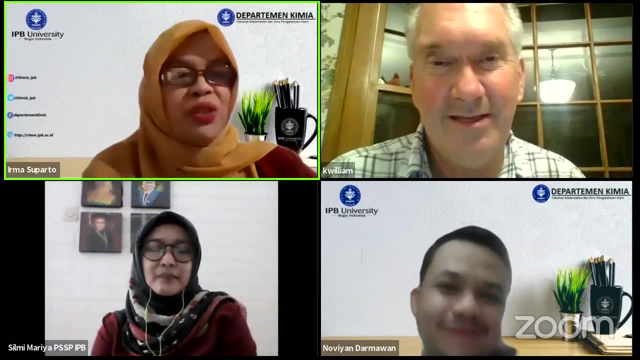 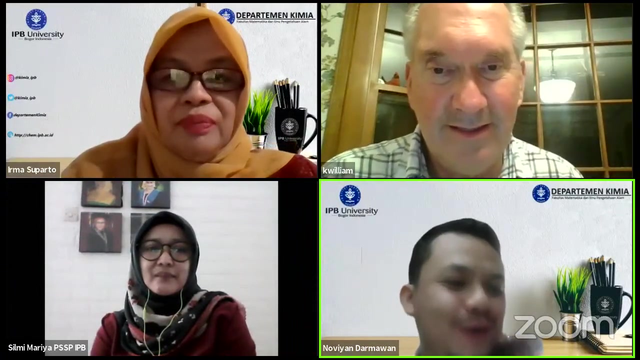 in the last uh session of our semester. right, uh, but no fiat, yeah, because uh so the student already had some uh open, uh open uh perspective about the biometric. yeah, that's right, you kind of sum it up, sum it up suggesting a student to continue the study and research. uh, for the cosmetic purposes, because 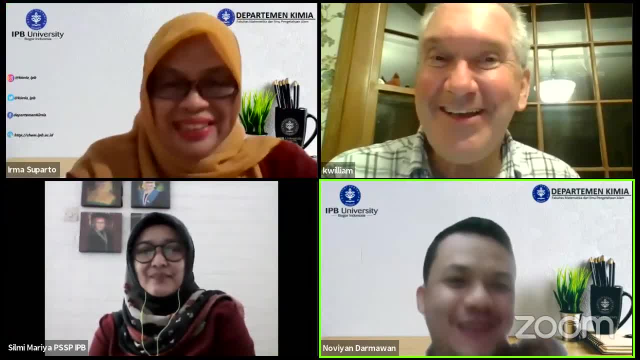 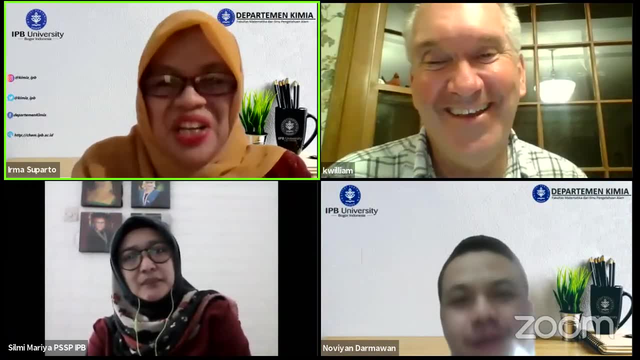 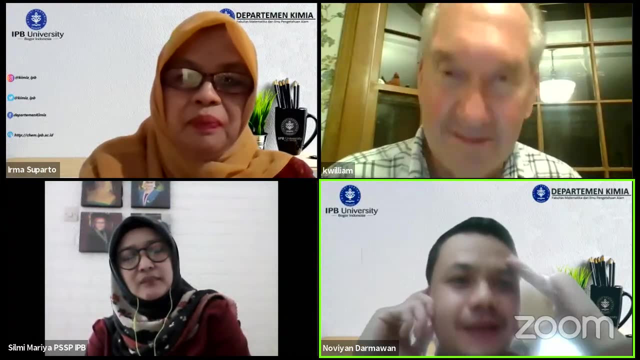 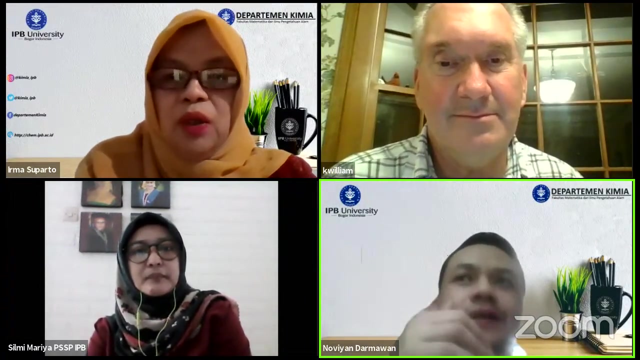 again, again, you're gonna have to get in front of the line of me. but yes, i mean here uh in indonesia a lot of like a korean product uh, cosmetic uh that they really uh forward uh how to say advance in the cosmetic uh for the application of biomaterial, for the 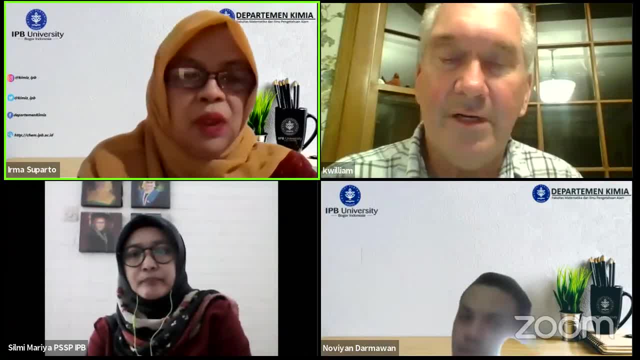 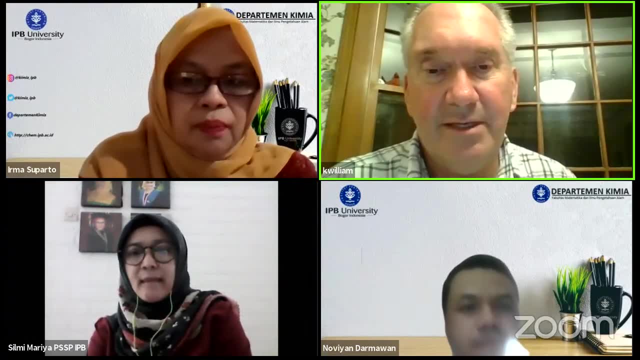 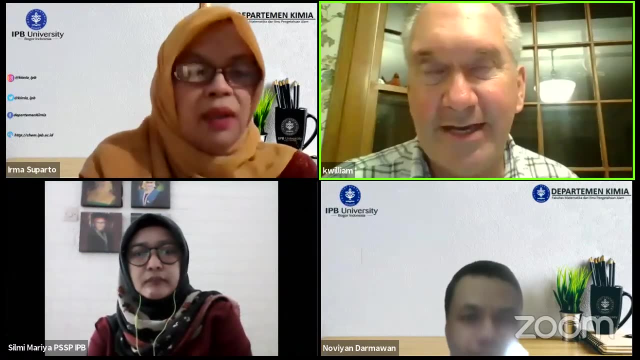 cosmetic, very progressive, right, right. yeah, well, i know, i know it's big business and and and stuff. just uh, you know it's, but it's like giving a drug: you got to know exactly what you're giving, you got to know the dose that you're giving it, or you're going to get different results and you and it's got to be a. 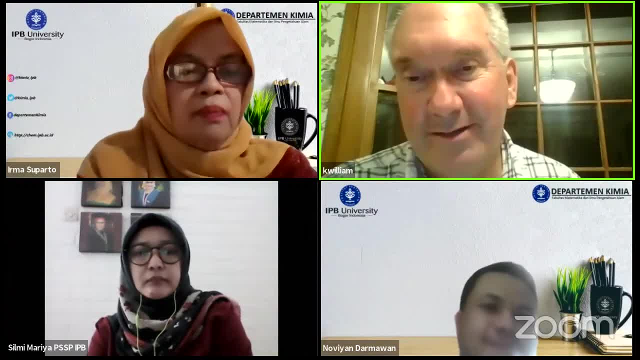 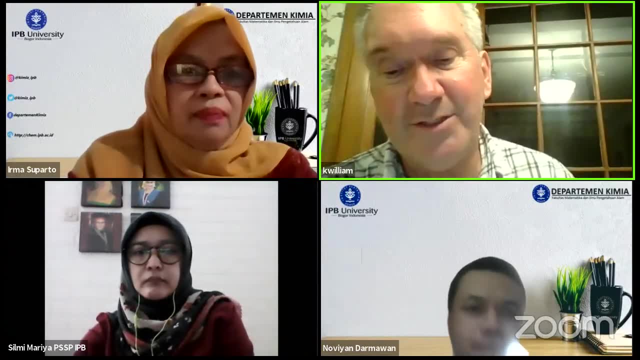 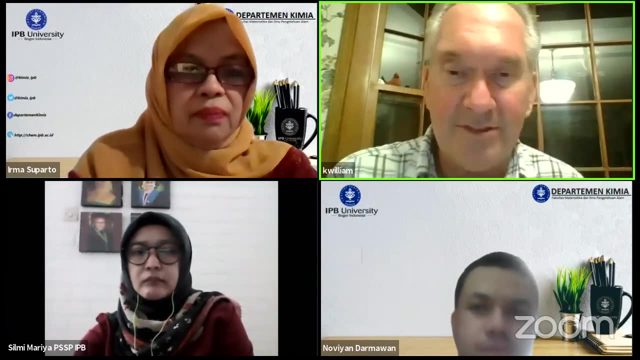 consistent, consistent product or it's. you're going to get different response. some people get great responses, some people vote. it's like taking platelet-rich plasma or you get some cells big in veterinary medicine. now it's just getting some cells from animals and shooting it in their knees. um, it'll work sometimes, but it's not almost enough and it's not worth it just because you're receiving drugs, so you've got to keep doing that. there's a lot of things that you have to do, and it's not that you know you're not doing the right thing if you're not able to keep up with the medication. 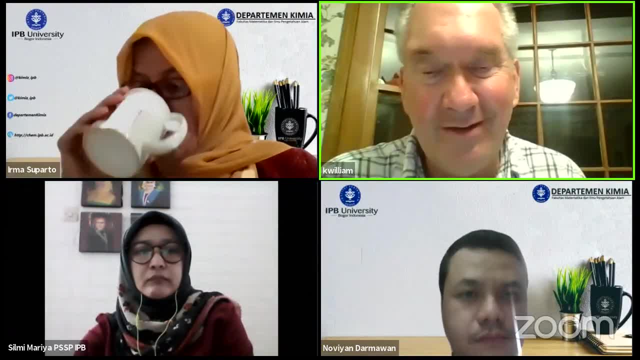 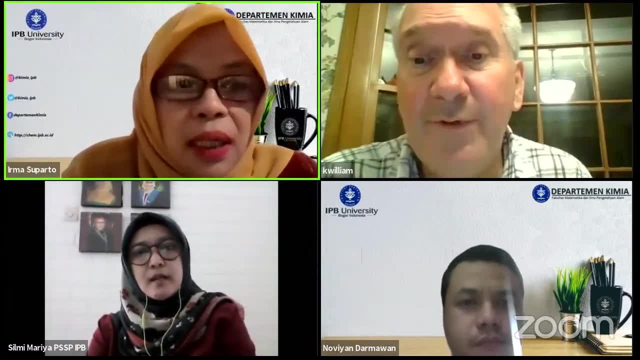 Sometimes it won't work. others because it depends what kind of cells and unless you know it and you've standardized it, you're going to get varying results. I did check with David Williams. if you want to make PDF out of those slides, you're welcome. 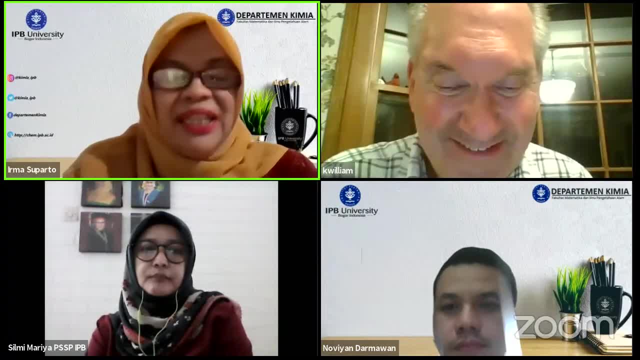 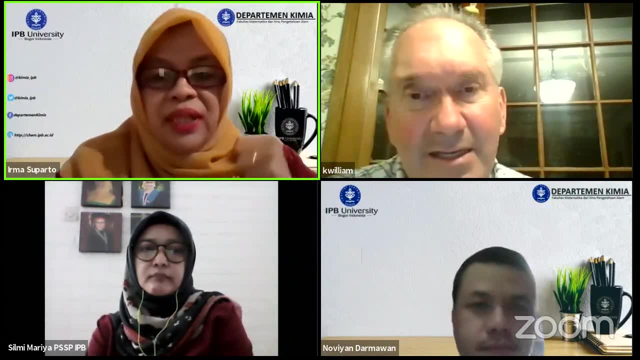 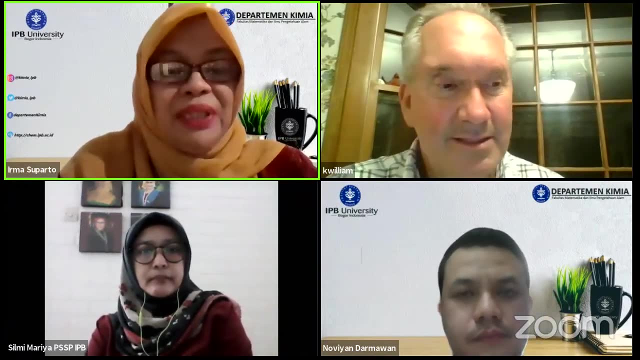 I will and I will share to this the code here. That was a very good closing statement that we have to make sure about safety, So that I will not make it add another statement. but, most important, we would like to say thank. 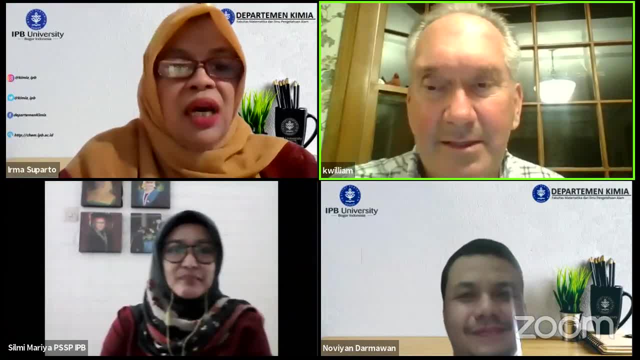 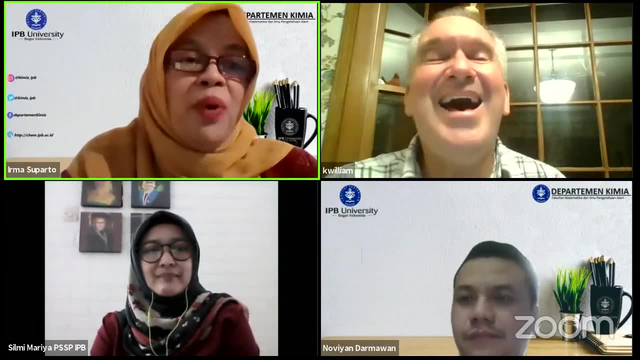 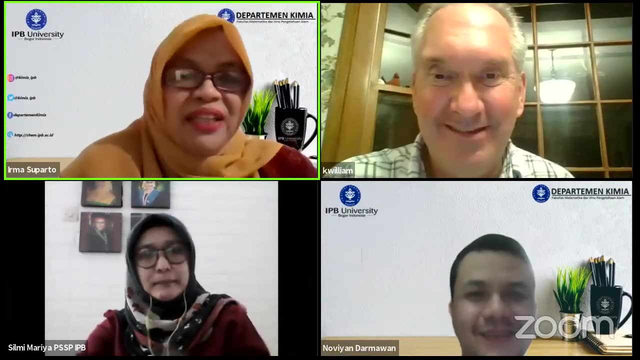 you so much for sharing. It looks like that you will be more. we will chase you more. asking of your- Or maybe sometime I can come over there and stay a while and, like teach a semester or something. Oh, yes, That will be great. 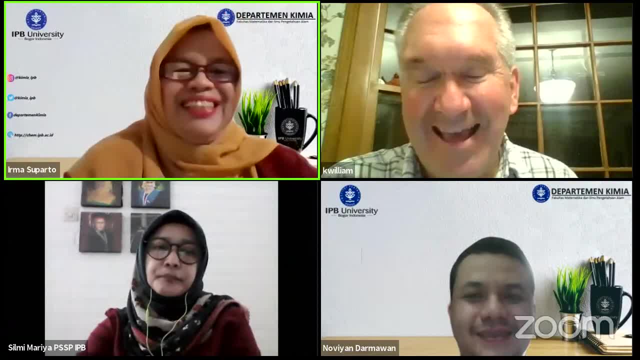 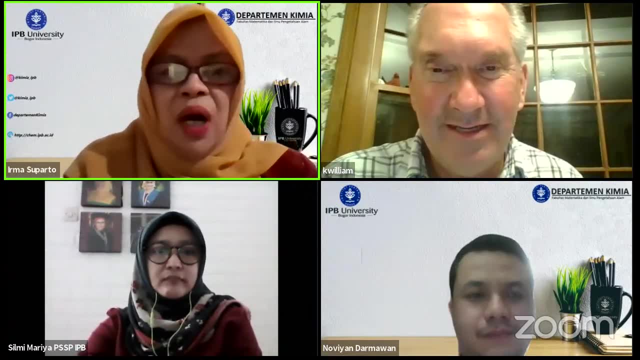 And then see what happens, See what's really going on in real life. right, Yeah, exactly. Thank you so much, Prof Cohn. Oh, you're very welcome, Irma, Great to see you. Thank you so much for the audience, for the head of department, Paya Nofian, and also. 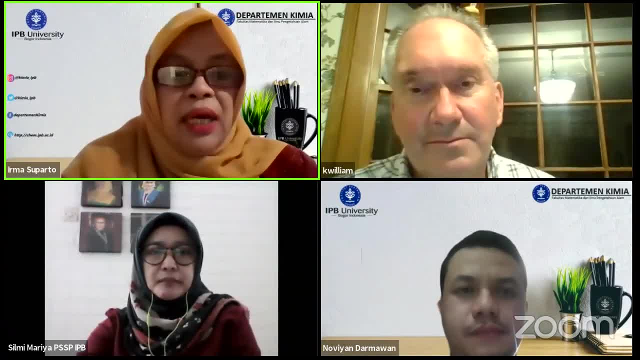 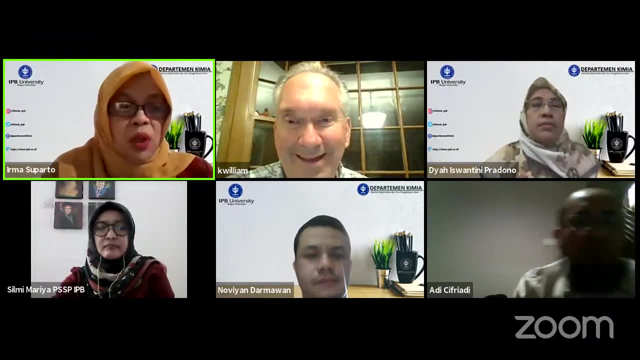 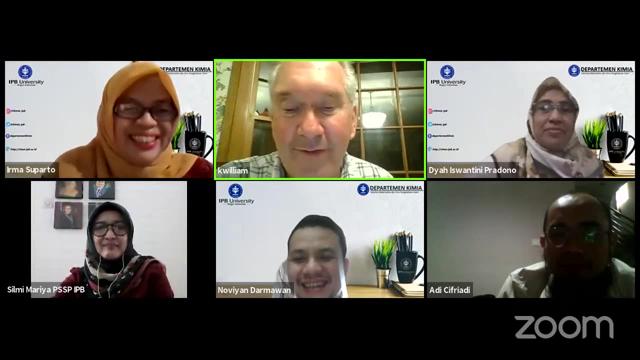 all the lecturers that attended this lecture. It has been very insightful and we are so happy and we cannot give you a soto ayam or satay ayam, but at least you can dream about it. So- I can. And we had fruit tonight for dinner and I put in mango. 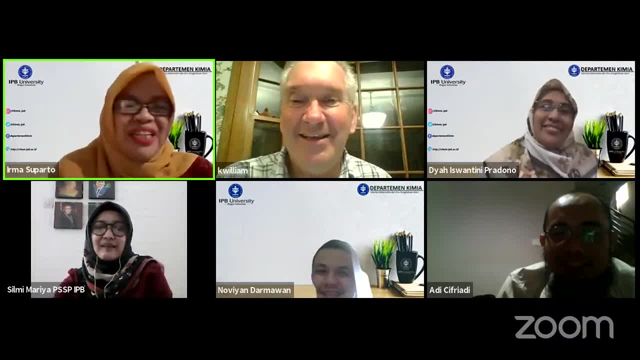 So- Oh, that's nice. At least you have a touch of Indonesia there, right, A touch of Indonesia. We can get the they're kind of yellow called champagne mangoes, And we can get- And so I had mango tonight anyway. 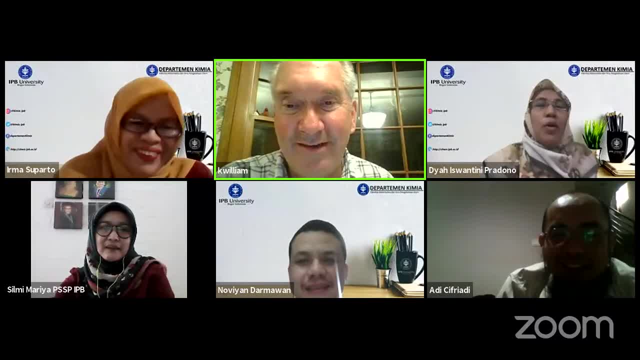 No durian, No durian. Okay, Next time we'll have a. it's a rain check. We'll check again, Okay. Thank you so much, Prof Kirby. Oh, you're very welcome, Irma. Thank you. 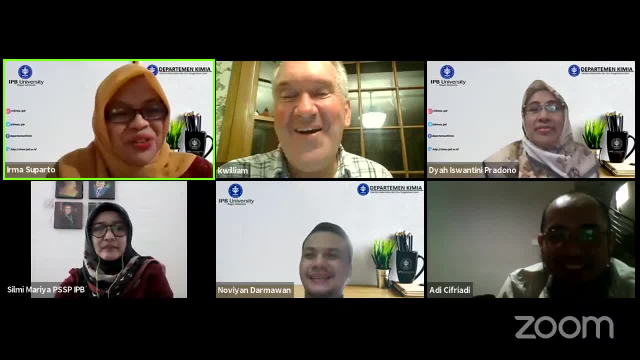 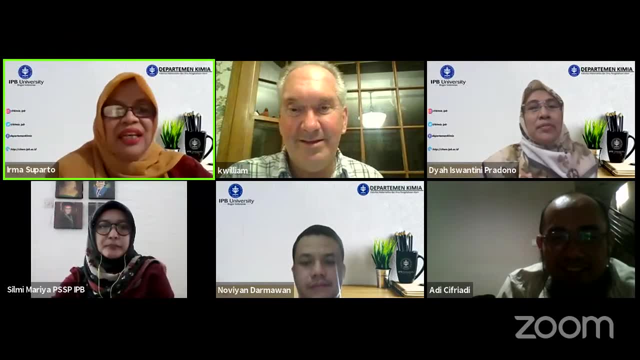 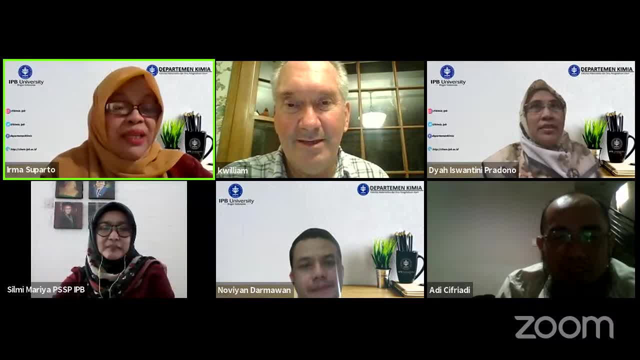 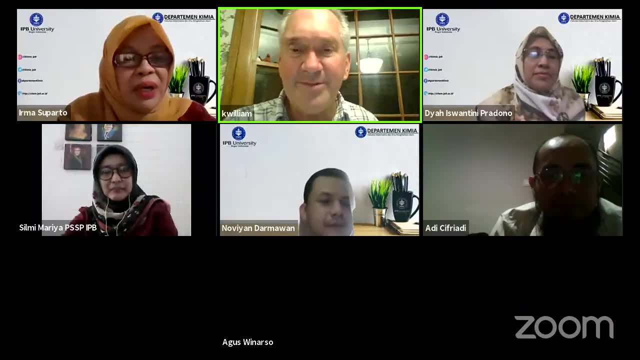 Alhamdulillah is praise to God that we finished all this, And so we hope to see you again soon. and may the pandemic get over soon- I hope so- When we get together again. Thank you- I hope so. Thank you everybody. 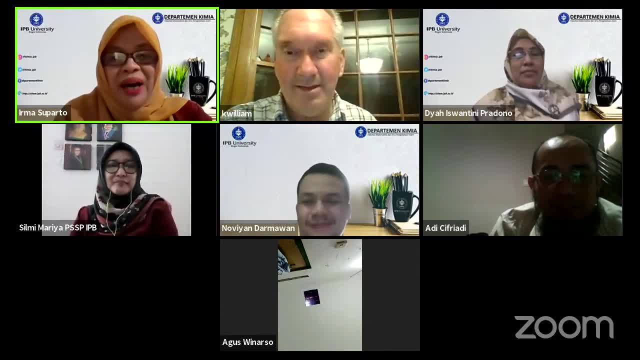 Thank you, Have a nice day and goodbye. With this I will close the lecture. Thank you, Okay. Waalaikumsalam, Waalaikumsalam, Waalaikumsalam, Waalaikumsalam, Waalaikumsalam.